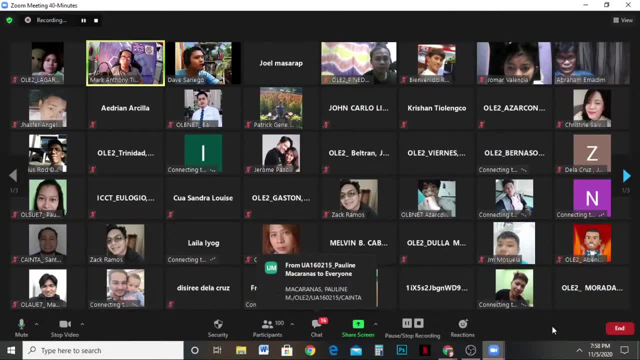 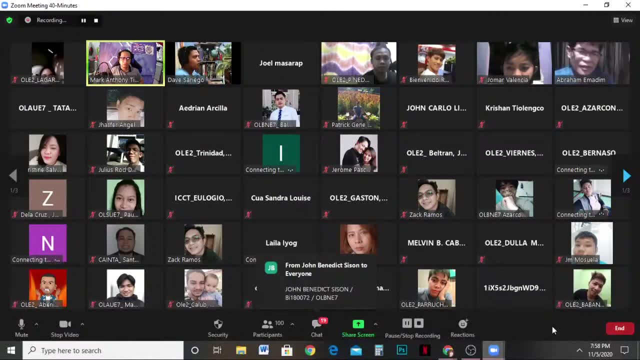 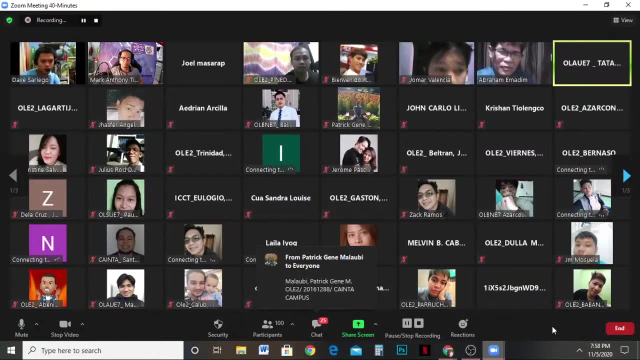 Midterm, Then after 1 week, 1st week. That's finals, sir. 1st week of December. Attendance already 4. I saw 4. There's a down payment. Down payment in December, sir, Down payment in December. Hmm, Let's see attendance first Those who didn't. 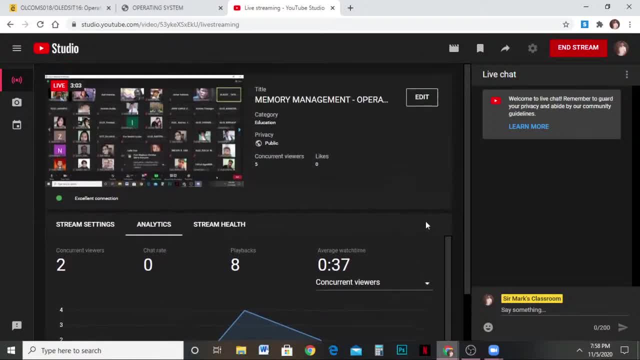 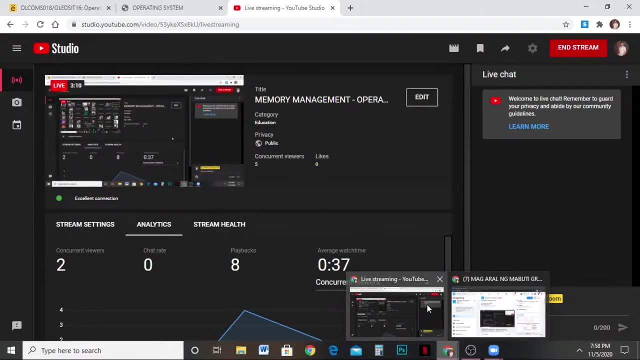 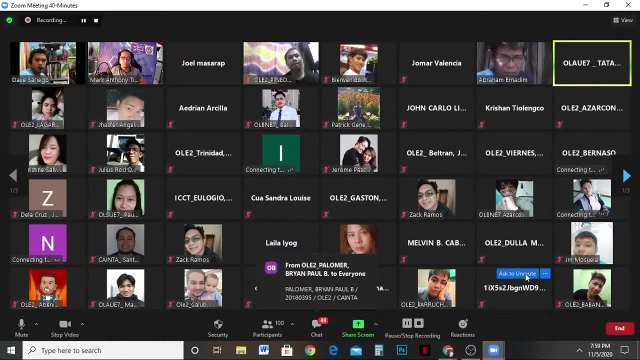 enter. You should be live. Just two. Are we too many? Not yet, Not yet. We don't have time. Let's see Who's watching Before we start the lesson. Let's do clarification first, Anything that you want. to clarify Nothing, We don't have any problem. 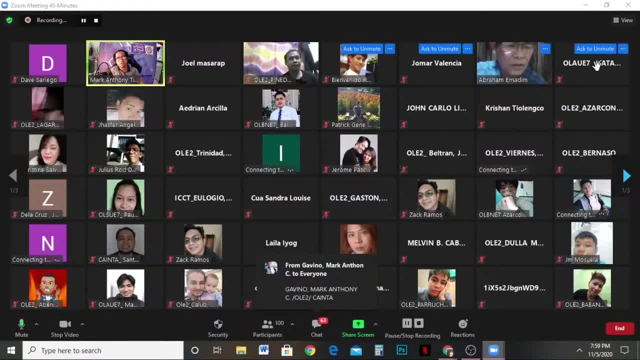 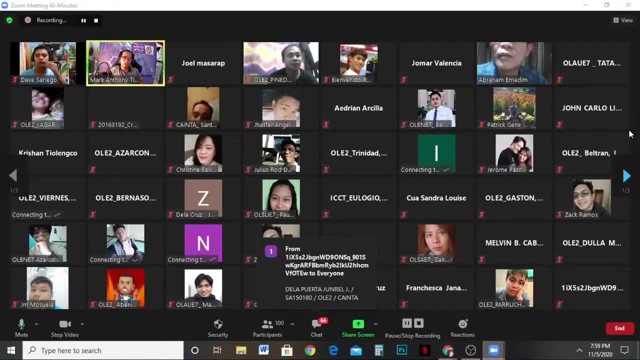 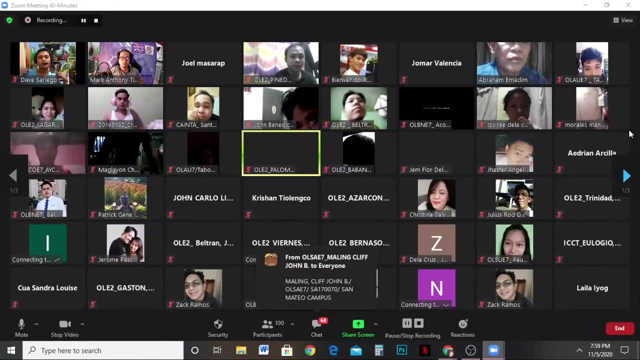 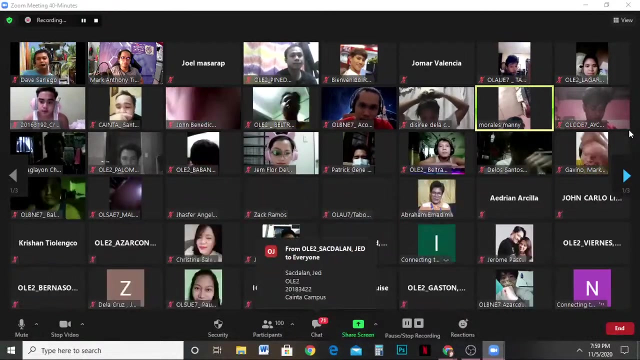 With the subject: Open the camera. You're unfair. Open your camera, Open your camera. Open your camera so we can all see each other. I'm still eating, sir. I can't open the camera. I can open the camera so we can all see each other, so we can all be happy. 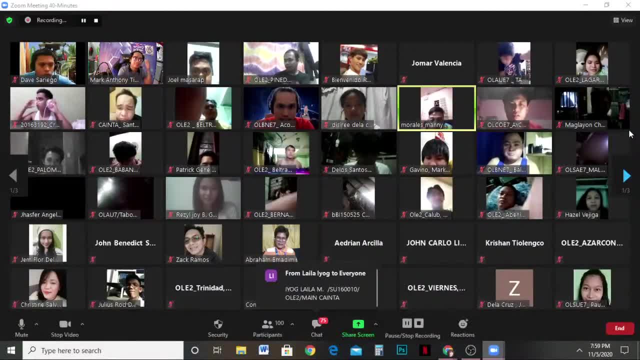 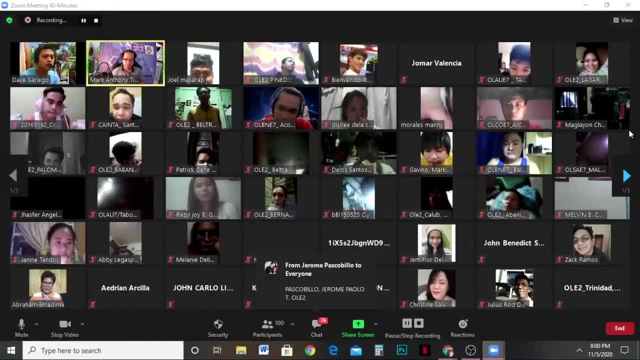 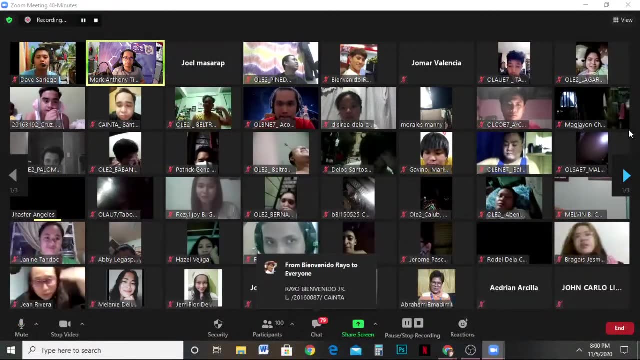 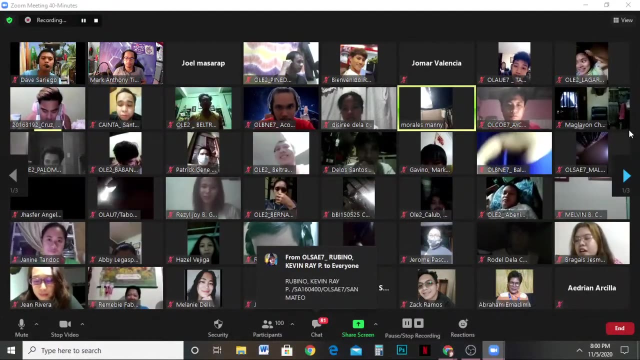 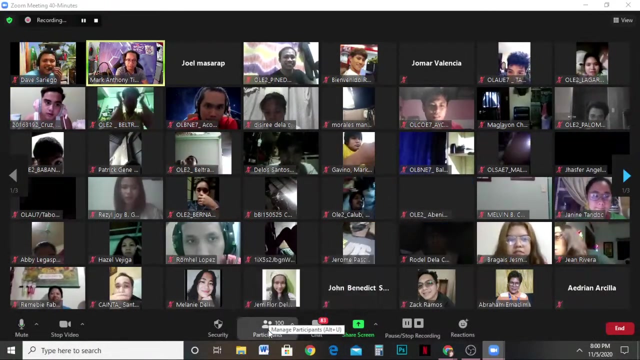 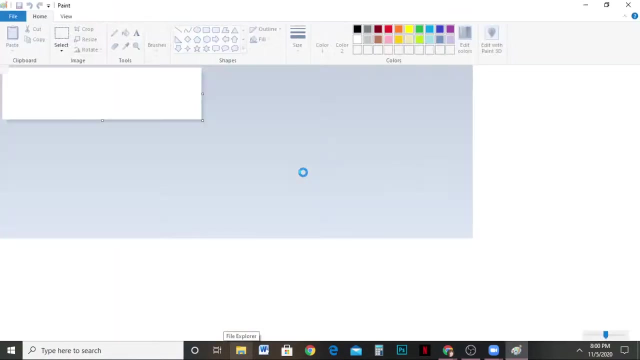 let's go, sir. ok, let's go, sir. ok, we will clarify all of them. this is fast, this is really fast. let's go, sir, sir, sir, let's start with the questions. ok, screen 100 participants. sir, sir, is our exam 2? ok, your exam? 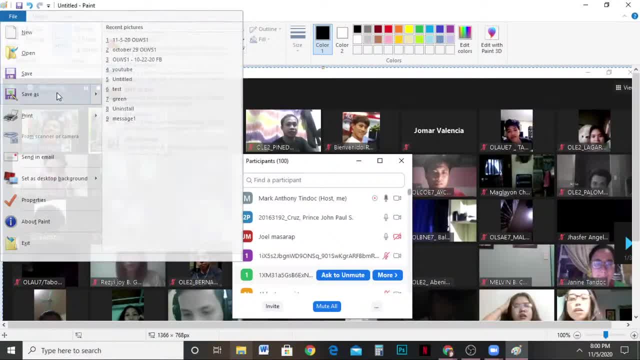 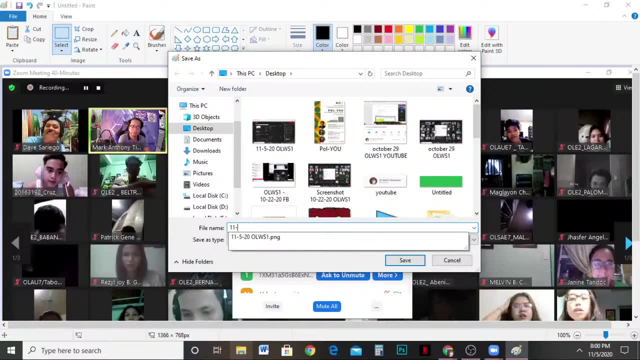 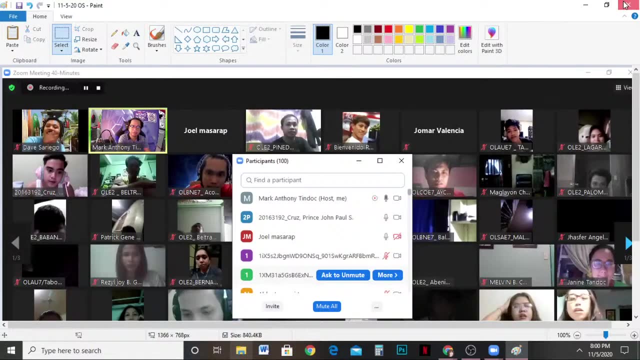 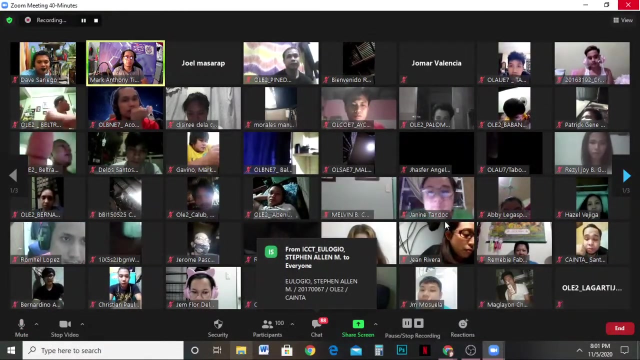 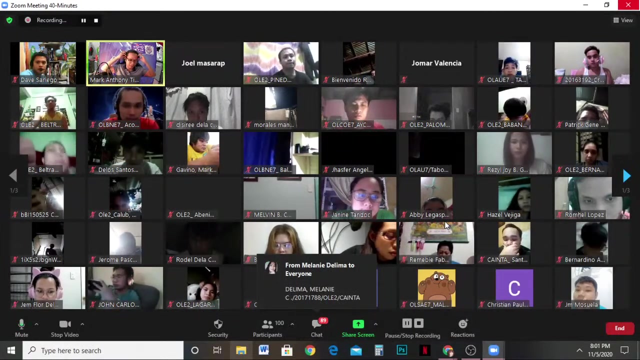 I haven't fixed it yet, but it's ok, it's up to me. thank you, sir. right now, 11, 5, 20 OS. ok, the exam is over. all of us are ok. my only problem is the new enrolment I extended. I extended your activities for life. 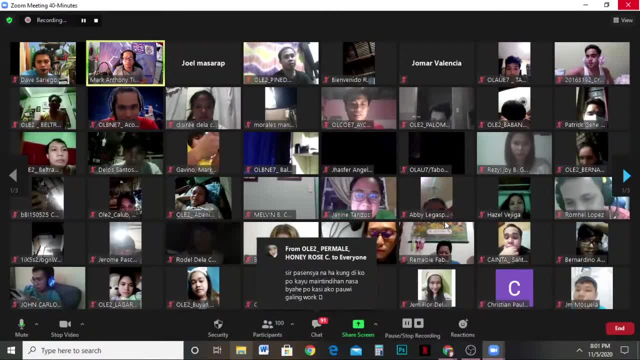 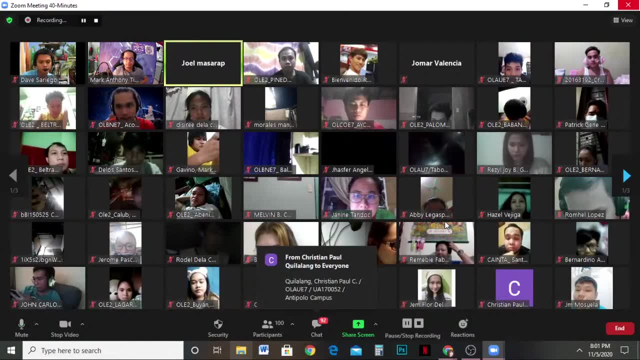 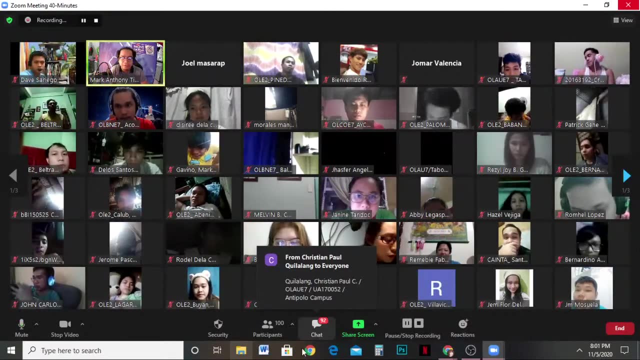 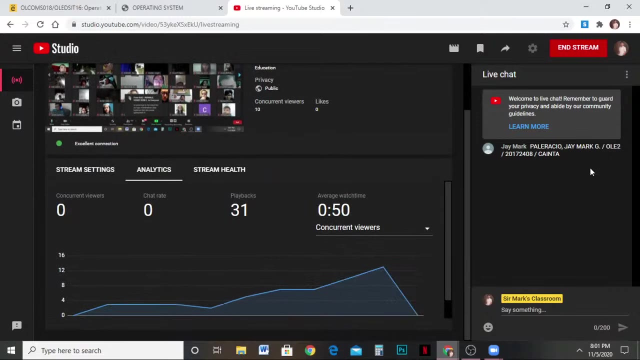 but there are still many who can't answer. sir, I'm sorry if I can't understand. I'm on a trip, ok, I'm going, ok, ok, ok, there are no questions. let's start the lesson. there are only 8 people. it's ok on youtube, the attendance of those on youtube. 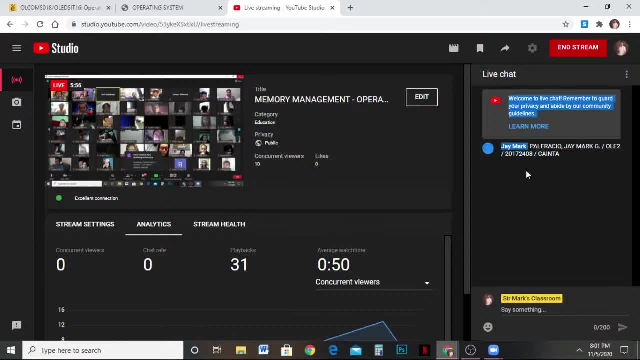 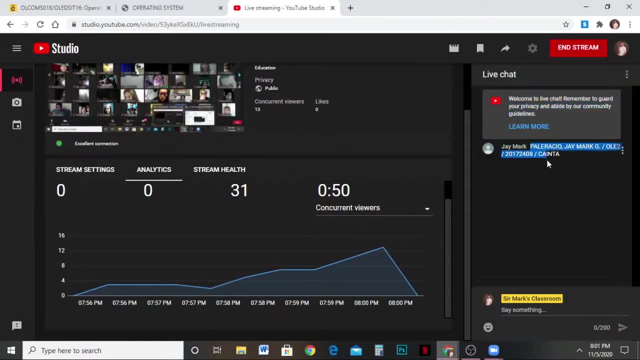 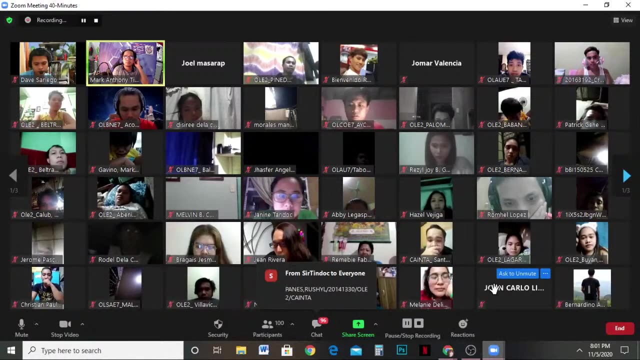 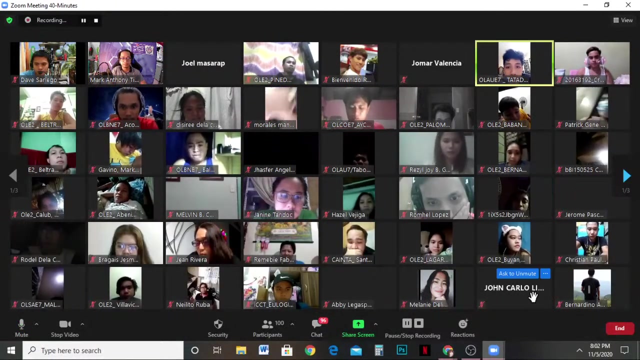 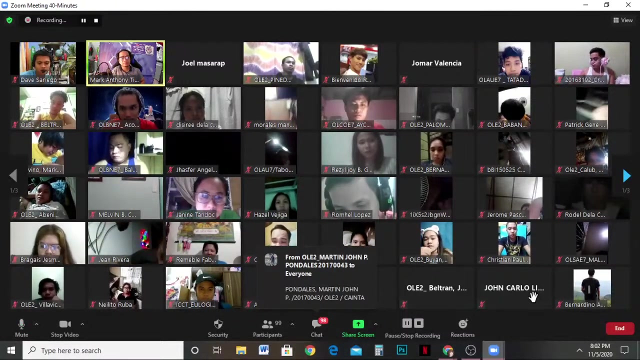 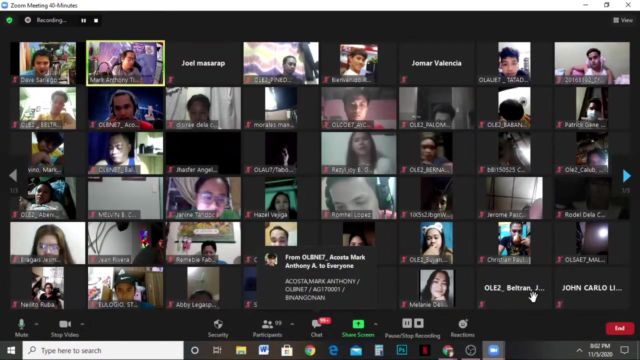 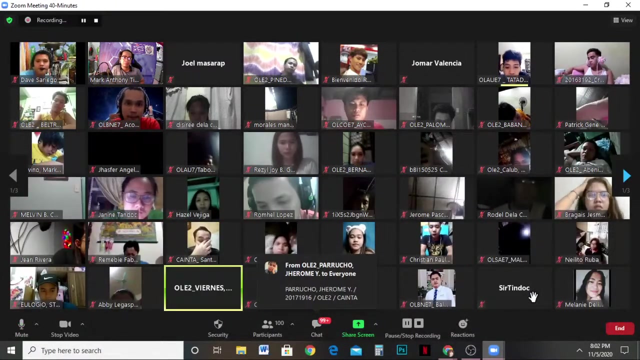 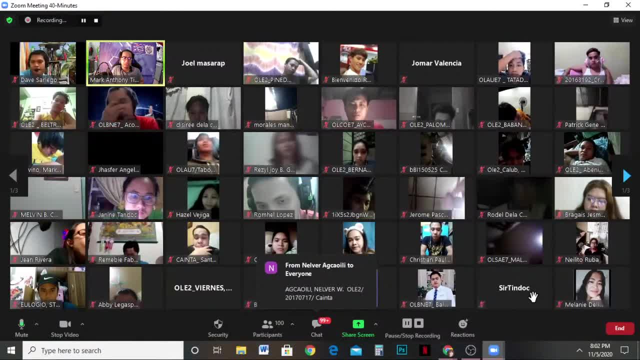 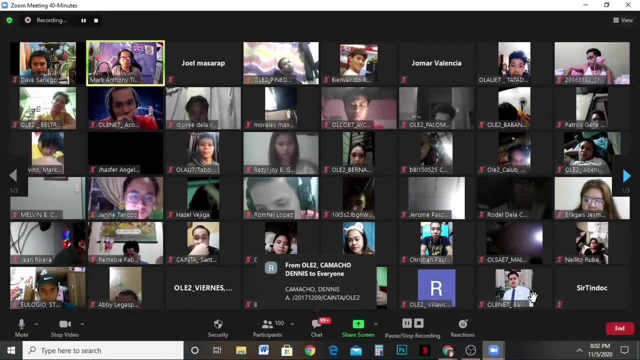 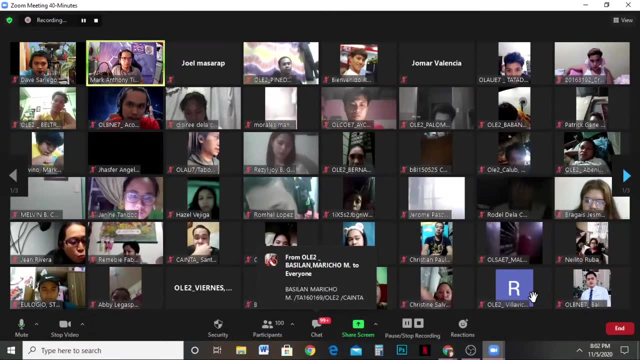 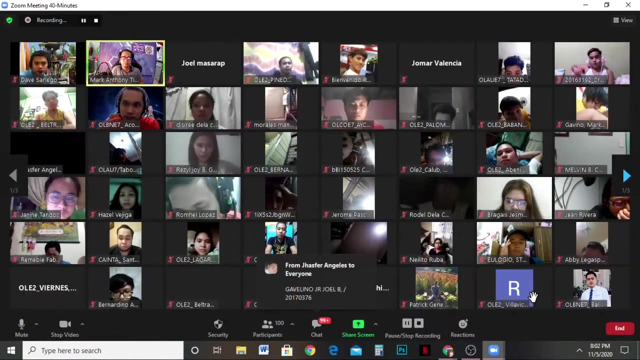 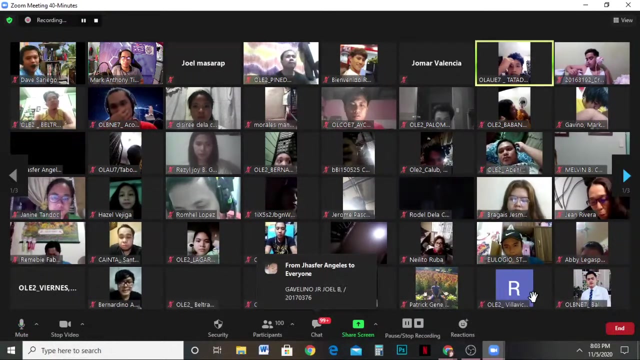 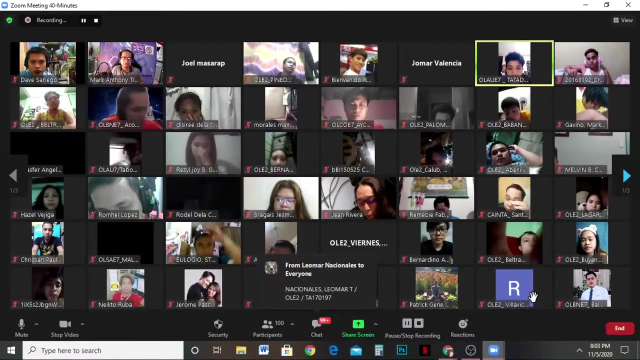 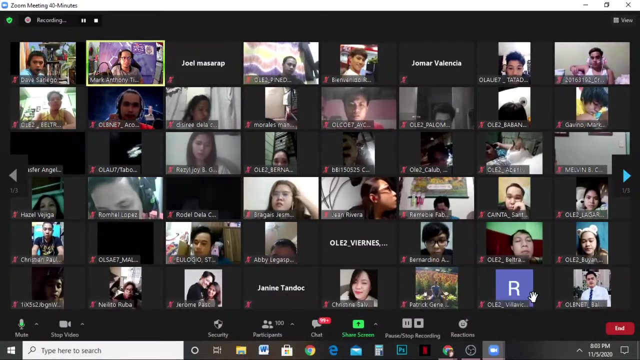 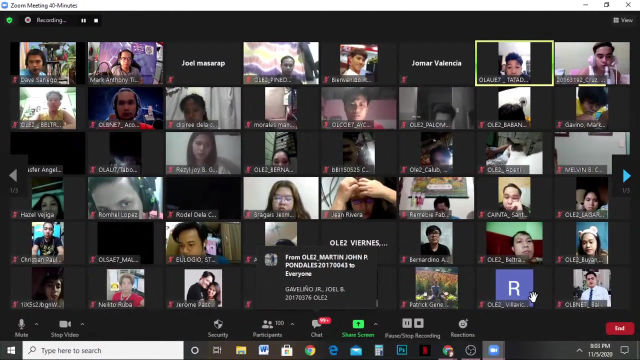 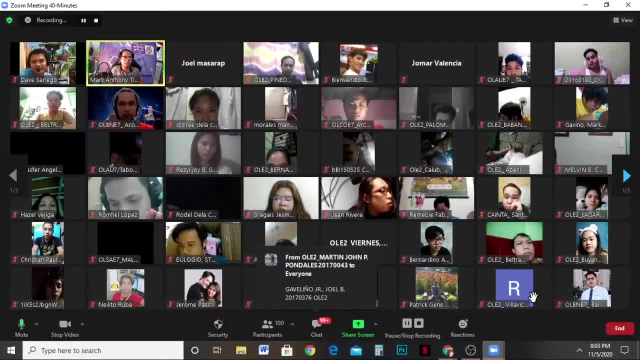 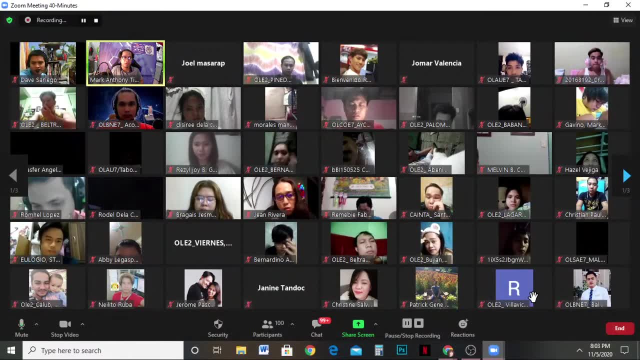 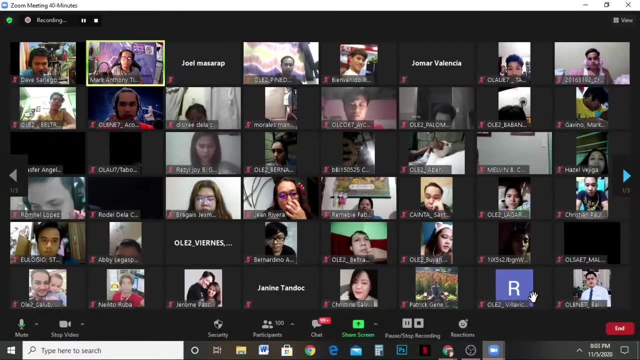 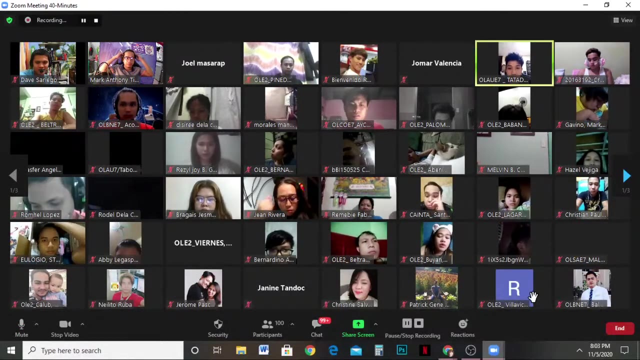 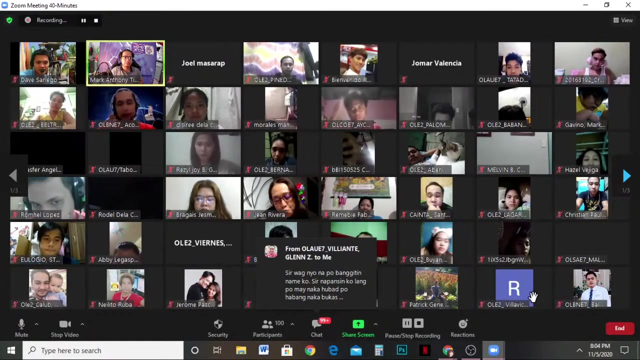 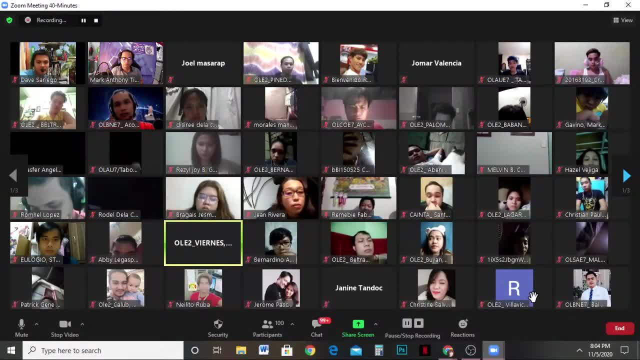 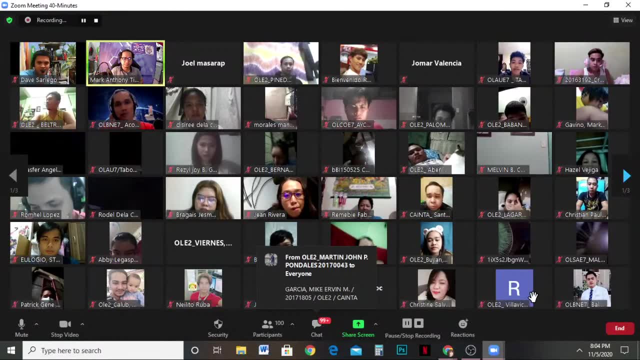 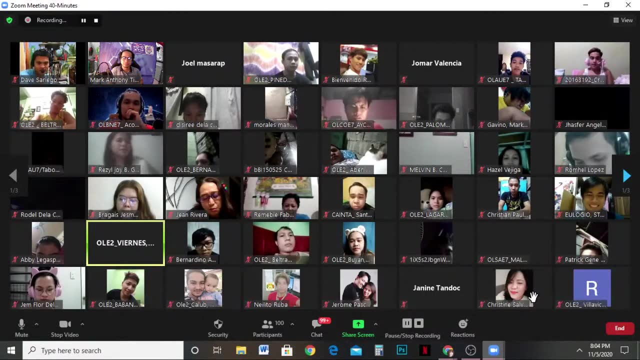 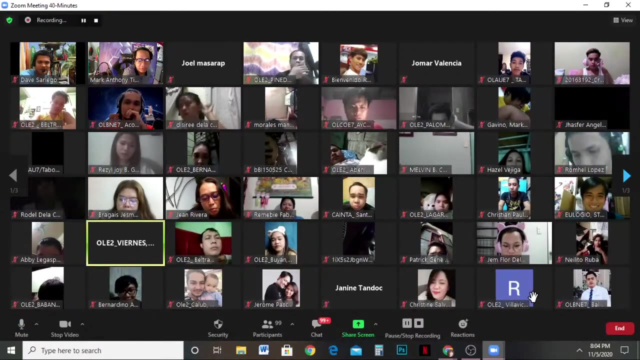 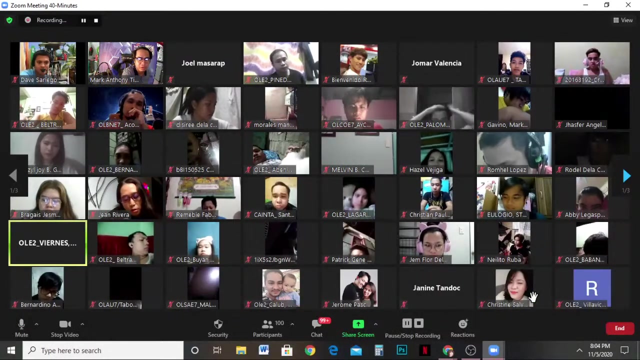 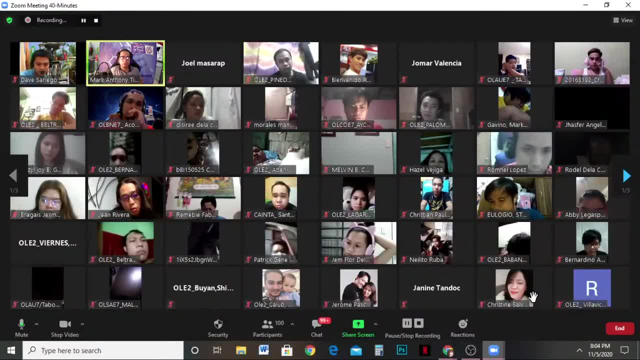 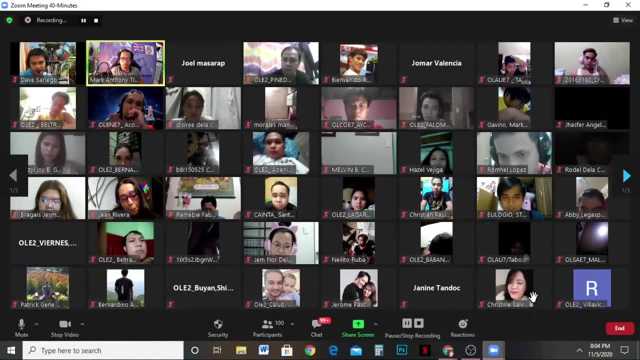 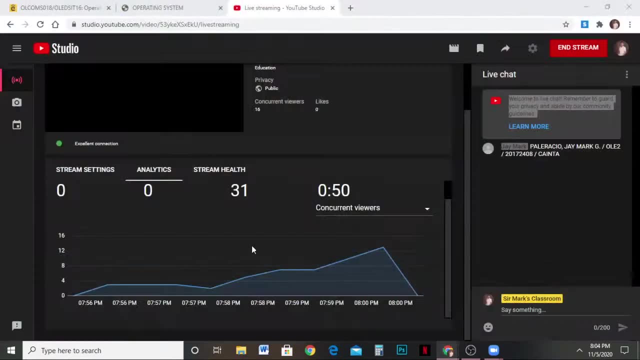 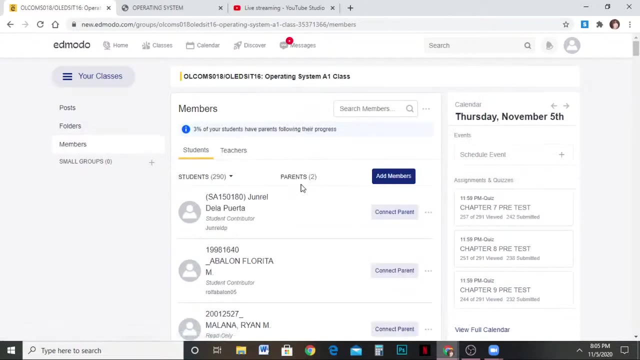 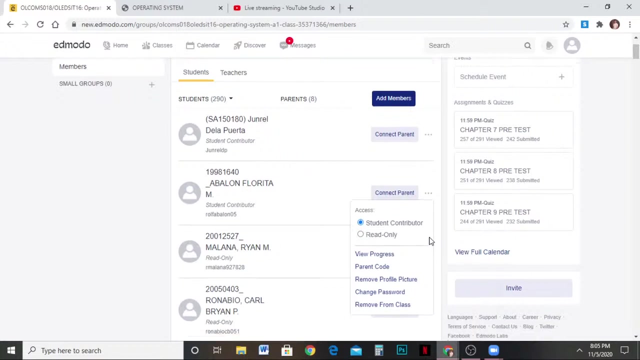 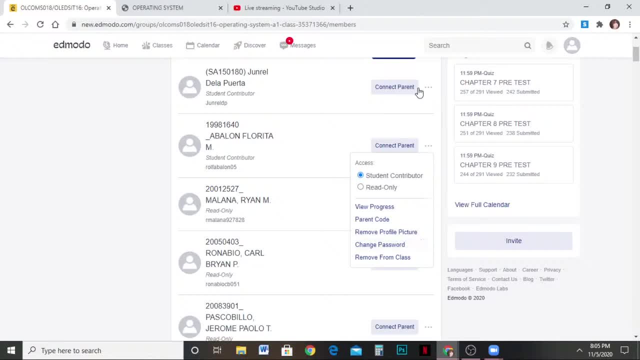 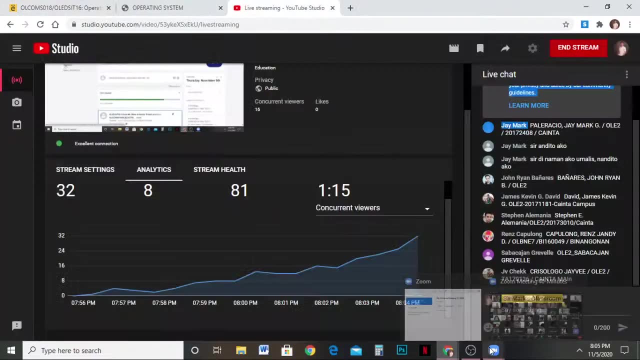 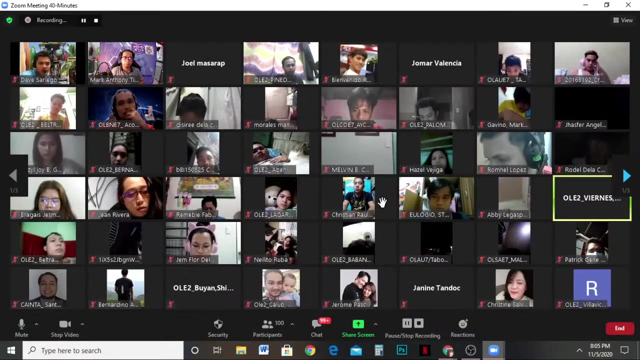 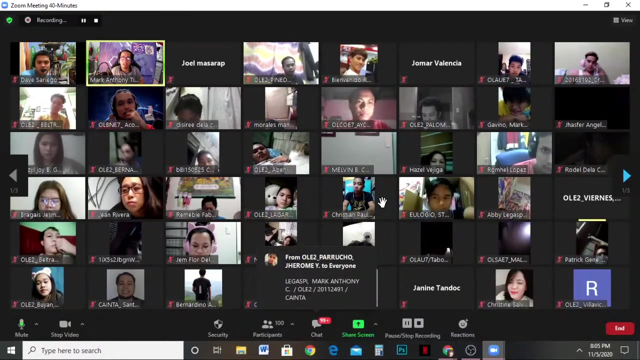 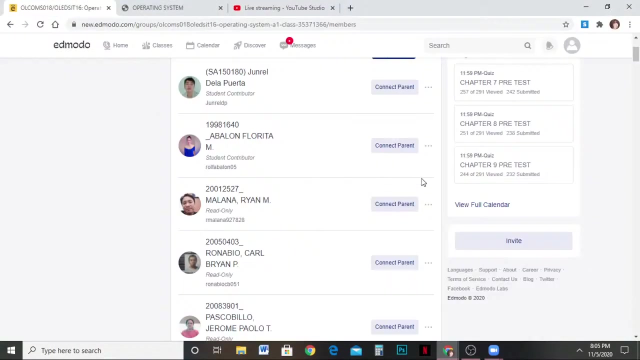 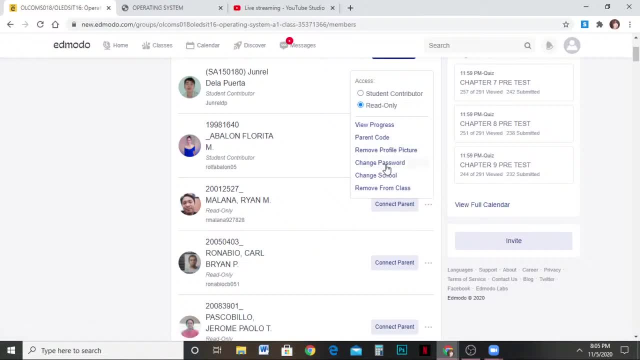 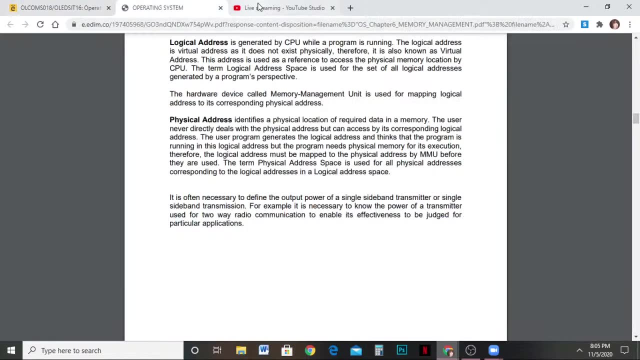 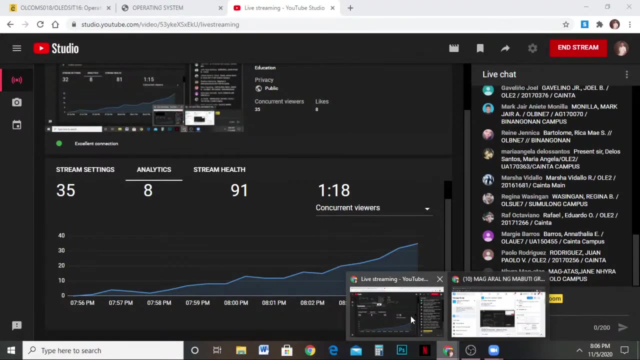 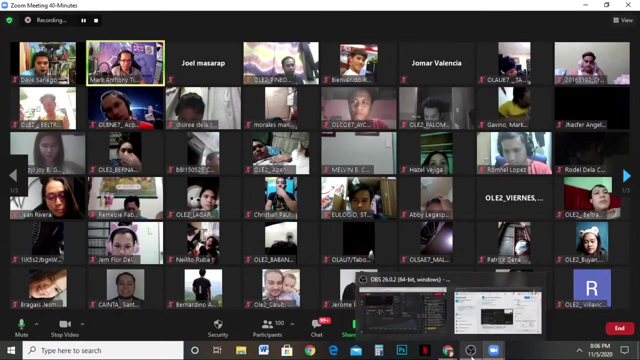 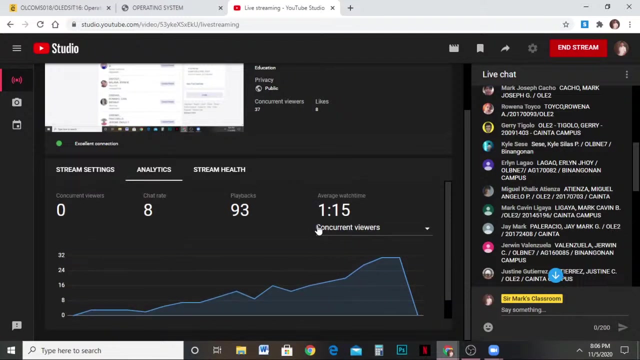 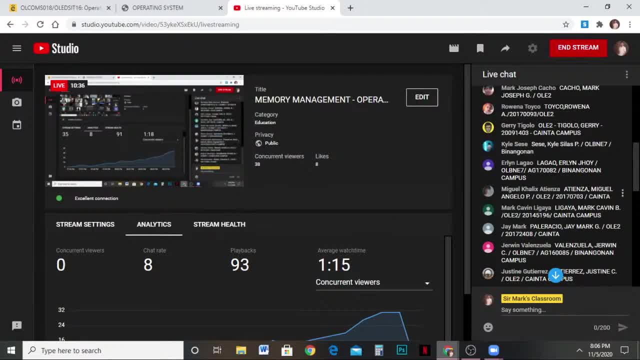 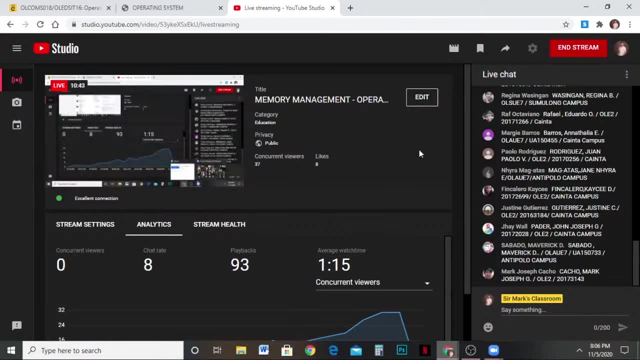 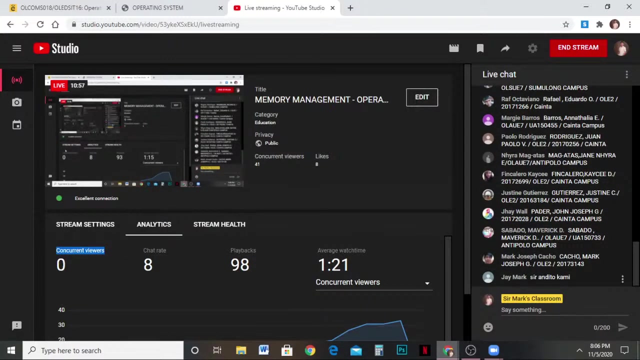 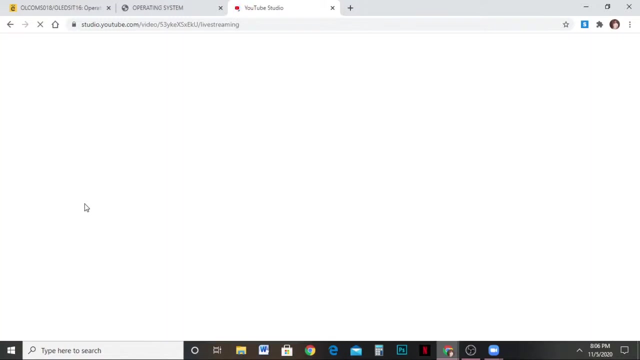 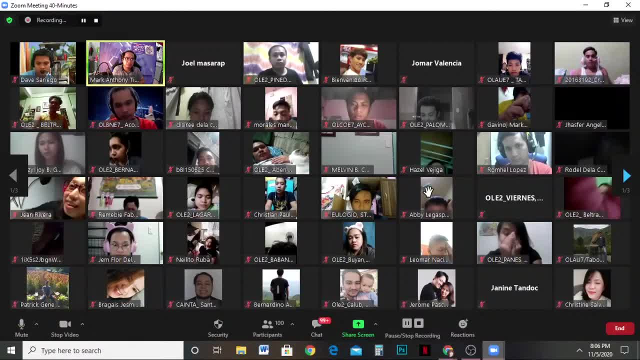 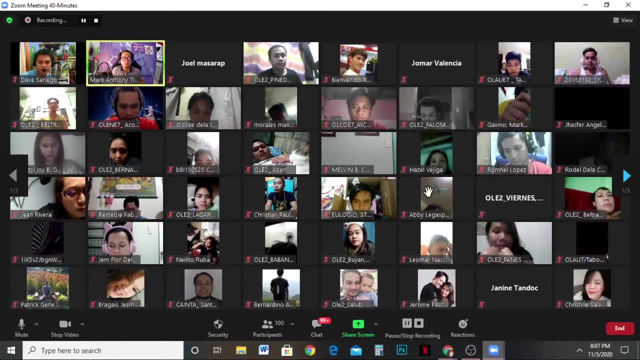 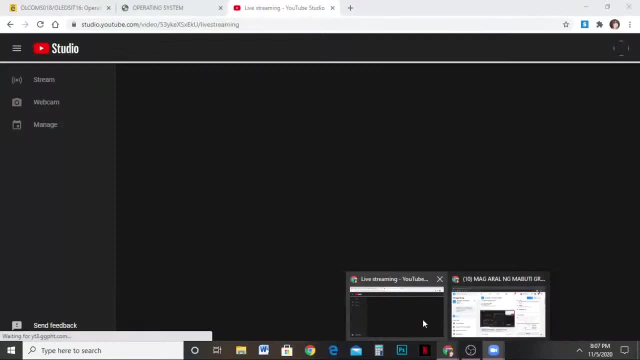 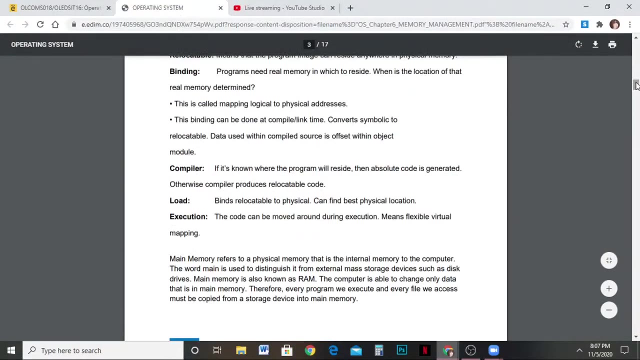 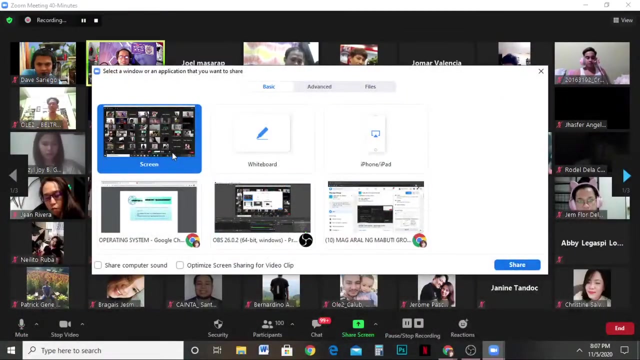 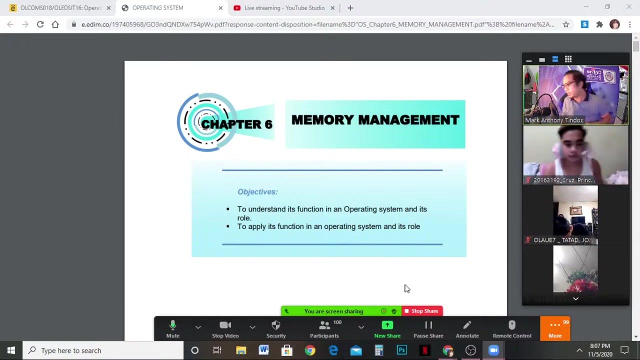 ok, ok, ok, ok, ok, ok, turn, no, no, no, no, no, no, okay. chapter 6: okay, like this, so it will be more fun. you read this already, right, okay, let's go interactive, interactive learning. I will read again: and, and where is mine? now for the 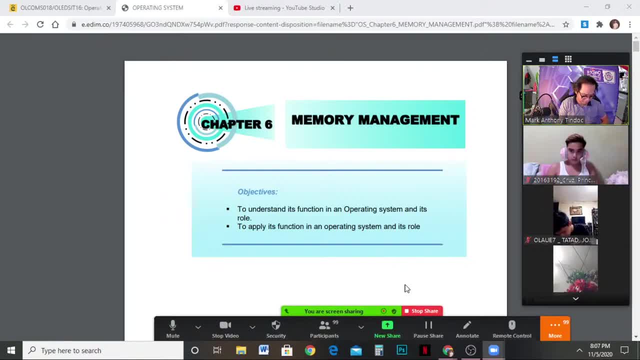 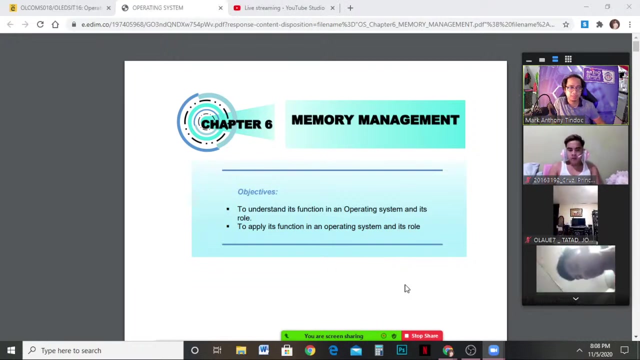 grade. okay, so last topic we talked about is process management. right, that was in the past, so before the exam, so now what we will talk about is all about memory management. memory management- the name is self managing the memory. if you read this, about what is this memory? 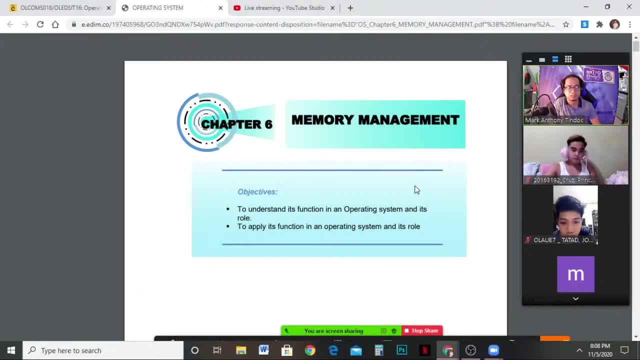 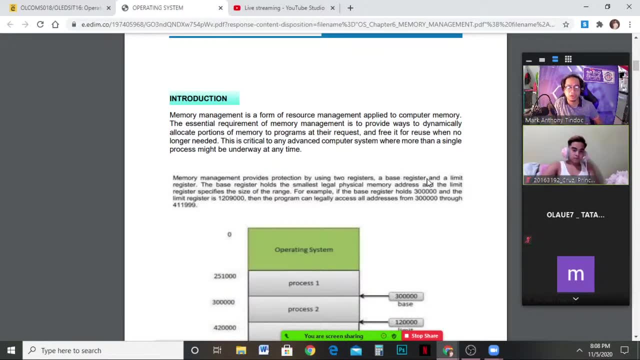 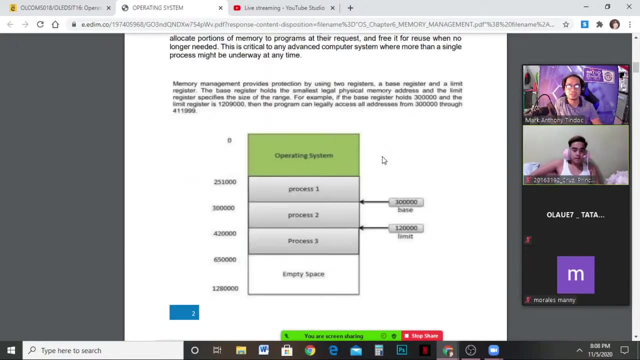 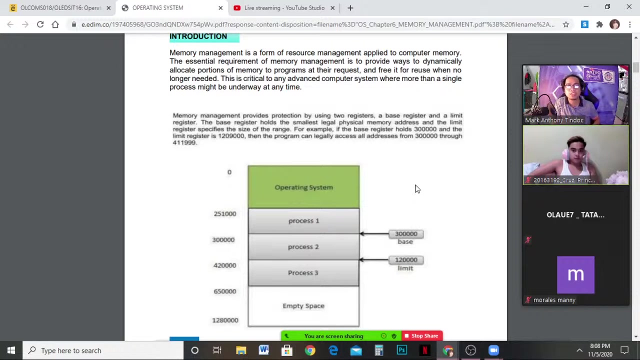 management, memory management, so you can also see anyone, okay, okay, okay, okay, okay. so memory management is a form of resource management applied to computer memory. the essential requirement of memory management is provided provide ways to dynamically allocate, dynamically allocate portions of memory to programs at their request, and 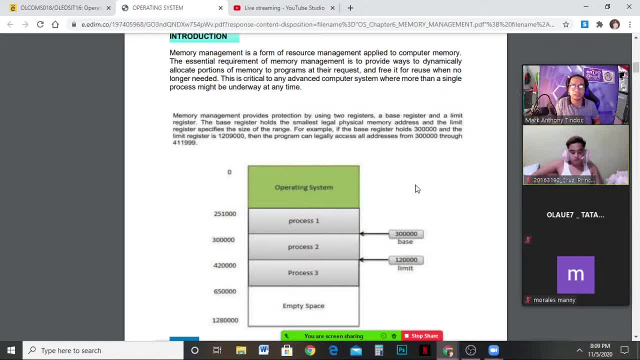 create for reuse when no longer needed. this is critical to any advanced computer system where more than a single process might be underway at any time. so this one first. the question is: ah, what is it called? ah, it is written there: allocation. actually it is called allocation and. 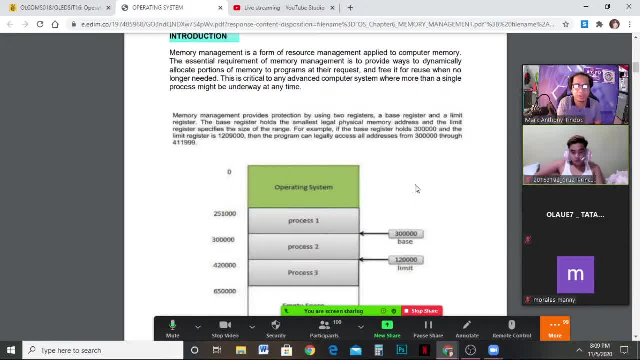 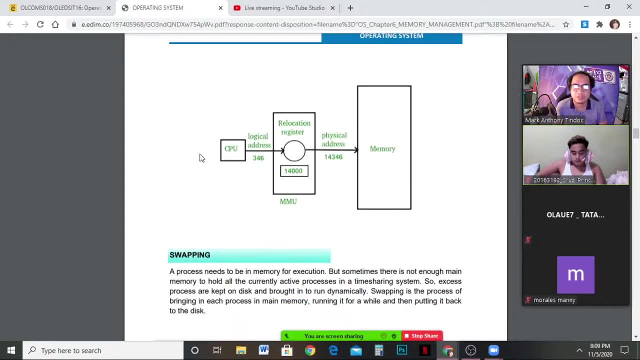 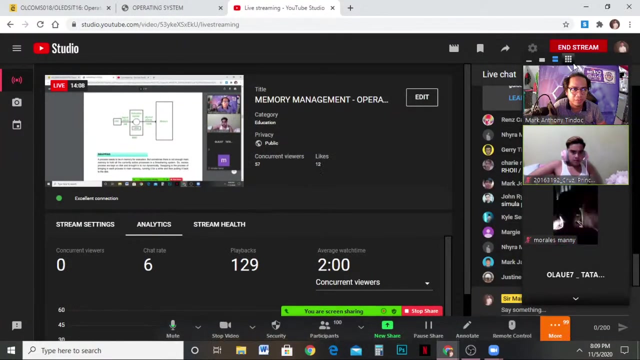 the allocation, because what happens is, if you remember what is here here, here is the processor, nothing. here is the CPU. for example, we have a program, let's just say from our peripherals. what is the peripherals? do you remember the peripherals? peripherals, computer system in youtube, peripherals. remember our peripherals? 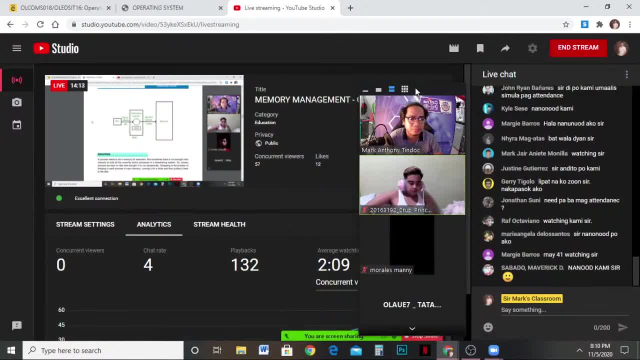 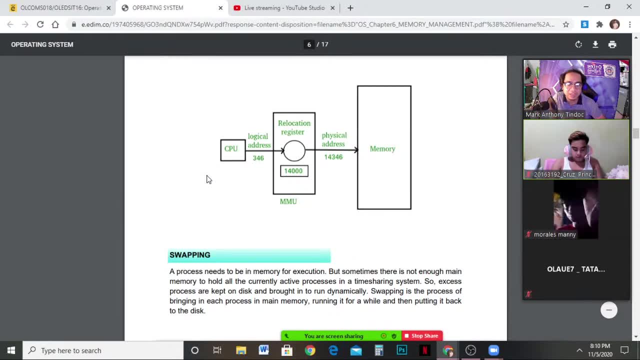 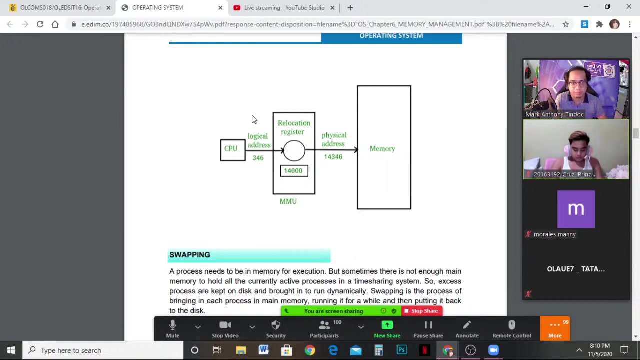 do not attend. schedule in youtube. attendance schedule in youtube. that, remember our peripherals, is the input and output. did you forget input and output devices? ah, computer mode. so input and output devices, input devices. it will go to our processor, our central processing unit, now, when it is processed. 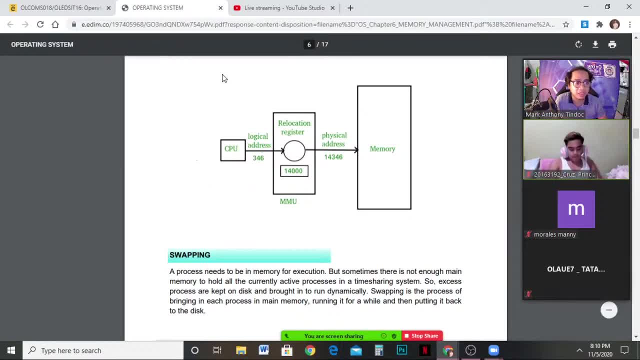 do you remember CU and ALU, CU, arithmetic logic unit and ALU? okay, now, when it is processed previously in the first year, what it teaches is just the main memory. it will get a file in the memory, but which is now the operating system that we are talking about? 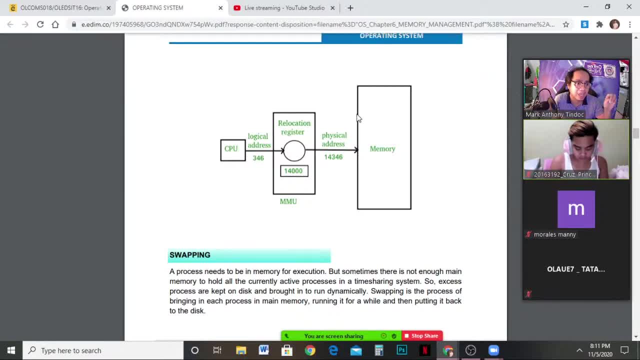 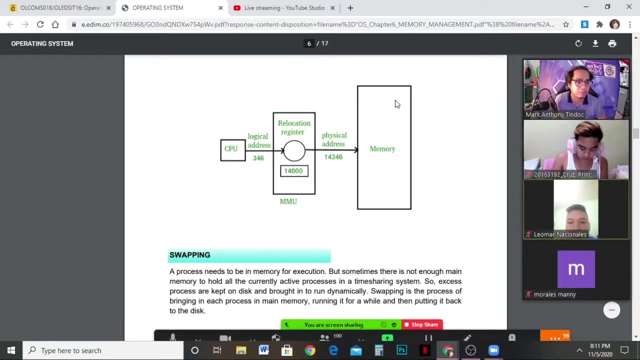 it has two classes: primary and secondary. our main memory, that's where all the files come from. so let's just back up our secondary memory. what is our secondary memory? of course those are our drives: hard disk drive, flash drive, SSD, etc. our main memory is our RAM. 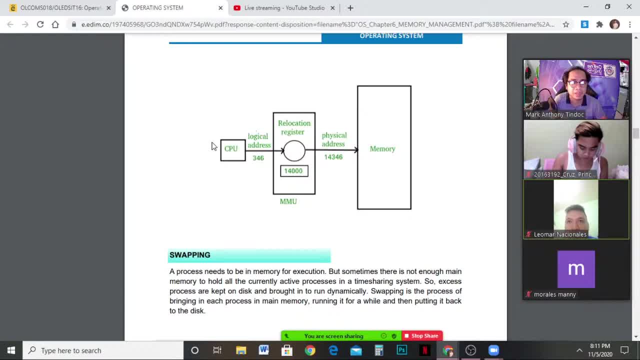 so it means every time, every time you have something to process, the processor gets a file in our main memory. so our problem is that our RAM is not that big- our main memory- so we need to have a backup. that's where our secondary memory comes in. so what happens is: 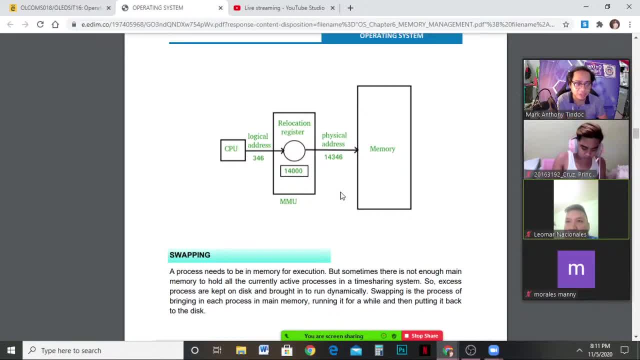 we know that our main memory is temporary. what happens is, every time we allocate a file, we will get a file. we also remove the file, the allocation. okay, we are freeing some space for us to use. so, if you notice, every time we turn off our computer, our memory loses power. 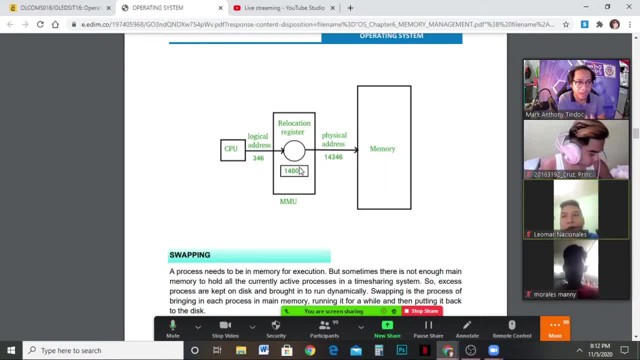 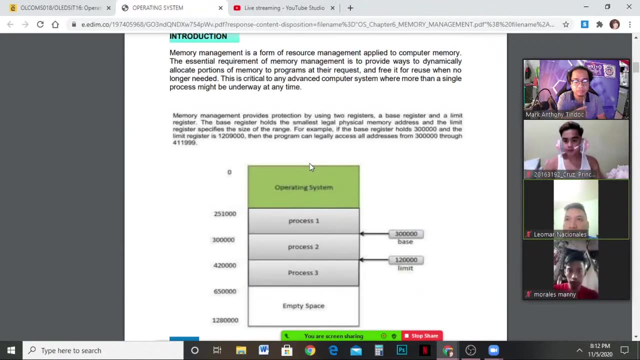 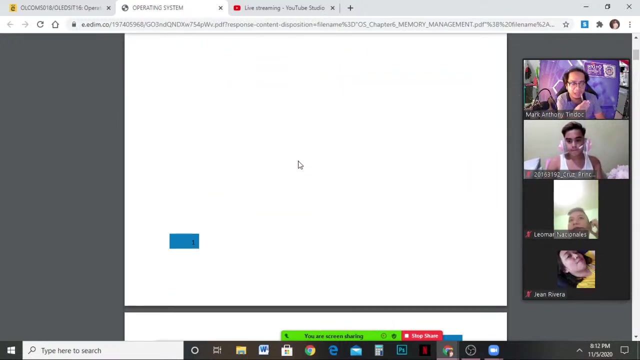 our files are deleted, our temporary files are lost, our temporary storage when. what happens when we execute a file or when we execute a program? so that's what we are going to talk about here: in memory management, what happens when we allocate and deallocate and when we locate. 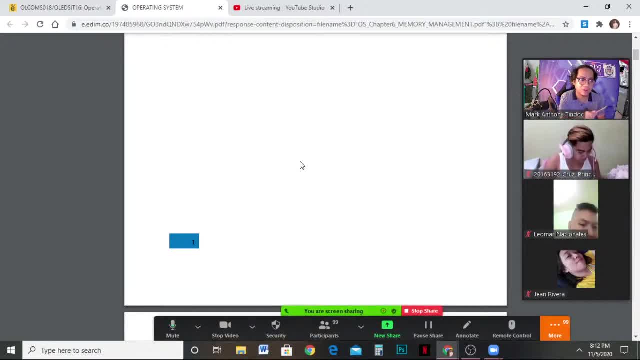 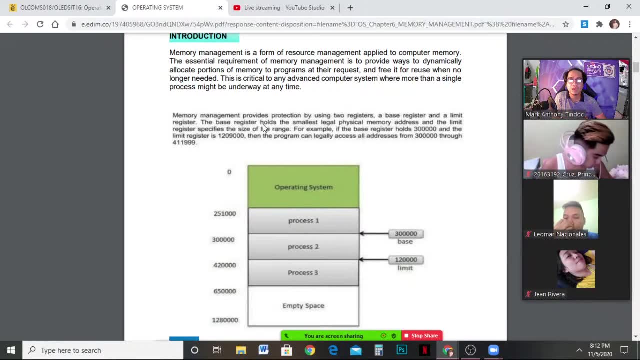 the space for the file or the program you want to execute. okay, okay. so this, this memory management provides protection by using two registers. okay, the base and the limit. so this base and limit is the range. okay, this is the protection. this is the protection of your computer. 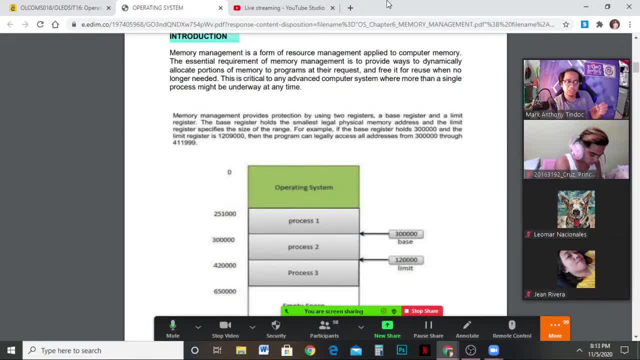 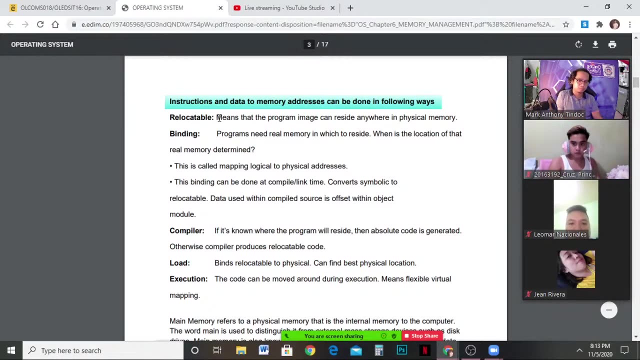 for what? so that it's not too low and not too big when you allocate it to your memory. so that's the work of the operating system: file management, memory management, sorry, memory management, sorry, sorry, sorry. I said it's replaced, so these are the. what do we call it? 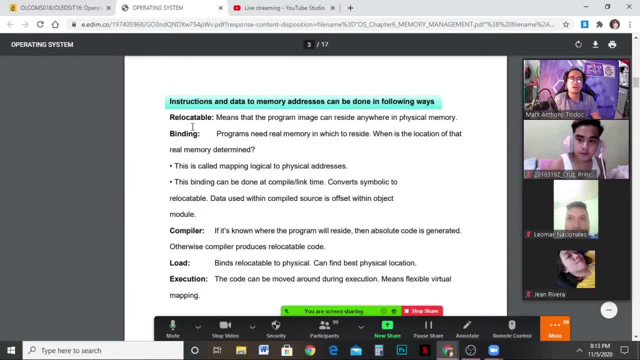 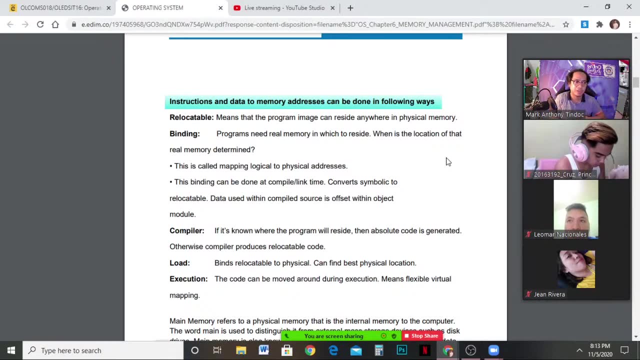 the terms we need to remember. relocatable means that the program image can reside anywhere in physical memory. what is physical memory? okay, that's it. there are two. we have physical and logical memory. what is physical memory and logical memory? sorry, sorry. physical address and logical address. what is physical and logical address? 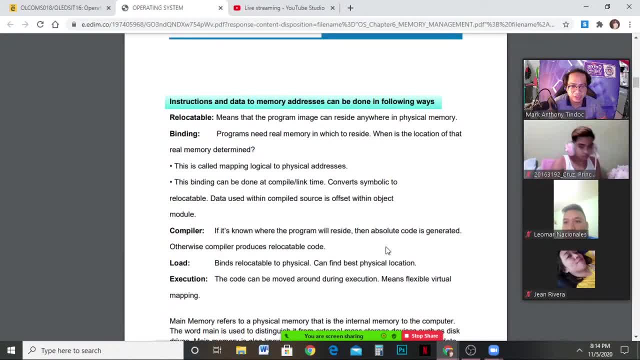 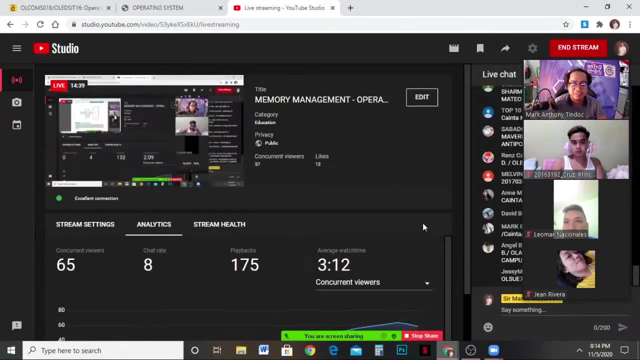 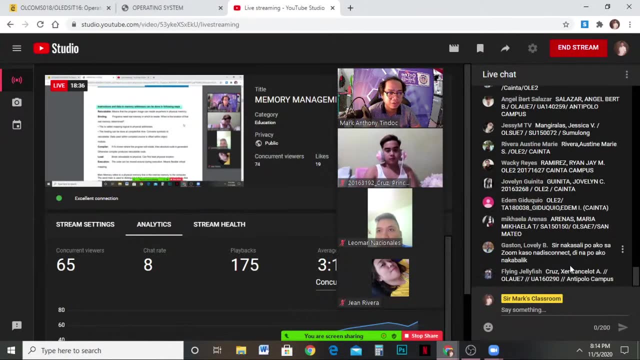 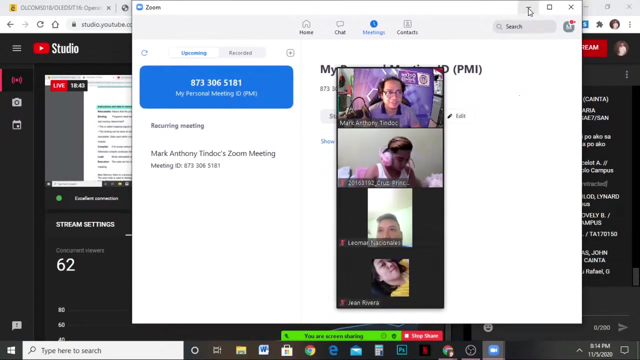 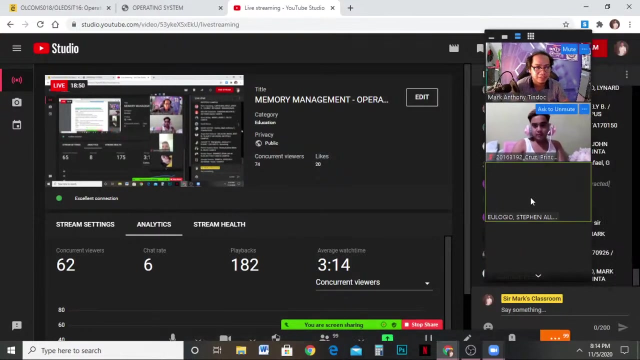 anyone physical and logical address on youtube? I'll just tell you. okay, type your name when you answer. this is real time, I can see you, so I'll just call. I'll just call zoom. I'll call sir. okay, go sir. what is it? the physical address? it's like the form. 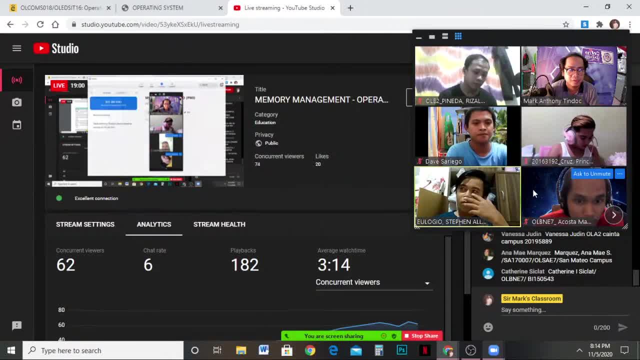 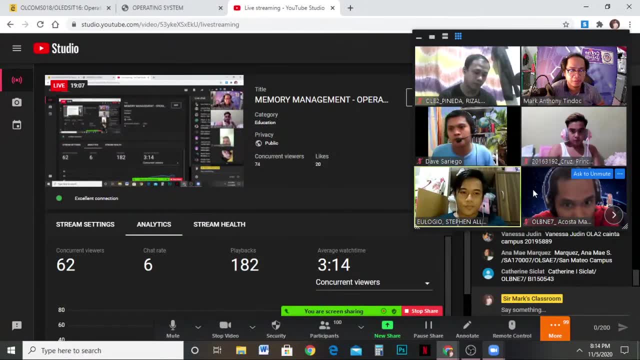 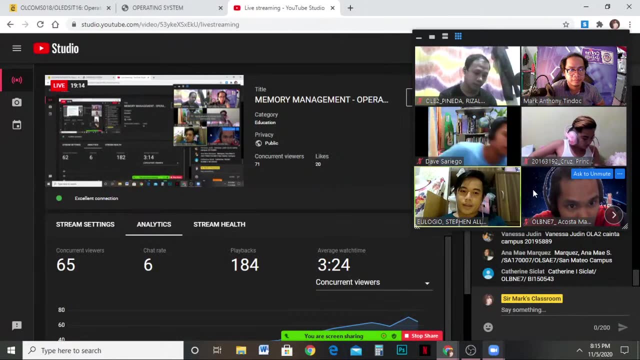 that? what is it called here? I'll just explain: orbex gray, it's binary, mmhmm. the physical address for me it's like um, it's like it's a memory address represented by a binary number, something like that. okay, there's no idea I'm able to remember. 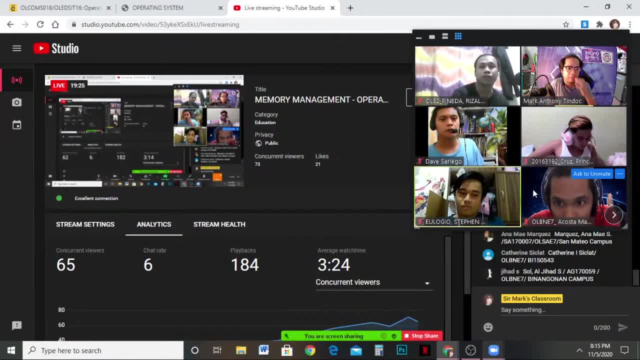 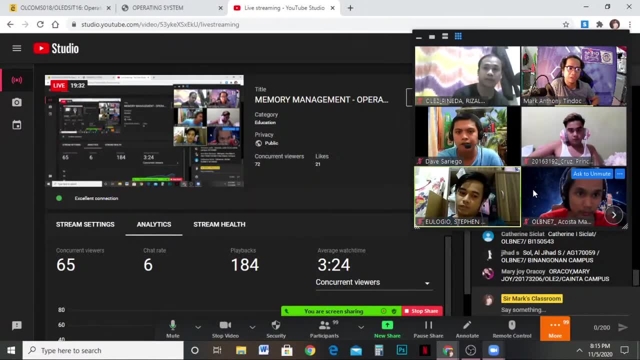 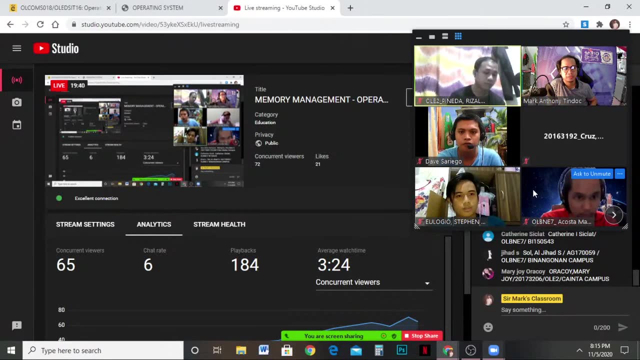 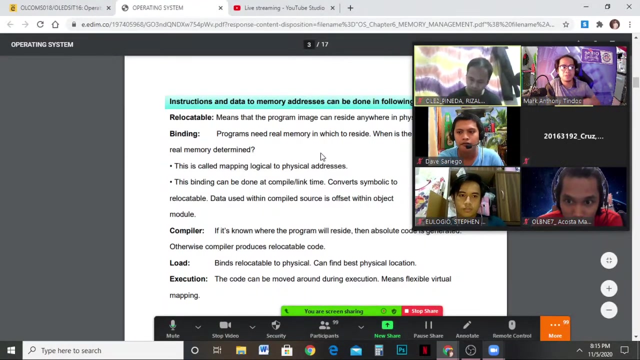 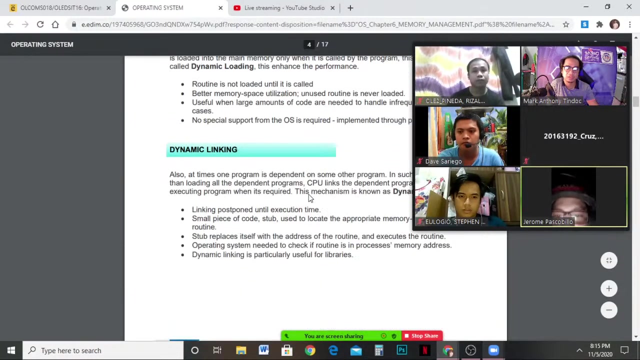 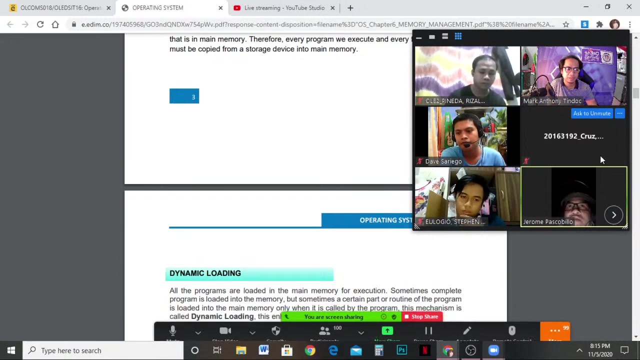 okay, actually that's space, that's right. that's the specific address of your memory, okay, okay, other than that, the difference between the two in the physical address and the logical address in the physical address. that's where the computer is getting the address. wait, sorry, sorry. so what you said, 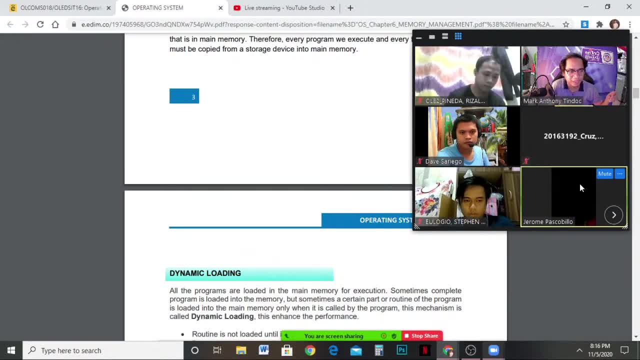 the computer is getting the address. the computer is getting the address. we are talking about the network, ah memory. that's where the computer is getting the data. that's where the computer is getting the data or address in the memory of the computer, whereas the logical address is embedded in the 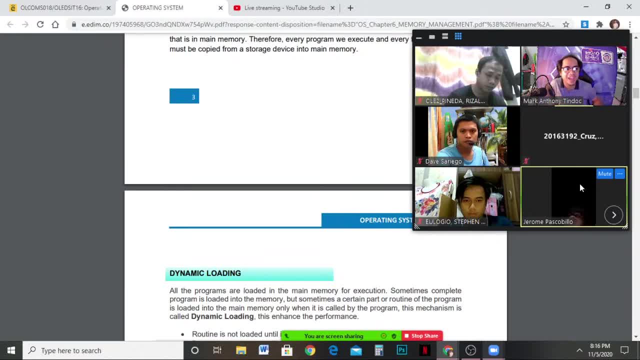 IP address of the networks. hmm, I was just saying we are talking about the network. I'm familiar with it. okay, that's right, that's right. but that's good, that's right, that's right. I'm still working on it. okay, okay, okay, okay, pass, okay, go. 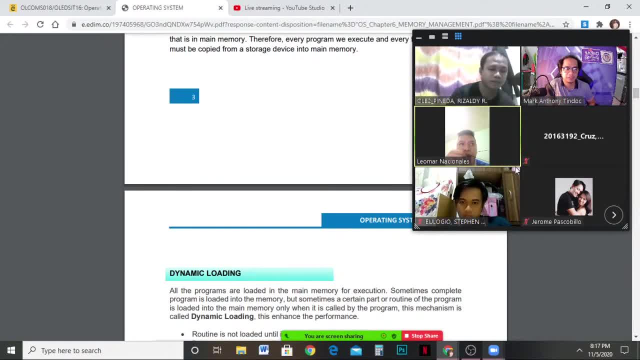 the physical address is what the house is representing, okay, and the difference between the logical address. that's what the house is representing. that's what the house is representing. to secure the application or program: okay, to secure the application or program. okay, okay, okay, okay, okay, okay, okay. 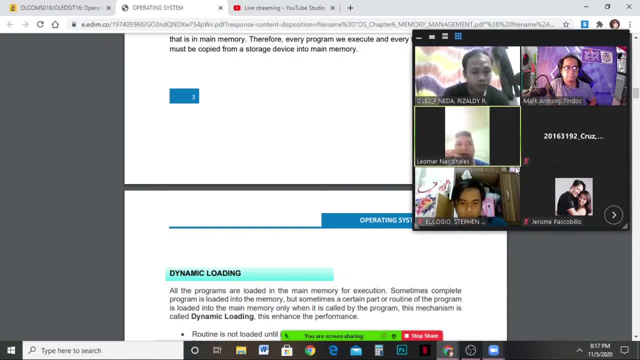 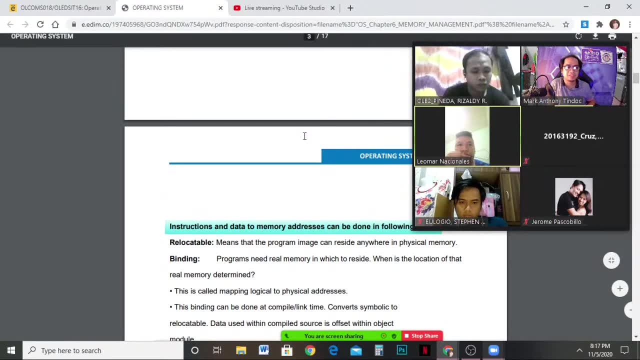 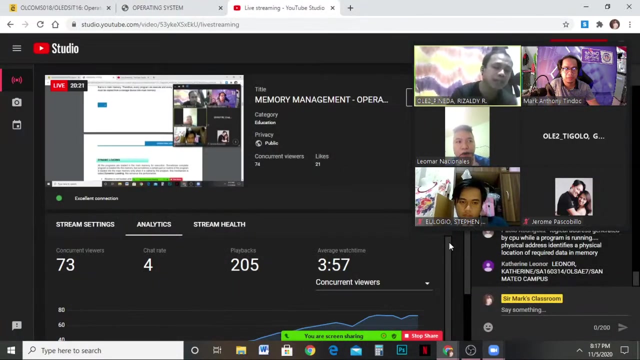 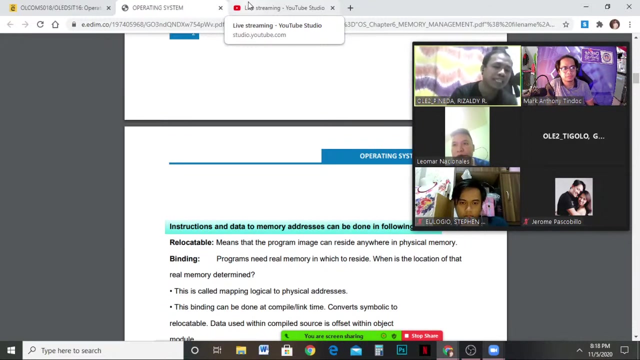 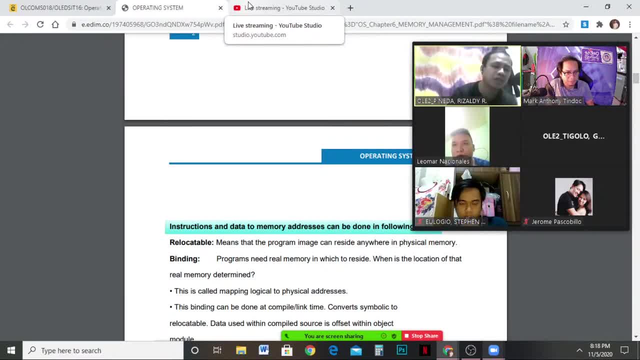 is the location that exists in the memory unit. Okay tama, Actually yun yun Kasi ganda yun Logical address is parang ano lang siya: Imaginary, Virtual, Virtual or imaginary Provided lang siya. 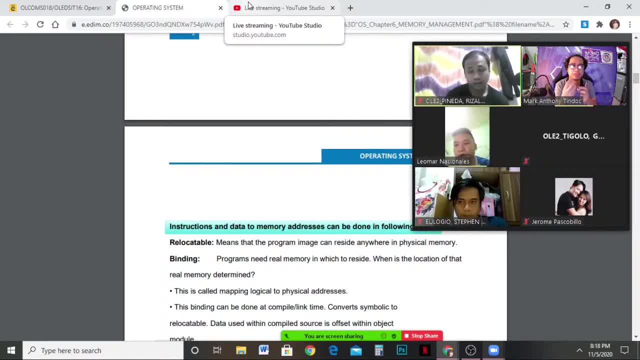 by the device CPU. Sabi nga niya kanina Provided siya ng CPU, Sabihin si CPU yung nagbibigay ng logical address mo. Okay po, Tapos i-re-register yan, I-cocombine yan. 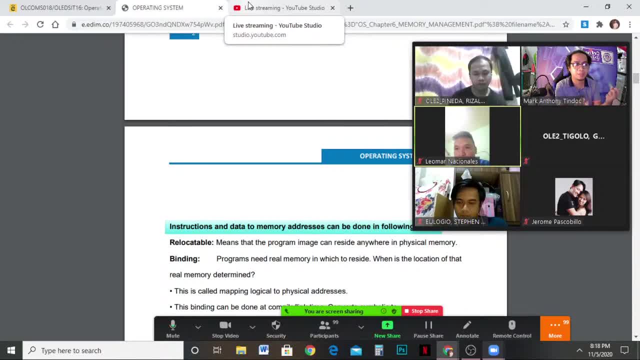 together with your physical address. Okay po, Yung physical address is mismong location dun sa mismong memory mo, Yung main memory mo. Okay po, Ibig sabihin kung saan siya nakalocate dun sa main memory mo. 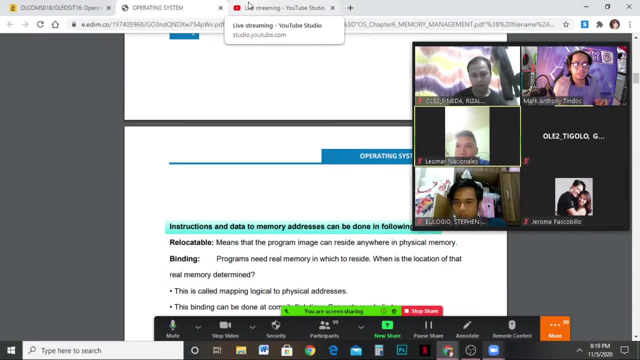 yun yung physical address mo. Yung logical address is provided by your processor. Parang ganito, para mas maano kayo, bigyan ko kayo ng analogy in network. I-analogy natin in network, Parang ganito siya: 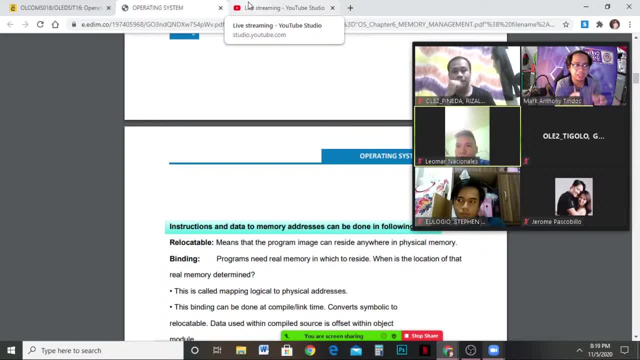 Diba, kung maaalala nyo sa network pag sinabi nating physical address, that is the MAC address. Ano, yung MAC address, sir Yun. yung location nung device mo Yung address. 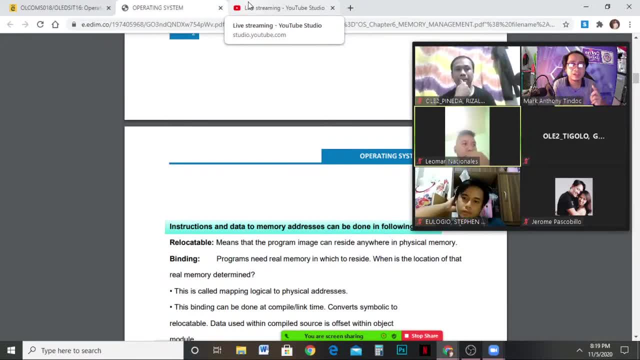 nung device mo Gets po. Eh, sir, ano naman yung logical Yung logical ayun, yung binabanggit kanina ni Pakobilyo, which is IP address Yung IP address, provided naman siya. 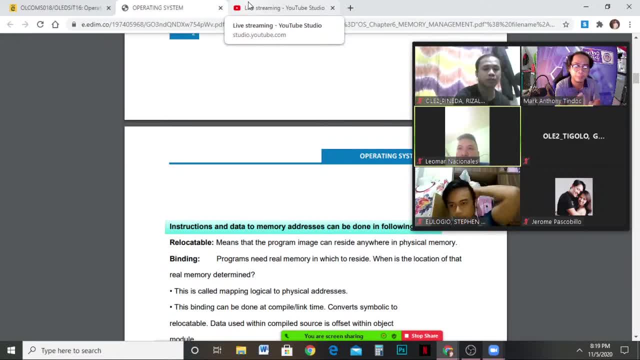 through the net. Through internet, Kung mapapansin mo, pwede ka magpalit-palit Nang IP address. tama, Paano nagpapalit-palit ng IP address? Paano nagpapalit? 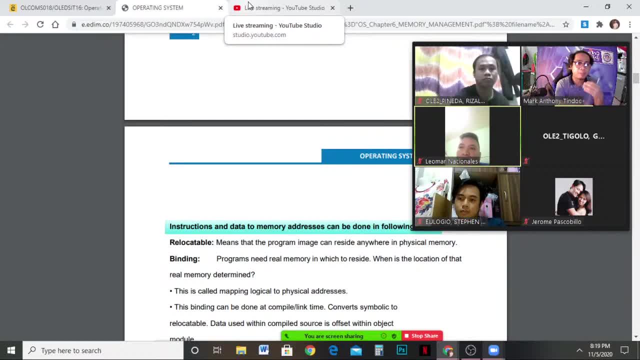 Kasi every time papatayin mo yung computer mo mangyayari magpapalit yung IP address mo. Bakit Magpoprovide na naman ng panibagong IP address sino yung World Wide Web? 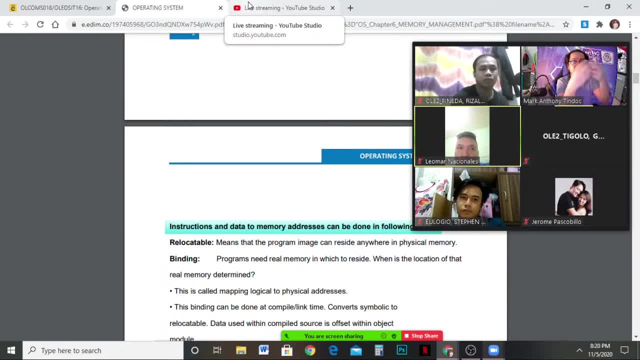 sa'yo Gets po. Parang ganun din pagdating sa ano natin, sa computer natin, yung memory natin. Ang mapoprovide ng ano natin, ng logical address, logical memory is CPU. 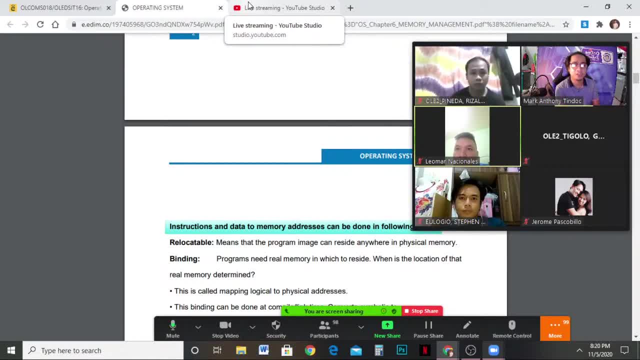 Yung processor mo. Okay po Ngayon ipapasok yan meron dyan ire-register yan para saan Iko-combine yan dun sa physical address mo para alam nung ano nung register mo. 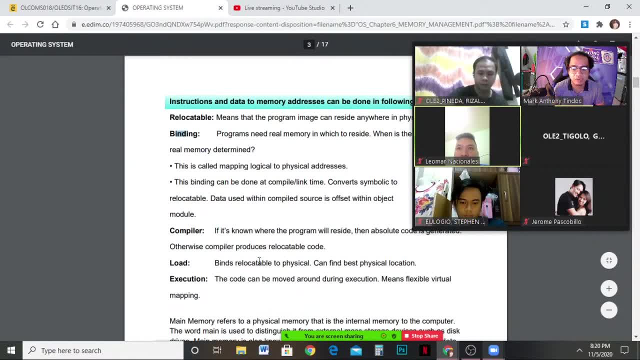 nung compiler Yan na to to to Nandito na Compiler Nabasa ko kanina, Ito Compiler Kunsaan niya ilalagay yung actually hindi si compiler, si loader. 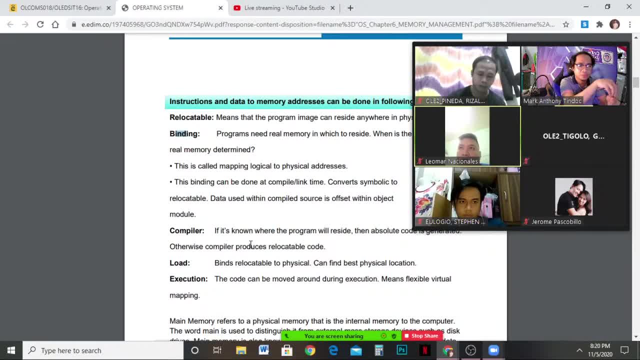 Yung kunsaan niya ilo-load yung ah data O saan niya kukunin yung data? I-execute na data mo. Okay po, Para mas mag- Sayang, pwede mo mag-drawing dito. 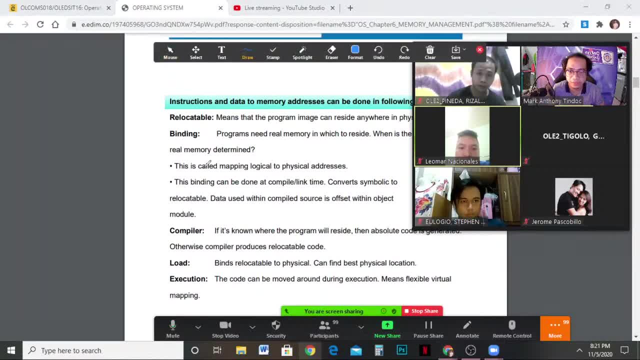 Wait lang, ah. Alam ko pwede mag-drawing dito Yan Drawing Yan Pwede Nakikita nyo ba to Ah ito Example, ito si CPU diba Ito kasi yan. 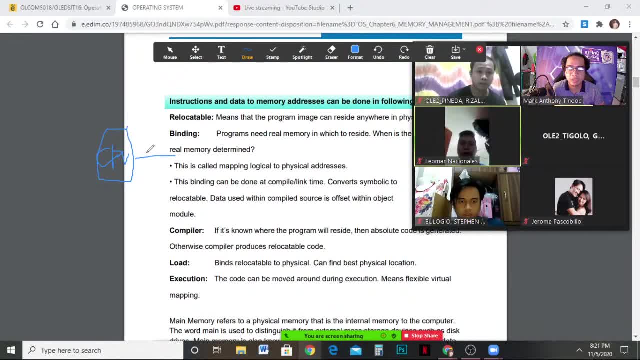 CPU. okay po, Tapos magpoprovide siya ng logical address, Logical address. Logical address L-A. Gets po Pag-provide niya ng logical address. meron kasi dito compiler. May compiler dito. 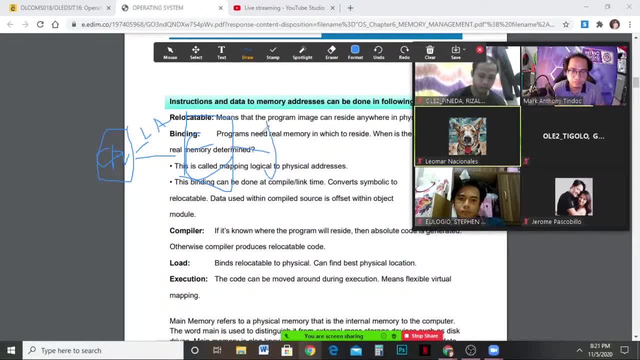 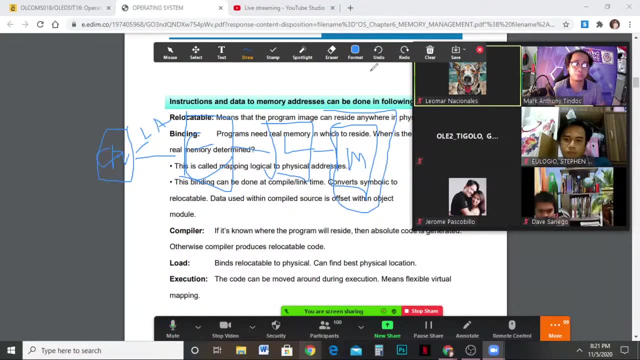 see: Tapos ilo-load, Load, Tapos memory Memory. Okay po main memory. Now ganito po yung nangyayari. ah, Ito yung pinaka-cool process niya. 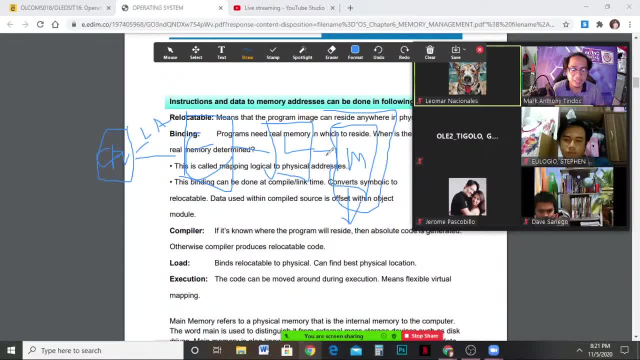 ngayon, kapag hindi ka siya dito, kailangan mo ng backup. This is your secondary memory. Susundan ba Okay po Now example dito magbibigay ito ah address niya. 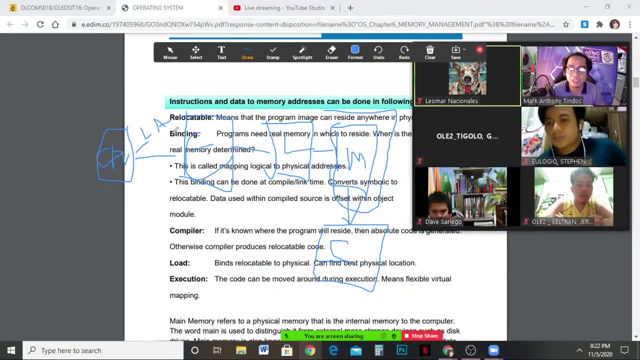 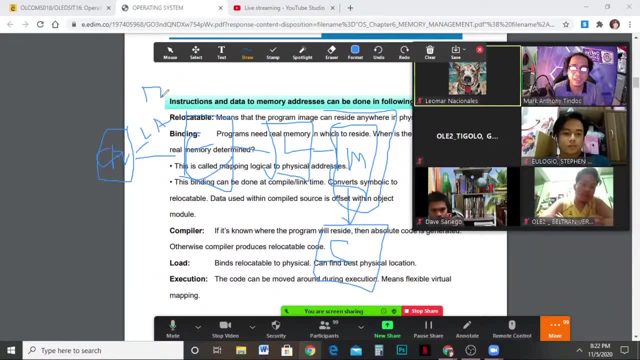 nari ang address niya: A Ah, A Nag-provide siya. A Okay po i-cocompile yan, ilo-load yan, tapos meron siyang allocation dito. Okay po i-cocompile yan. 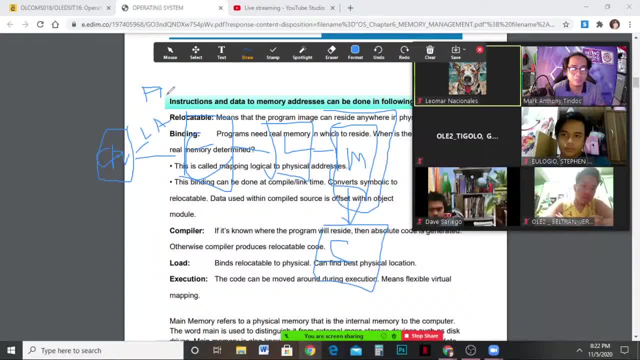 ilo-load yan, tapos meron siyang allocation dito: Okay po, i-cocompile yan ilo-load yan, tapos meron siyang allocation dito, Ang adres dito, number naman one. 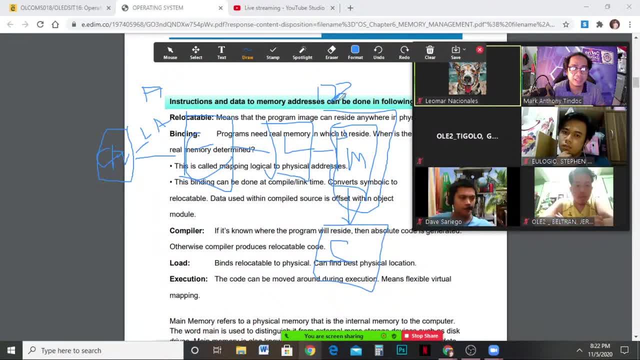 two, three. That is your physical address. Okay po, Combining with, provided nakikita niyo ba, Nagigets niyo ba Yung drawing ko. So ulit, ah, ito magpo-provide kunyari. 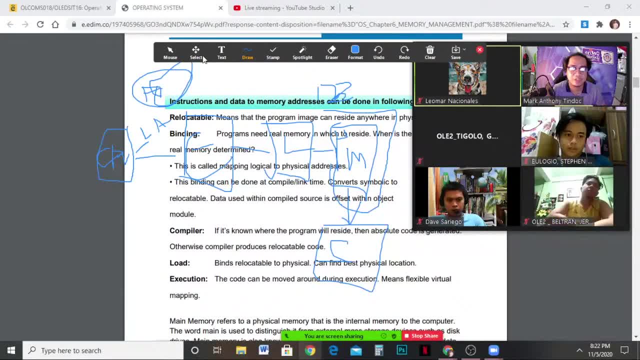 A, A yung pin-provide niyang address mo. Now ang mangyayari? ire-register yan, So ulit. ah, ito magpo-provide kunyari A, A yung pin-provide niyang address mo. 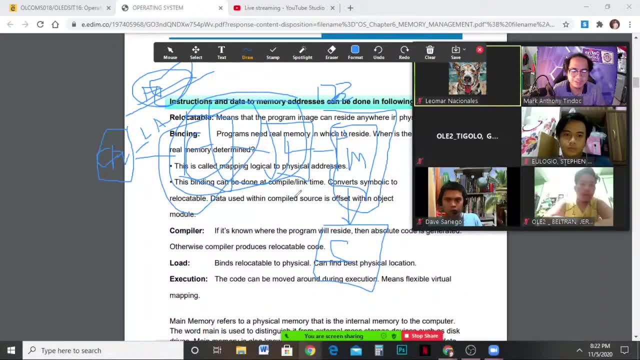 Now ang mangyayari: ire-register yan. Ito pala may text, eh Nandun natin. Okay ulit, Spotlight, Ito pala may drawing ko Draw Saan na I don't see. 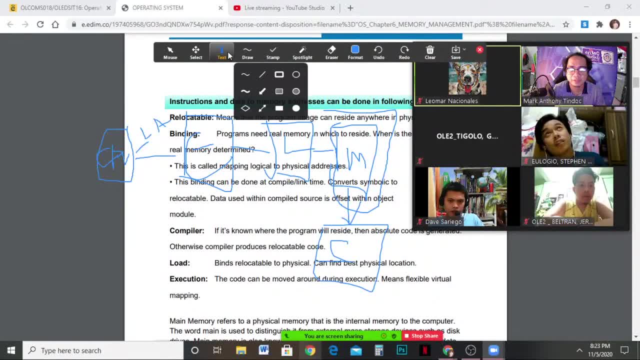 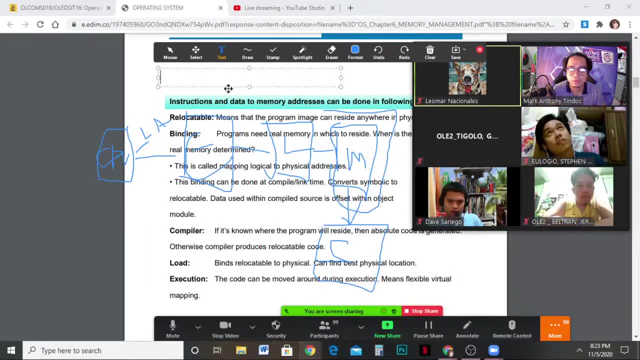 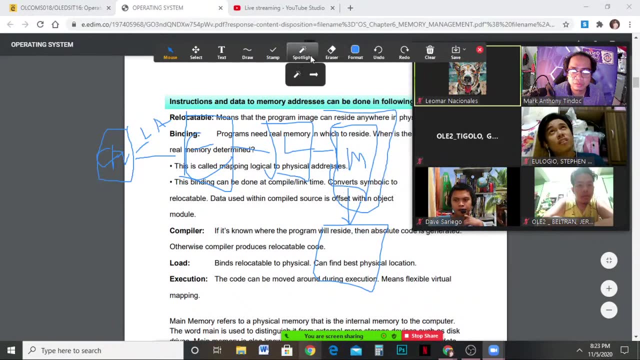 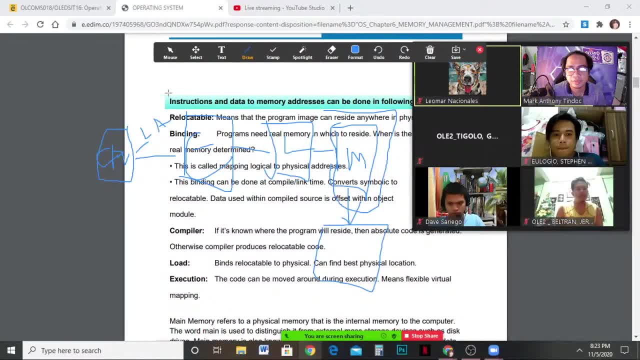 oh no, it disappeared. oh, there it is. and A okay, after A. then here it has an allocation here. it has an address here. for example, its address here is 1 or 11. only what will happen is for it to be located. it will be provided it will be 11. 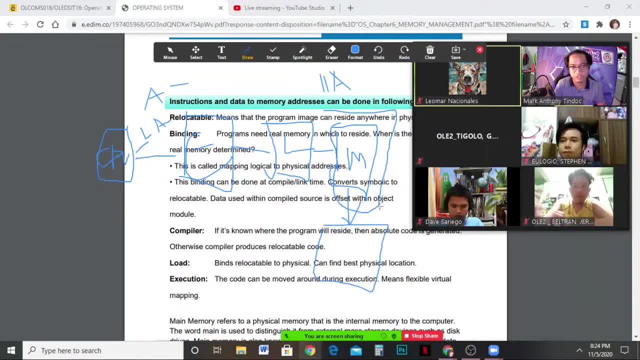 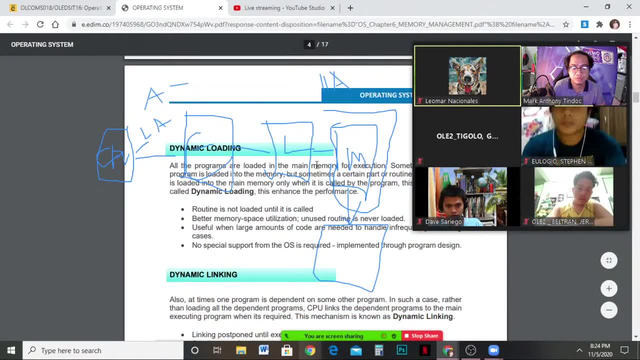 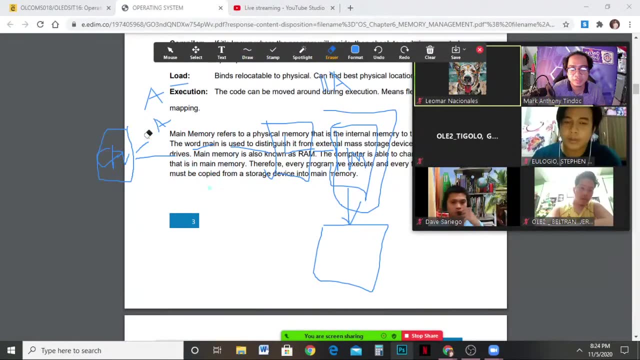 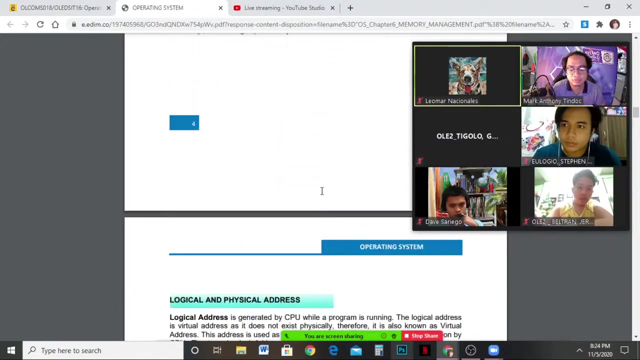 get it. this is your executable program. I hope there is one here. wait, I hope there is one here. it's blurring. get out of there. it's going to be explained if I hope there is one. oh, there it is. I explained it earlier. this is it. 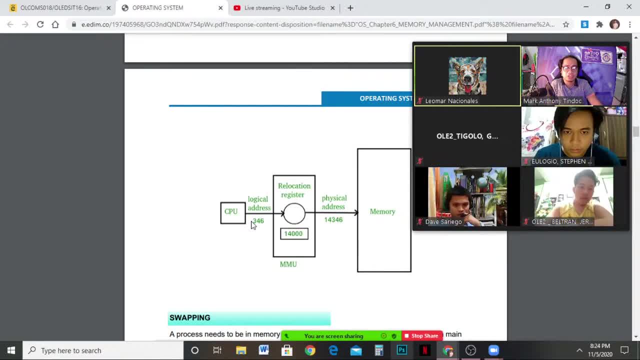 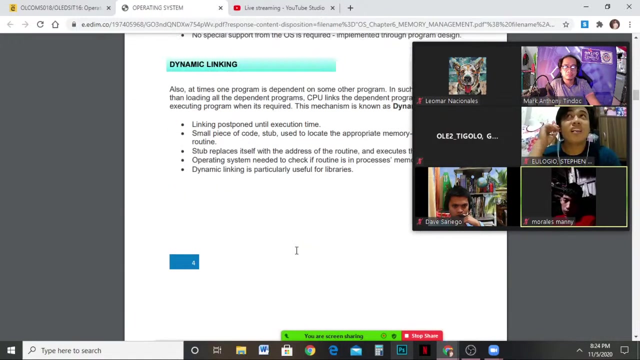 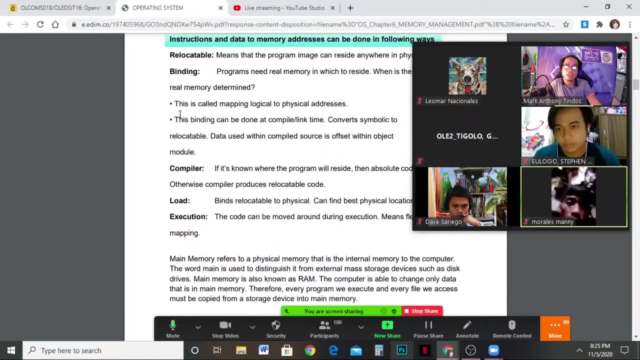 CPU. so register allocation. okay, register allocation- there it is provided by your CPU register allocation. then memory: get it. it will combine the allocation of physical address to logical address for it to be located here. okay, wait, next. this is what I explained earlier. this right from CPU. 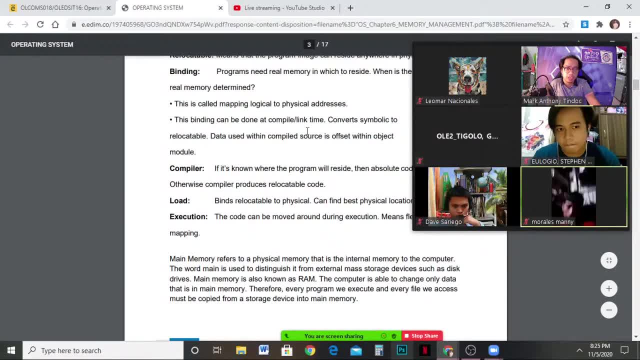 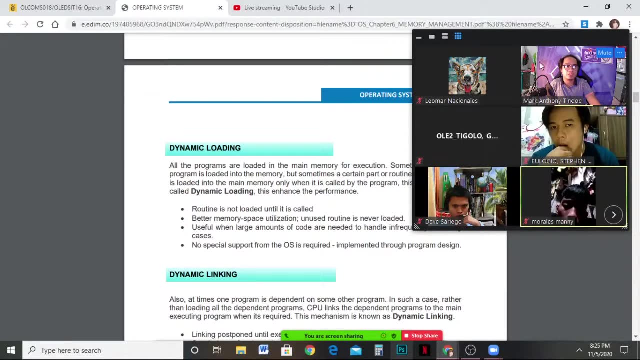 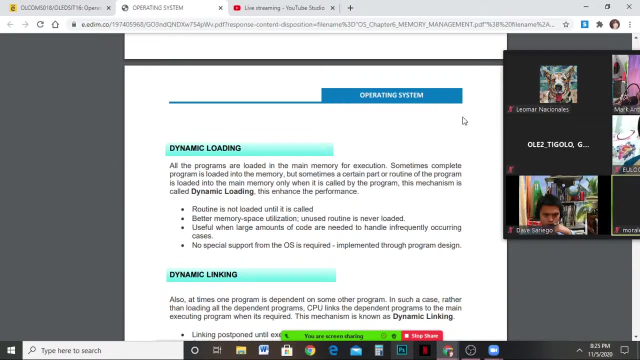 to compiler, then it will load, then memory to execute the program. what will happen now? if there is no memory, the program will not execute because there is no file. okay, so here we have what we call dynamic loading, dynamic and ah ah. dynamic linking and dynamic loading. what is the difference between? 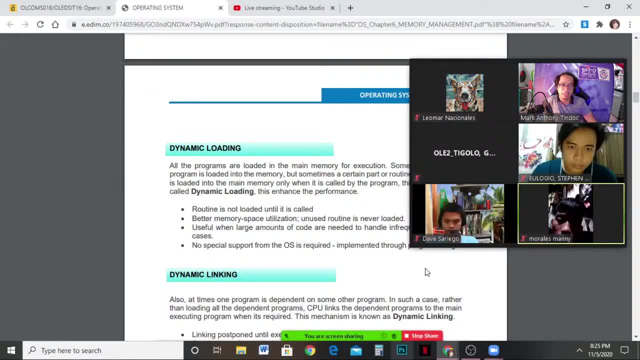 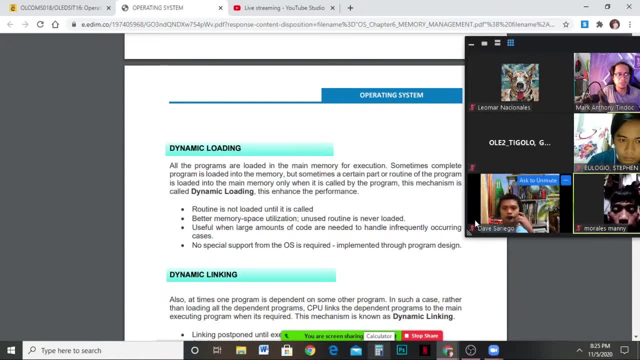 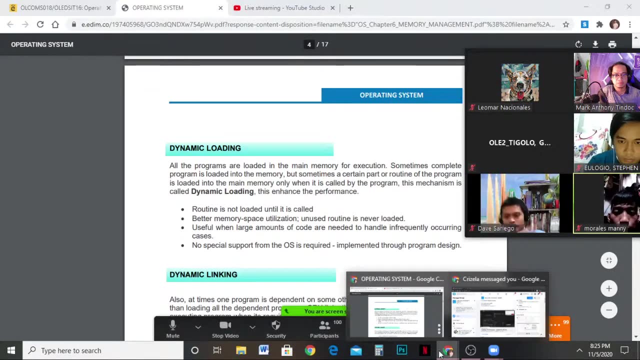 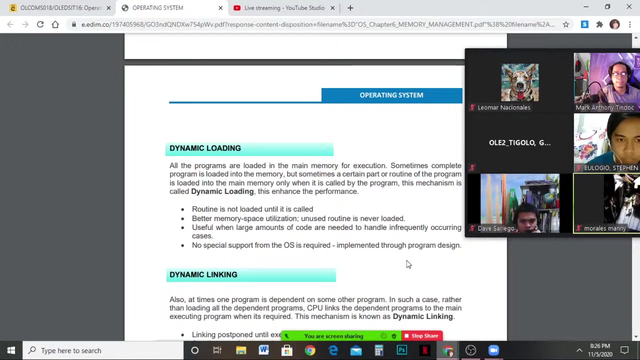 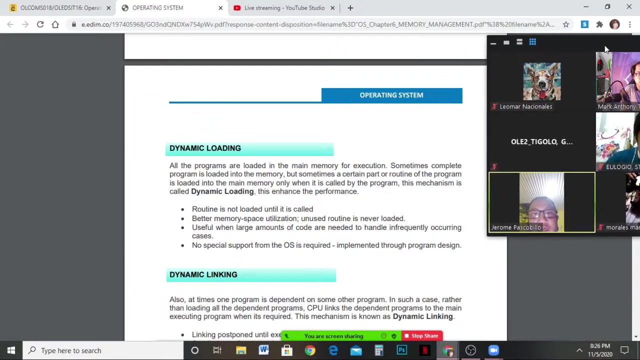 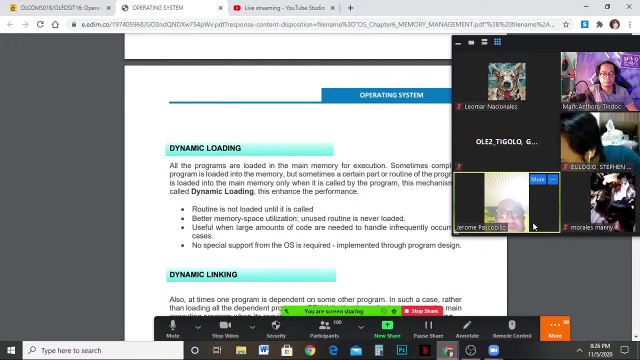 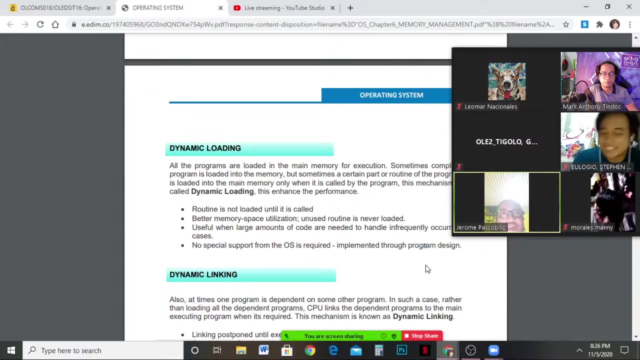 dynamic linking and dynamic loading. anyone dynamic linking and dynamic loading. So for my own opinion, this is the possible operation of a computer that is already in the operating system, While for dynamic linking, these are the things that were installed prior to the operating system, before it was executed. 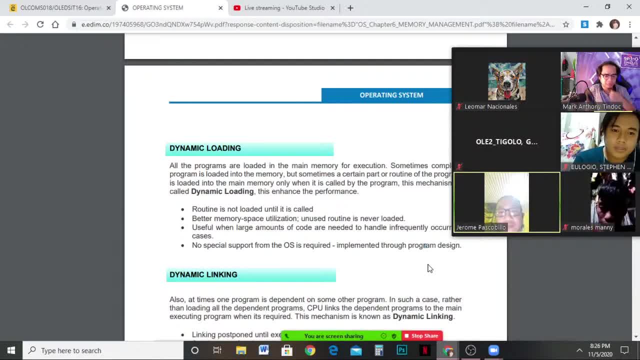 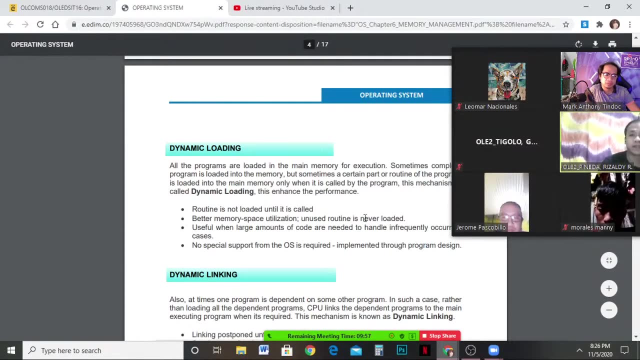 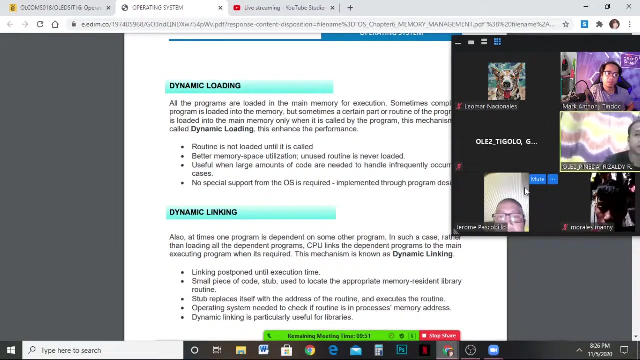 You know the answers right. It's a bit complicated, But the dynamic loading is correct. So the dynamic loading is correct. Okay, What else? What else Go ahead? Dynamic loading refers to mapping or left-open mapping, un-executable or deliberately into a person's memory search after it has started. 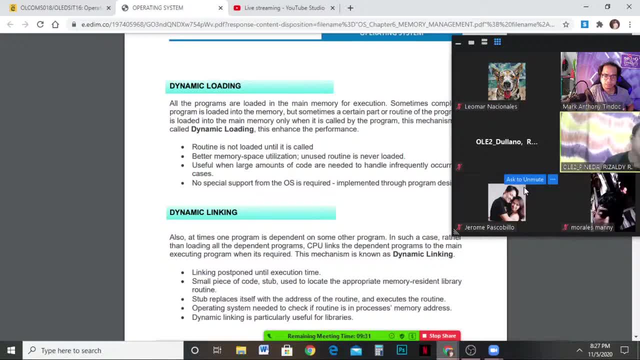 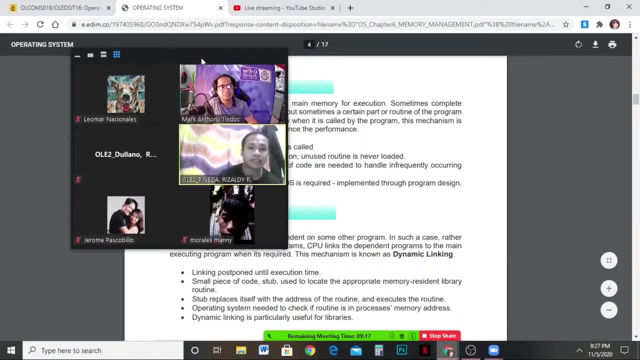 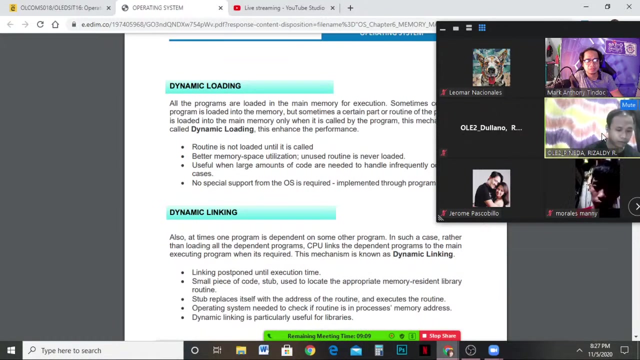 Then dynamic linking refers to resolving symbols associating their names with addresses or assets. Okay, I'm sorry, Kyle, I'm happy. Okay, He's happy. Okay, I'm sorry. Okay, I'll just make an award here to the post you posted. 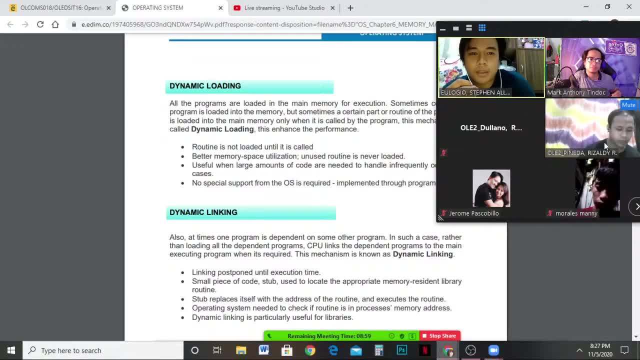 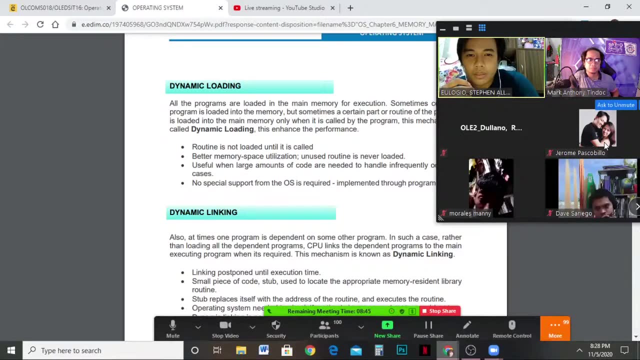 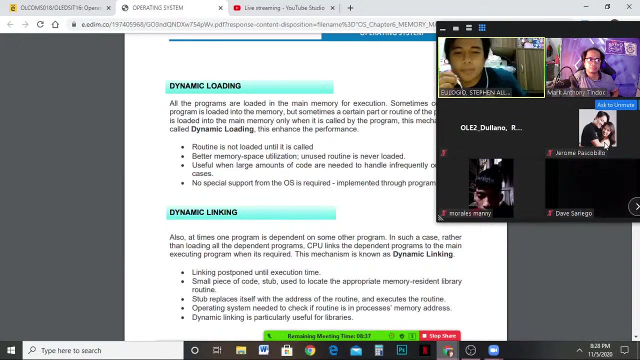 What I understood is that when it comes to dynamic loading, they say that all programs, It just loads in the memory for execution and then then the dynamic linking is a program that depends on other programs. So it's not directly to the CPU. The CPU's not giving it to you. 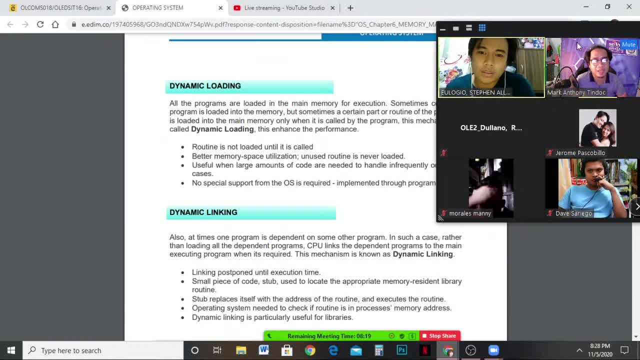 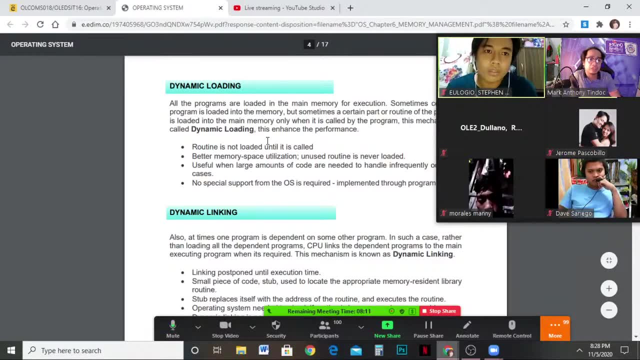 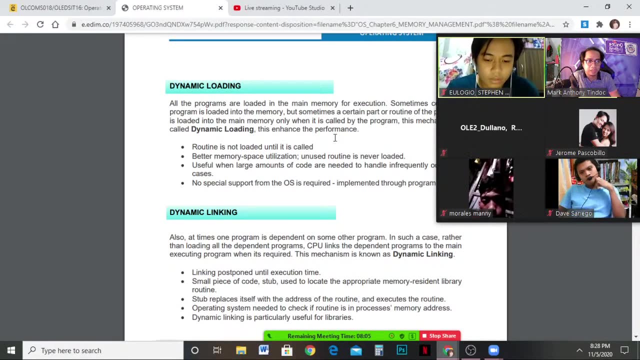 So that's the, according to the reading here. Okay, aside from reading it, I'll give you one more information: The dynamic loading I know I mentioned earlier. I don't know if he really knows that or he read it on google, but the dynamic loading coming from, uh memory. 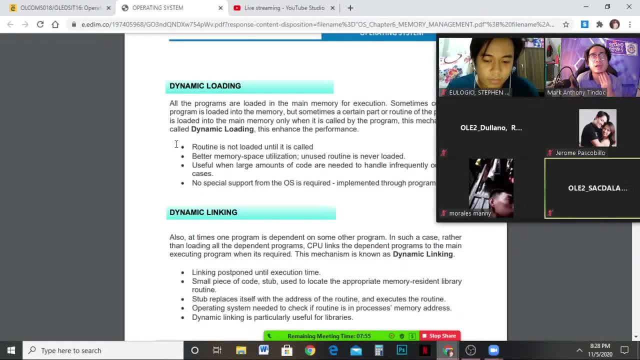 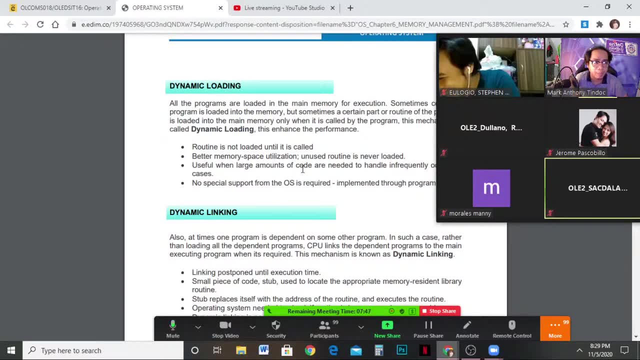 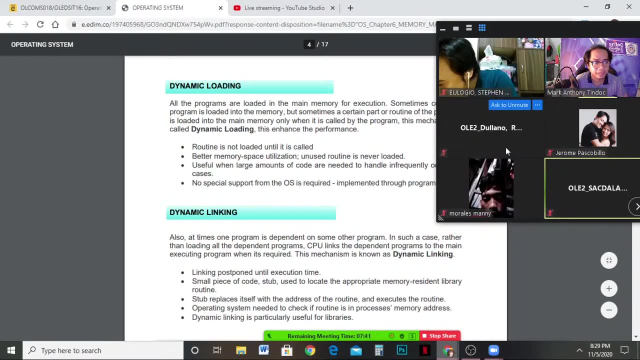 so it's like before you execute a program. what happens before you execute a program? right, we have what we call a compiler, then loader, then execution. so where does that file get? in our memory? so, the dynamic loading: directly in your main memory. you will load everything in the program that you want to execute, okay, but not necessarily everything, just what you need. 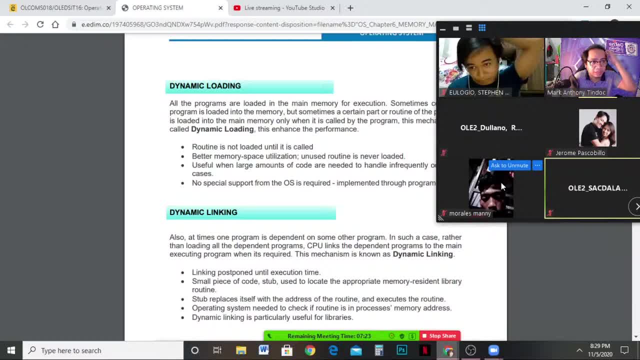 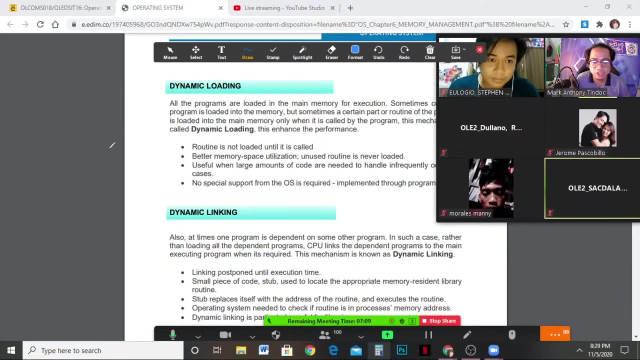 now, what is the difference between? what is the difference? this is because this is what, uh, dynamic linking is just a link, to say, the ones like this drawing again. so let's give it one more. look at this and go back to the drawing. for example, you want to understand my drawing. 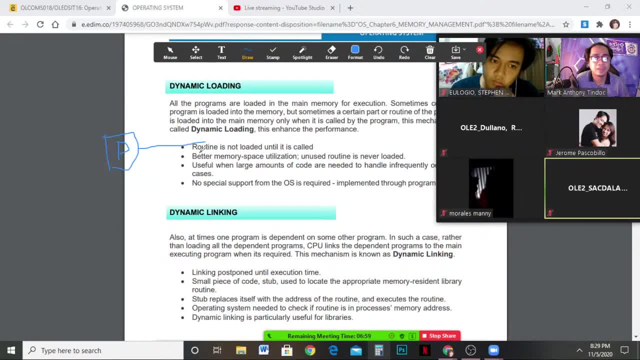 so this example: here we have an executed program, so copy, and then what happens here is that with dynamic linking we have a compiler, assembler- remember the compiler and assembler. right from our um, uh, call it in our programs, our programming language, right, we have assembler and then assembler. so you can't do that in. 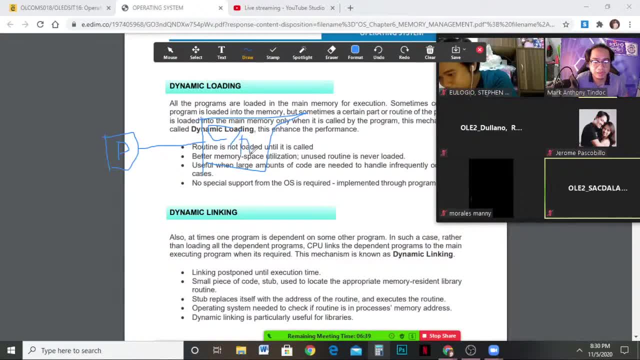 compiling or you can't do it in another language. the compiler has assembler, and then where the storage is located, it's in the program name's. where you can't find it here, you can't find it: compiler, assembler. this is where the link will come from. it means that before it can be executed, 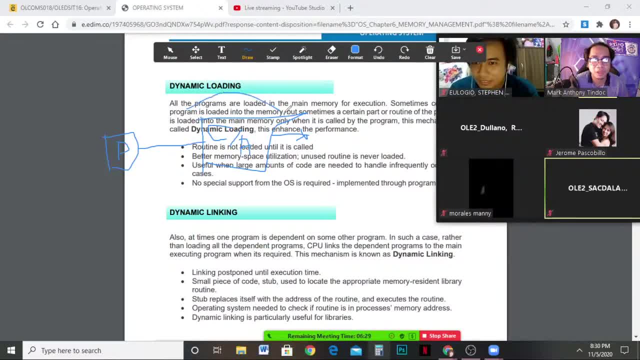 it will combine first. it will combine first before it can be executed then here in the main memory. it means this: loading: before it loads, it will get a link. before it loads, it will get a link. it means that this dynamic loading and dynamic linking. 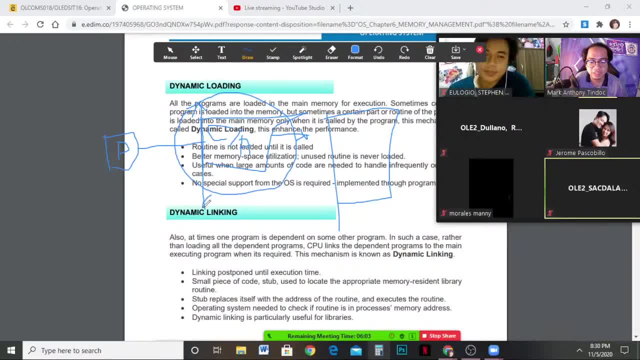 is connected to each other. what is the purpose of these two? to execute a program. what they are doing is: they need to execute the program, they need a link, they need to load now. this is because they need to load. this is because this dynamic linking 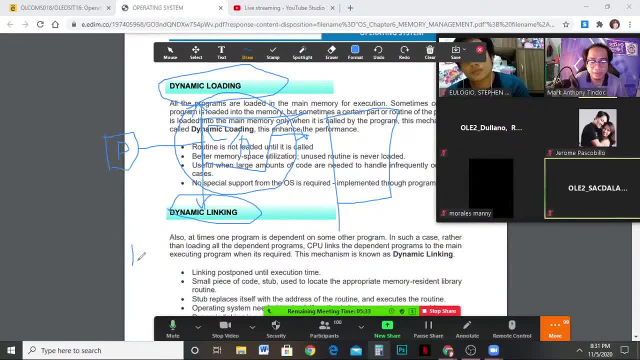 it means that it is dependent. it has step 1, step 2, step 3, step 4. it means that before you can go to step 1, it needs to be executed. it means that before it can go there, it needs to be done. 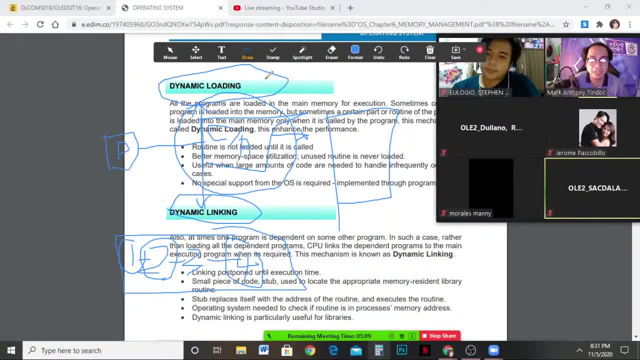 it needs to be done. it needs to be done the program, because this right here is on our memory. it means that you can use this directly on your memory to execute, to execute, you know to execute it. you can run it on your memory, you can load it directly. 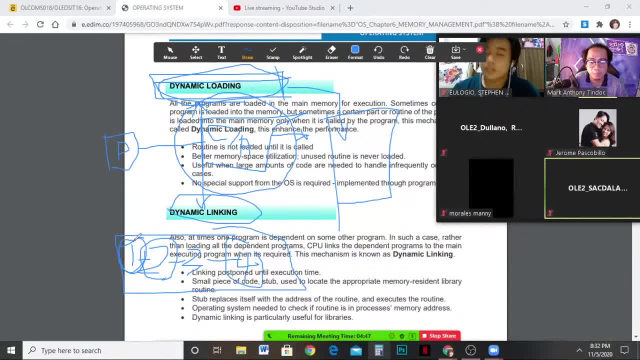 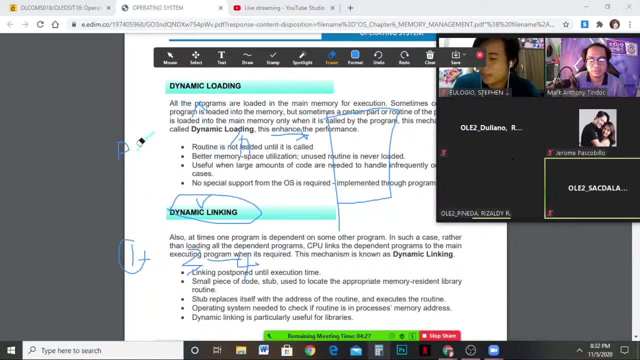 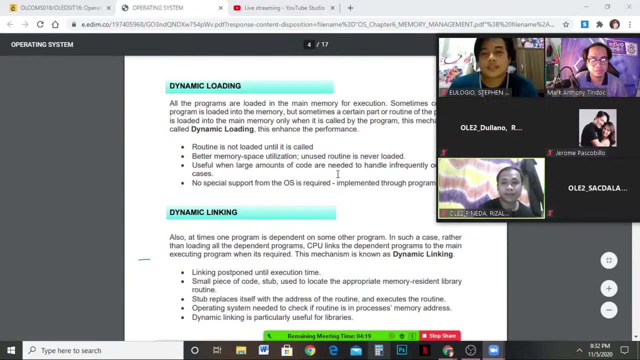 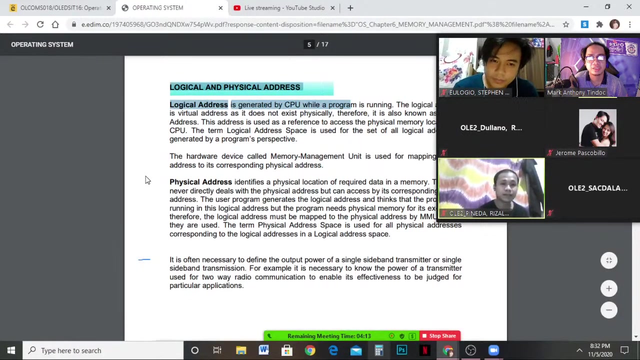 because this is provided, it will compile, it will provide ito, mapo-provide ito ng assembler mo. Okay, Question, Wala diba, Wala Ito natin ando Next, Ito pala napag-usapan, na pala natin kanina eh. Physical tsaka logical address, Physical Ito pala nakasulat eh oh. 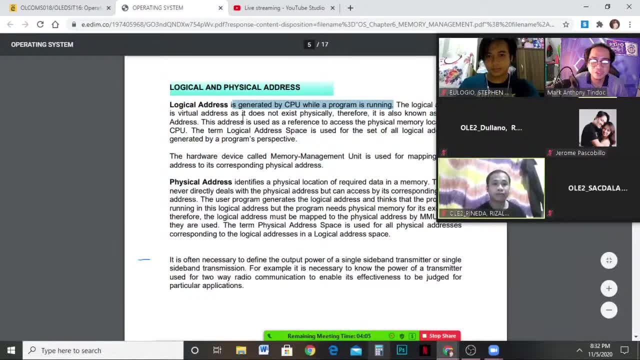 Ah, binasa mo lang ito, Mina, sino yung nagbasa Ayun: oh, Generated by CPU program running Identifies physical location of required data. So tama, Tama nga yun Usapan natin kanina diba. 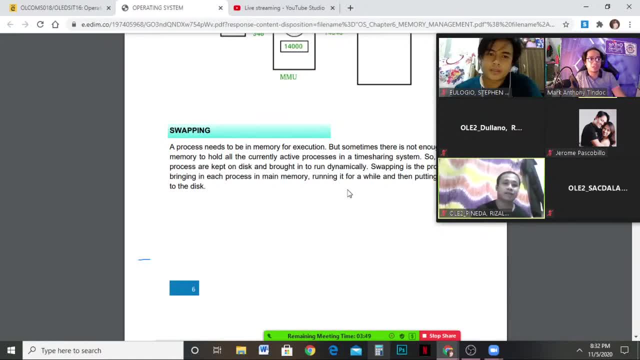 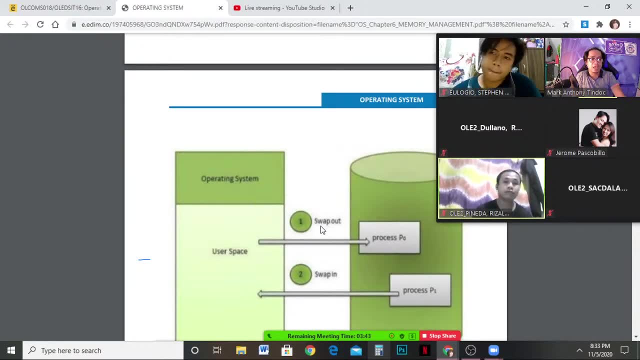 So swapping, Swapping, Ito naman swapping. Ito yung binanggit ko, kanina Yung. swapping may kinalaman to sa main memory tsaka sa secondary memory mo, Kasi hindi naman lahat kasha sa main memory mo, So kailangan mo ng backup memory. 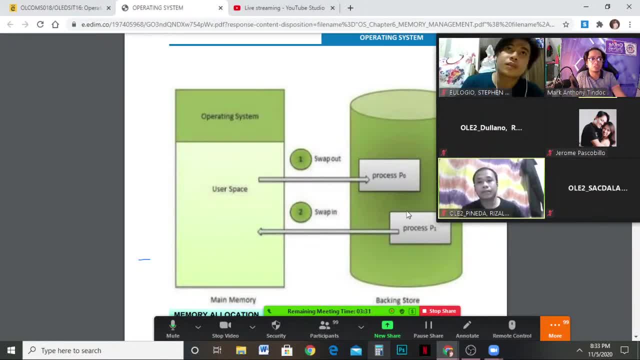 Ang nangyayari. ito yung allocation tsaka deallocation. So pag gagamitin mo kukuha ka Swap in, Tapos, pag hindi mo nagagamitin swap out, Yun lang yun Swap in, swap out. Yun yung swapping natin, Yun yung tinatawag natin yung swapping. 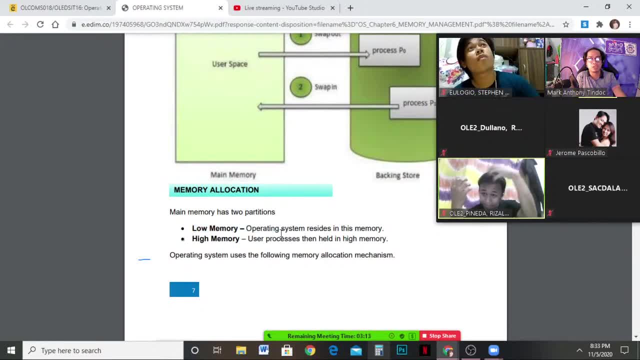 Sa memory allocation meron low memory tsaka may. high memory Operating system reside in the main memory, So that is low memory, Pag hindi nakaya. high memory. User processes data then held in high memory. operating system uses the following memory allocation mechanism: 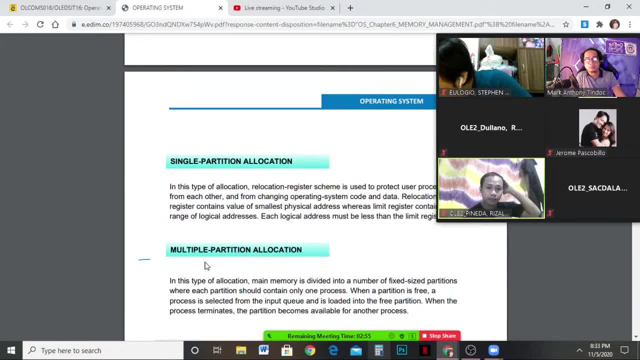 single partition allocation, um, multiple partition allocation and contagious memory allocation- actually the whole memory system you will use- means you will use the whole main memory. example: your memory is four gig. okay, your executable program is one mb. that is full capacity to say what will happen. we can no longer enter another. 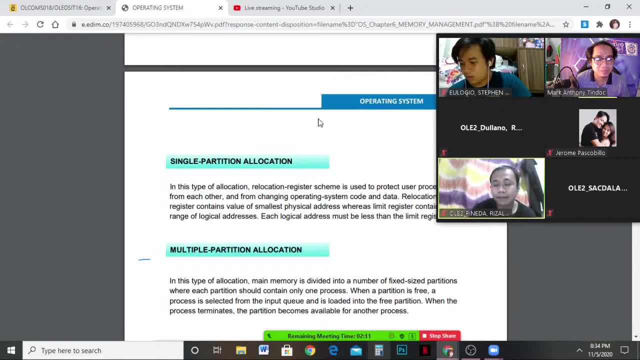 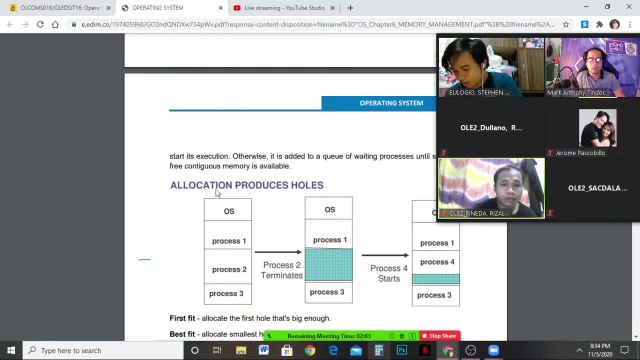 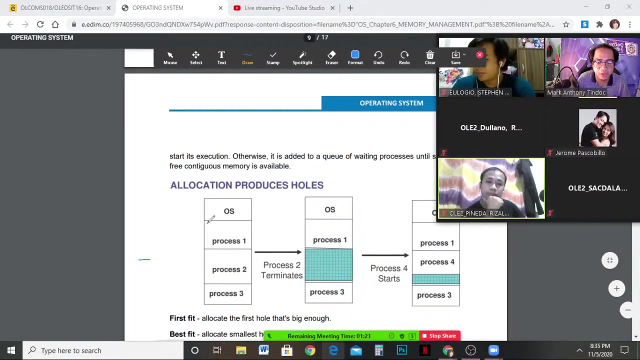 executable program. okay means I hope there is something here like this and okay. okay now multiple dynamic dynamic allocation: um drawing. here. it's dynamic, dynamic, suitable example. this is a bit small. this is where it will go get it. it will choose the smallest. okay, then, if it's a bit big, it will enter here. 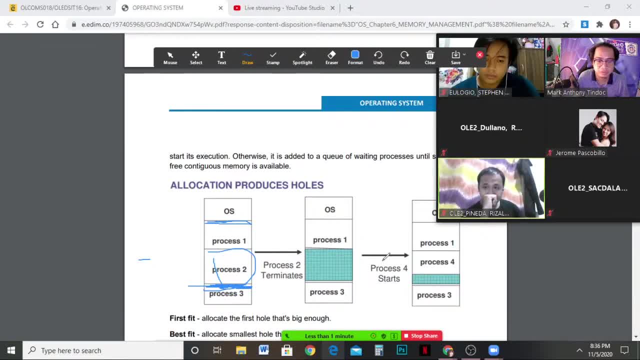 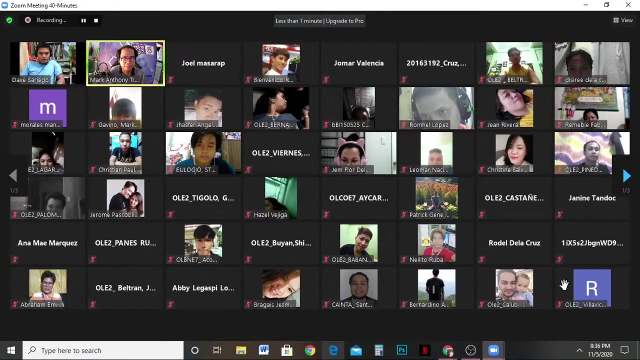 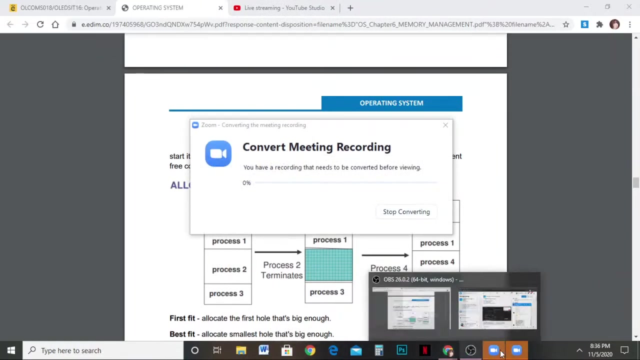 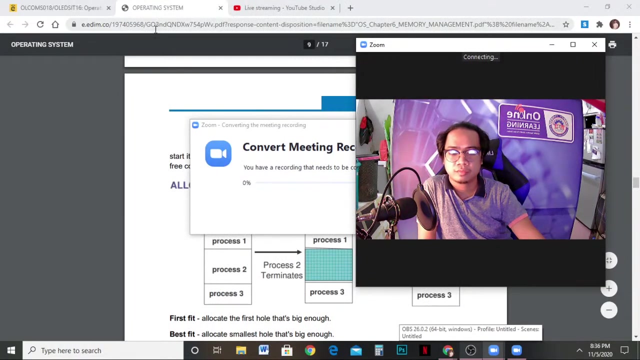 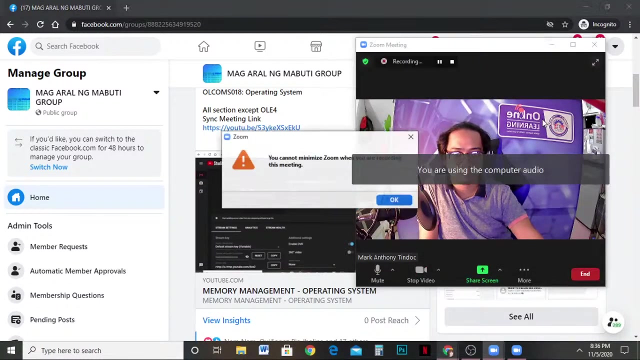 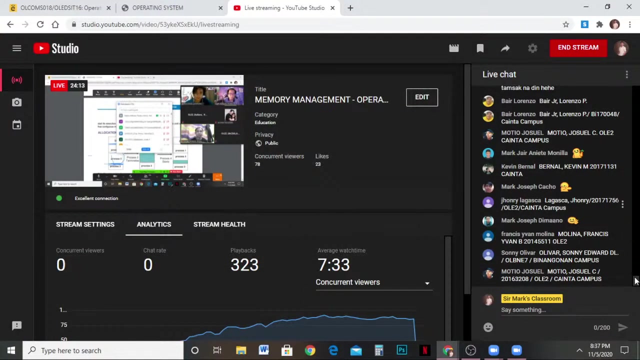 that is dynamic allocation, so there are different terms. this is going to be timed. enter again. did you attend? did you attend? yes, sir, let's stop sharing it's time. I'll end it and enter again. press enter: it's failures, it's failures, I suggest, sir. 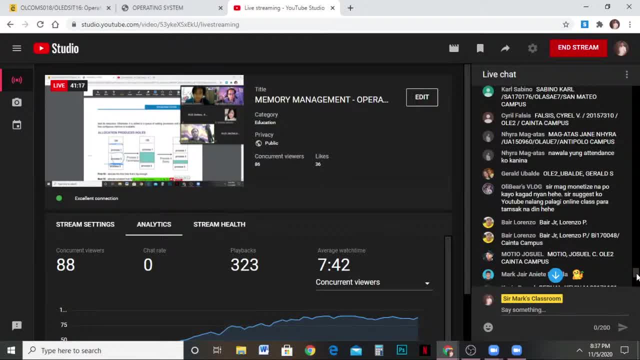 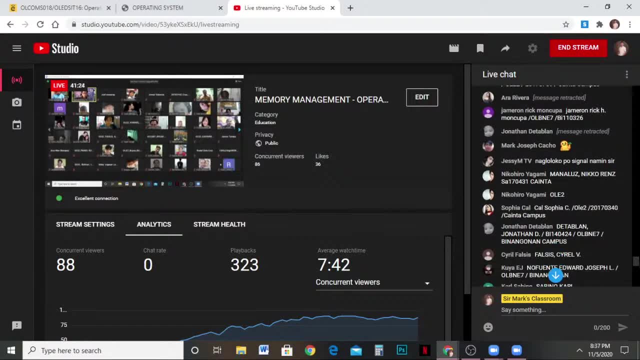 you should be able to monetize right now. I suggest you to only use YouTube. I suggest you to only use YouTube. I suggest you to only use YouTube lang, palagi online para tamsak monetize. ayun nga no monetize na, ah, dahil dyan binanggit mo yung. 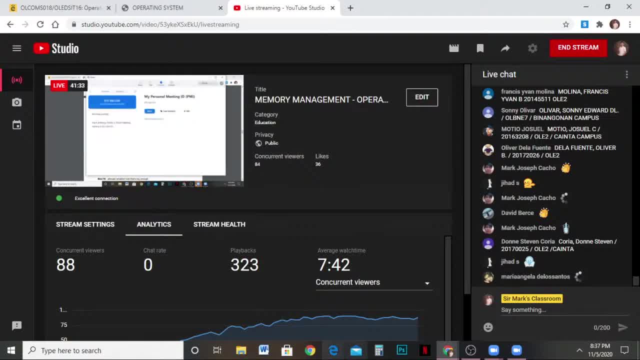 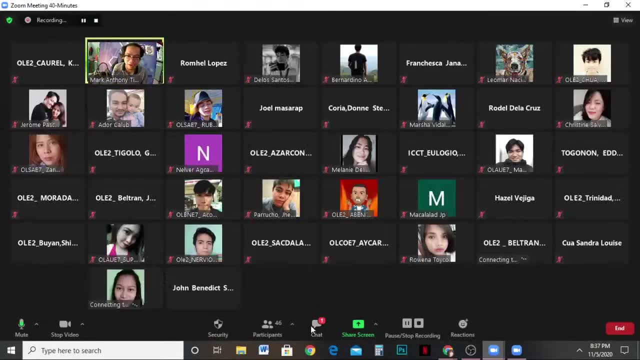 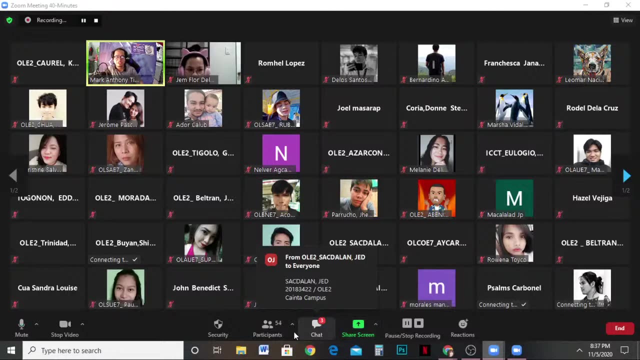 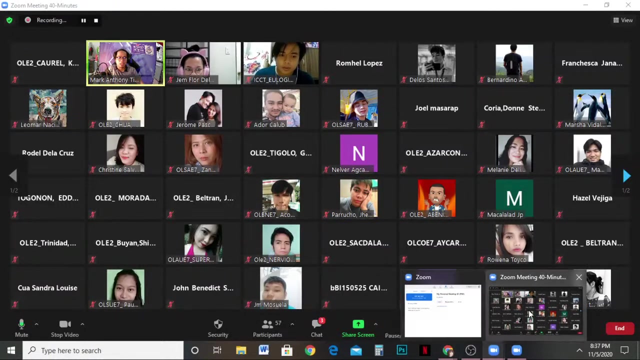 monetize, baka naman subscribe. subscribe din kayo nagbanggit ng monetize, subscribe nyo yan. kailangan ko ng 1000 subscriber para bayaran to subscribe and like and share the channel, kaya hindi ko naisip na mga monetize malabo eh 4000, eh, 4000 na. anyway, going back, balik tayo. 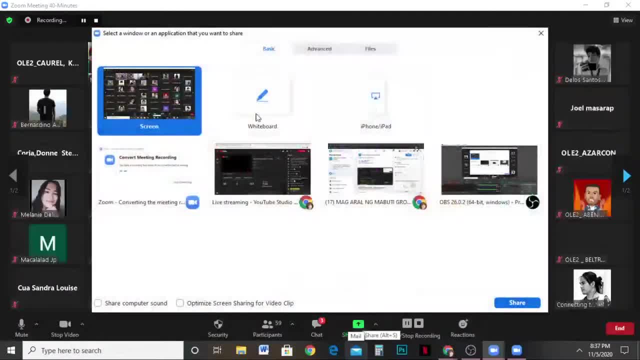 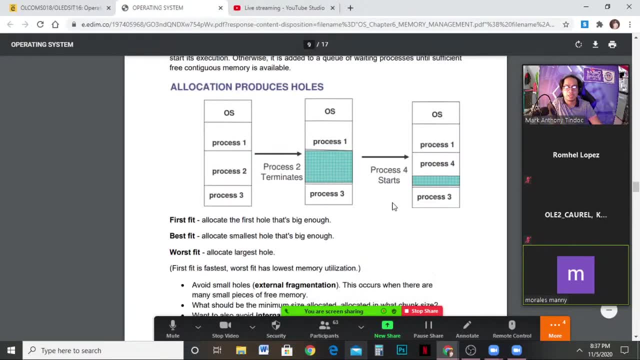 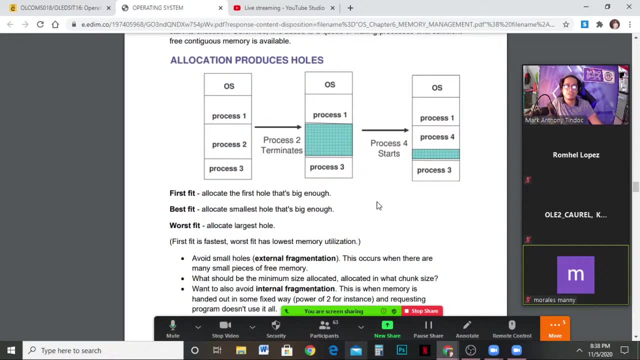 baka na yung mga monetize, monetize na yan hindi na, kapag nakapag attendance ka na, okay ka na. ah, ito yan dito, tayo na huli diba. ah iba tawag ngayon dito nung unang panahon, kasi ganun tawag sa amin eh. 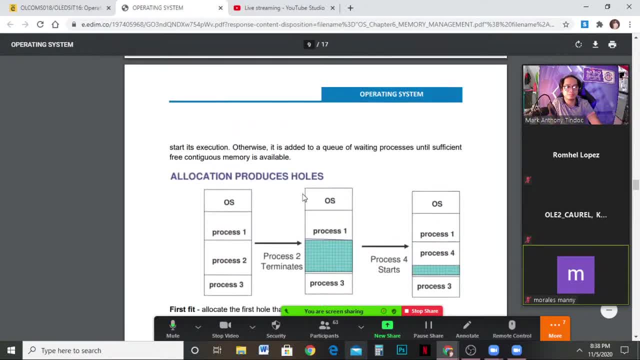 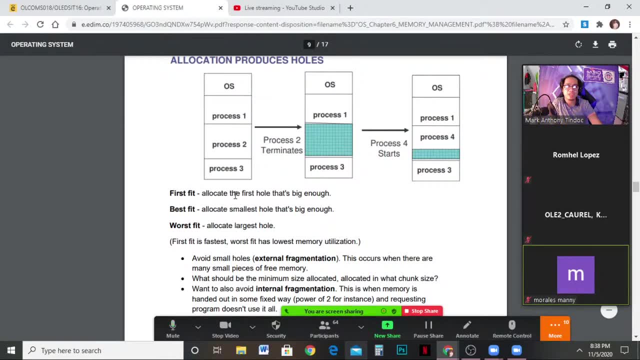 ah, ito pala yung, ito yung ano correct term yung ginagamit natin. first fit, yung pinapaliwanag ko sa inyo kanina. first fit: allocate the first hole, that's big enough. best fit: allocate smallest hole, that's big enough. 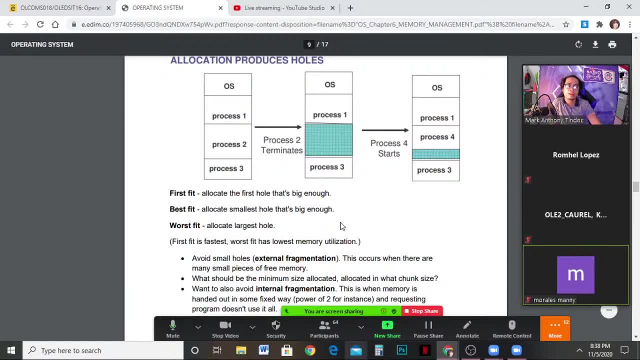 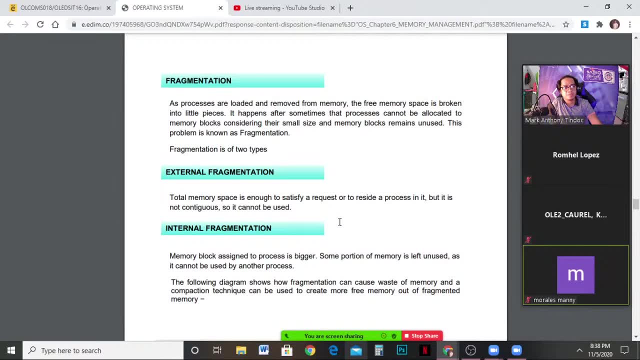 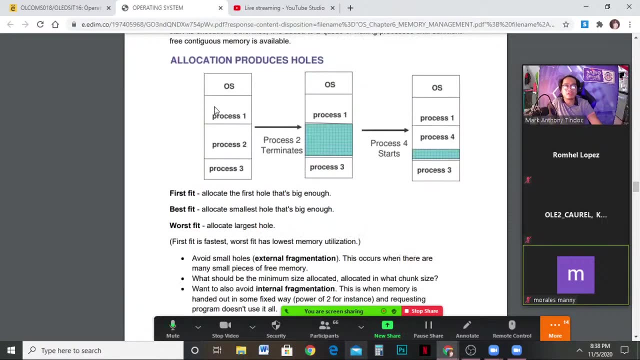 and worst fit, allocate the largest hole. okay, augmentation, ah, ito na ito yung pinakabago fragmentation. so pinapragment na natin, kasi diba dati kaya kunyari maliit, dati maliit, pagkakasahin dito. 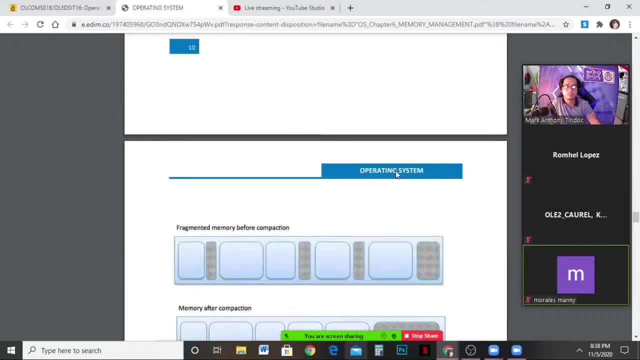 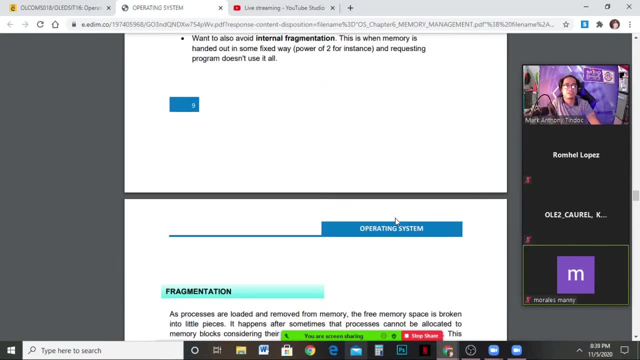 ayun, pwede ka na magpragmentation tapos na pala tayo. ayun, ah, pagkakasahin muna kasi may mga parang. ah okay, fragmentation is a process. ah as process are loaded and removed from memory. the free memory space is broken. 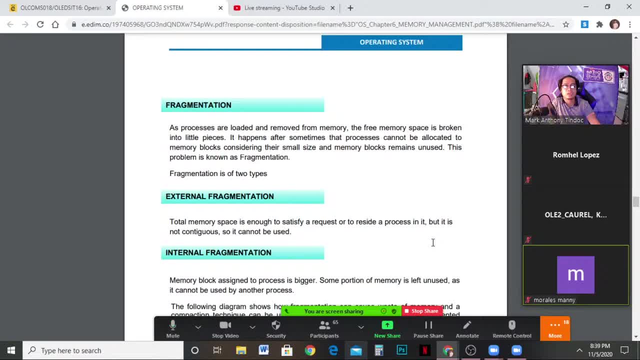 ah, as process are loaded and removed from memory, the free memory space is broken into little pieces. it happens after. sometimes that process cannot be allocated to memory blocks, considering their small sizes, and memory back remains unused. this problem is known as fragmentation. meron dalang klase ng fragmentation. 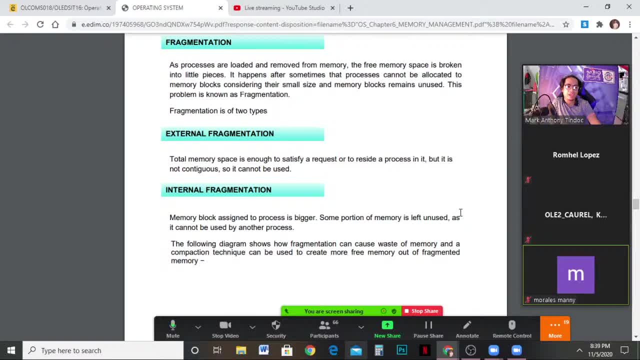 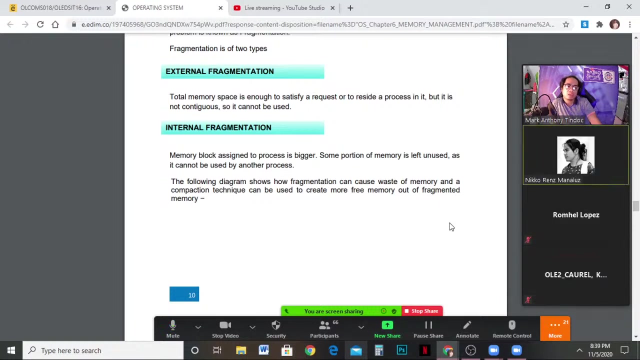 external fragmentation and internal fragmentation. external fragmentation: total memory space is enough to satisfy a request or reside a process in it, but it is not contagious so it cannot be used. ah, internal memory: memory block assigned to process is bigger. some portion of memory is left unused as cannot be. 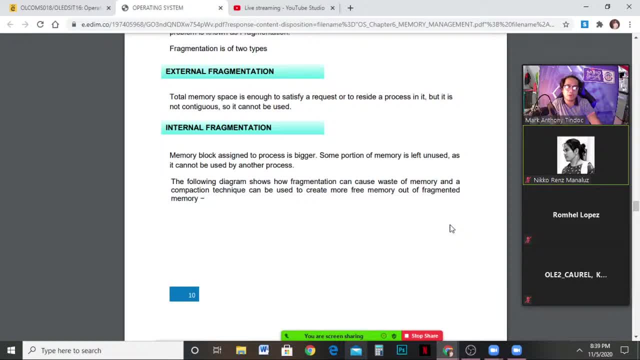 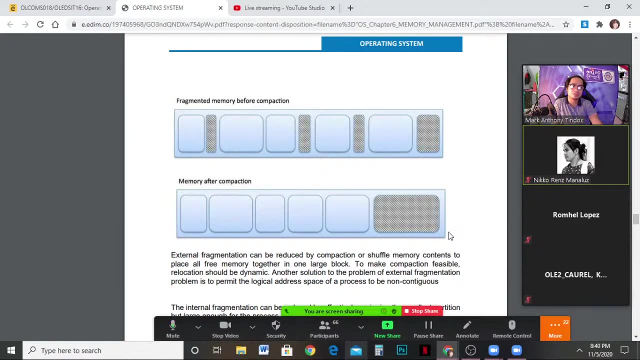 ah used by another process. the following diagram shows how fragmentation can cause waste of memory and compaction technique can be used to create more free memory out of fragmented memory. what is it called here? what is it called here? we are deleting cache memory. what do you remember? 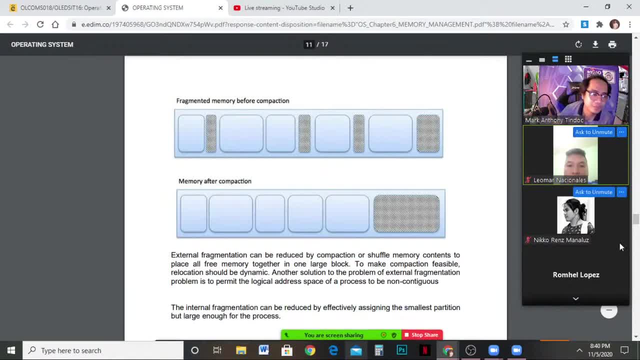 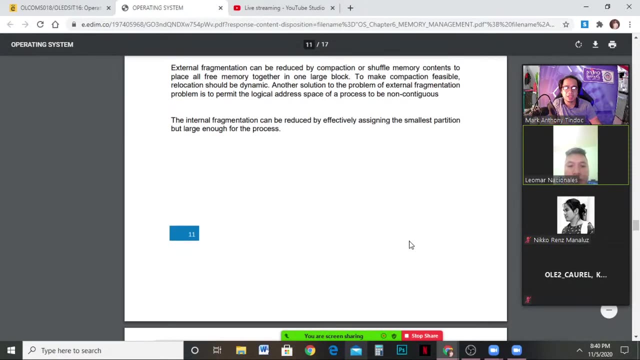 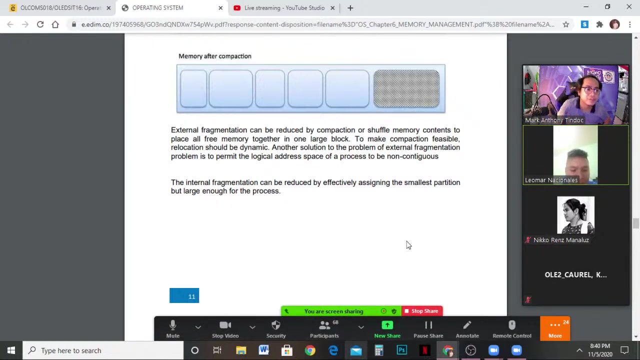 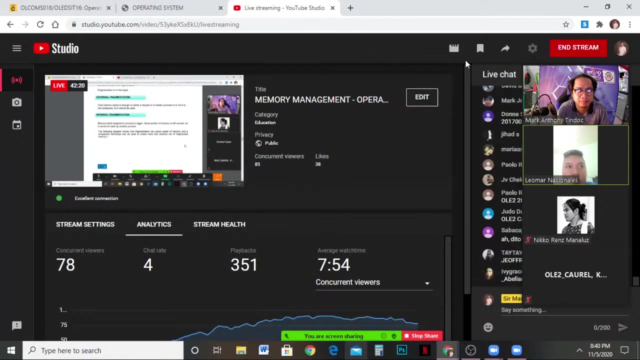 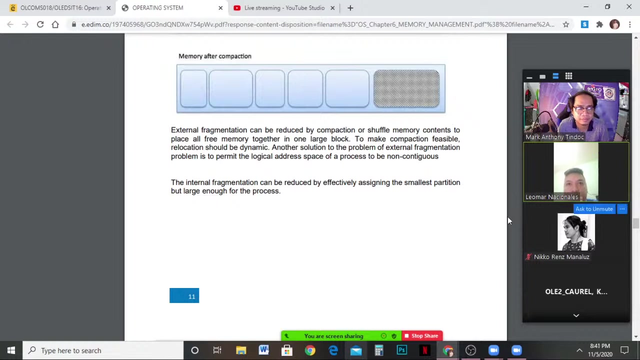 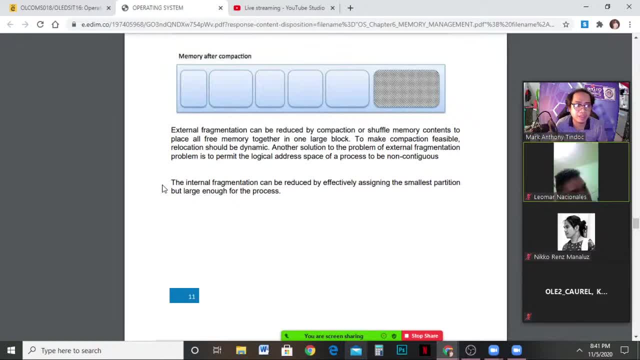 we have our main memory. it goes to the files we process, it goes to the cache memory. it also has a memory. our processor has a memory. so that's what we're sending to process now. if it's not processed, if it's not processed, that's what's left. 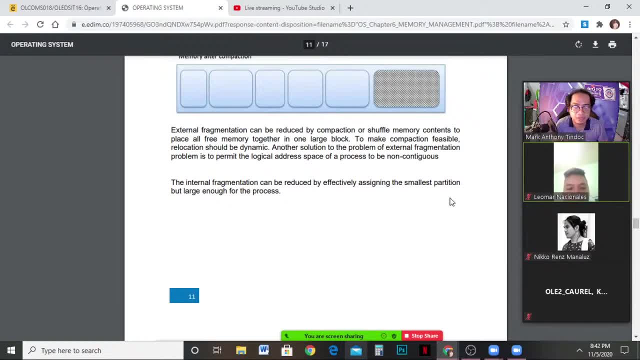 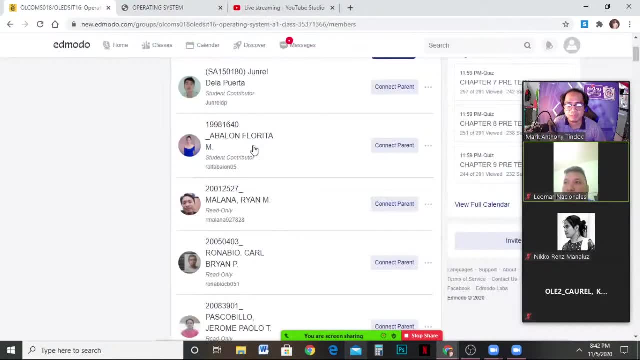 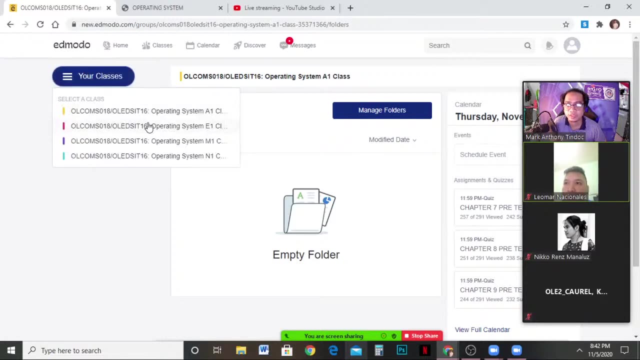 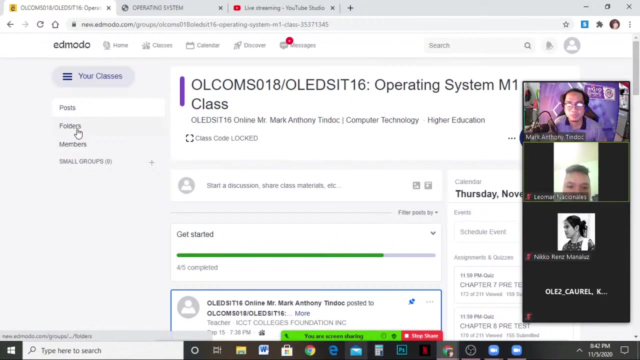 for fragment. that is your cache memory. okay, anyway, this is just up to there. our next topic is all about. where are we going to? topic next: empty. can you see this? I have a question. I mean: can you see this folder? are you looking at these folders? 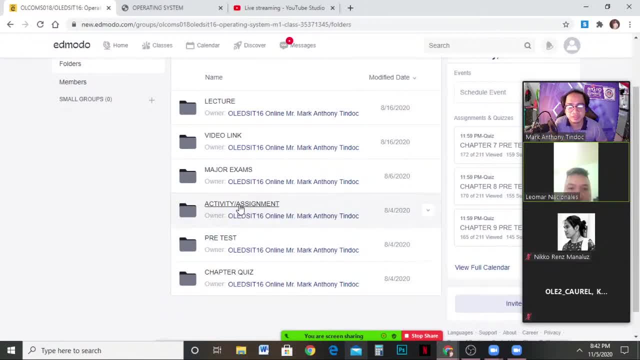 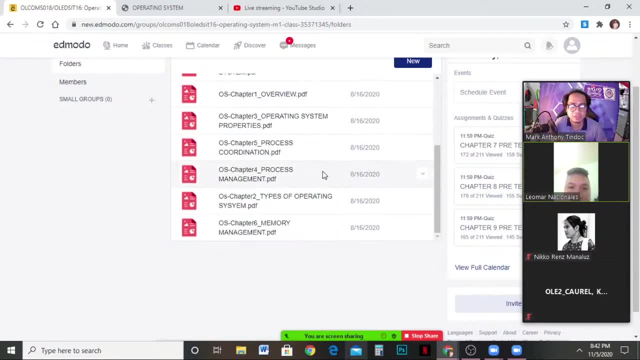 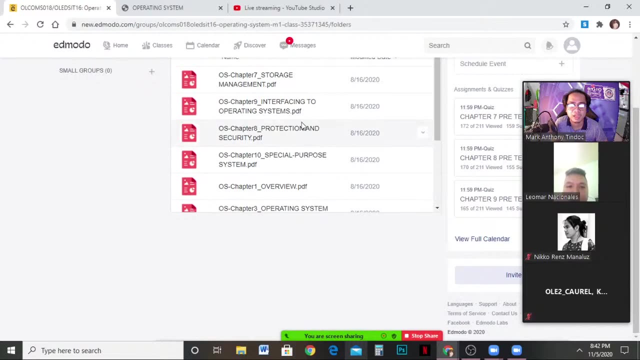 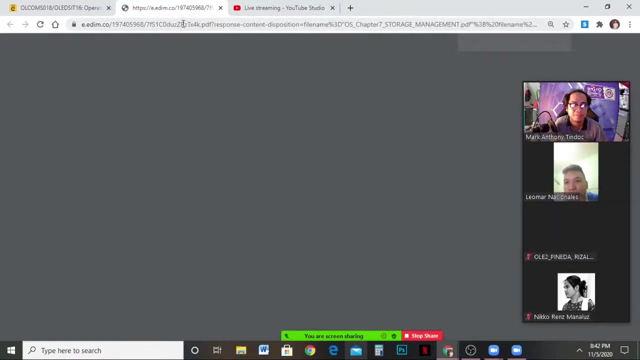 this is open to you. all of them are there. your exam is there. you can check it. it's not like that, sir. maybe it's just for me. okay, folders. no, that's why it's just segregated. maybe it's just for me, it's just for me. 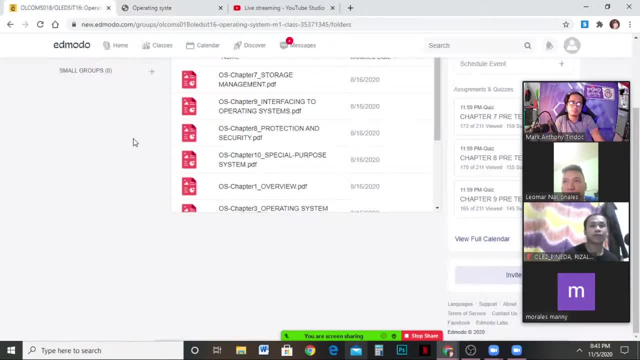 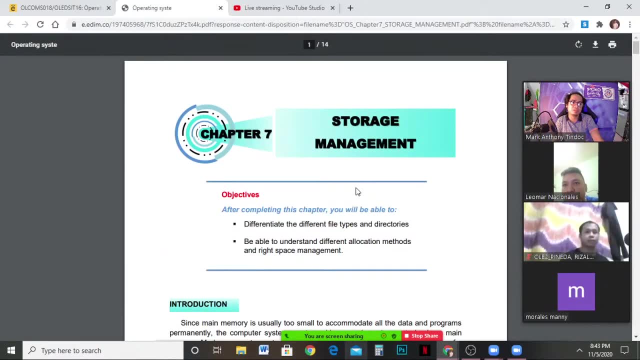 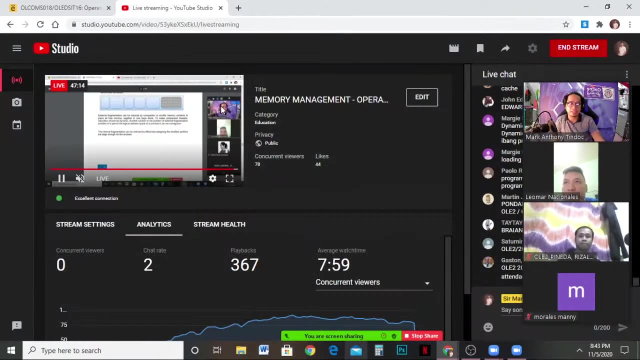 it's hiding from us. I forgot to hide it. it's just for me. I don't need to hide it. our next topic is all about storage management. do you know what we're talking about these management management about what? about what? about what? 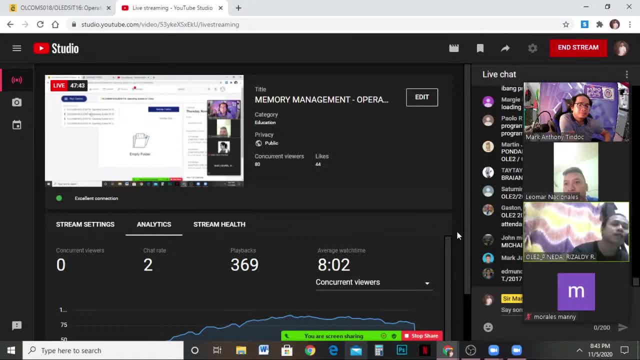 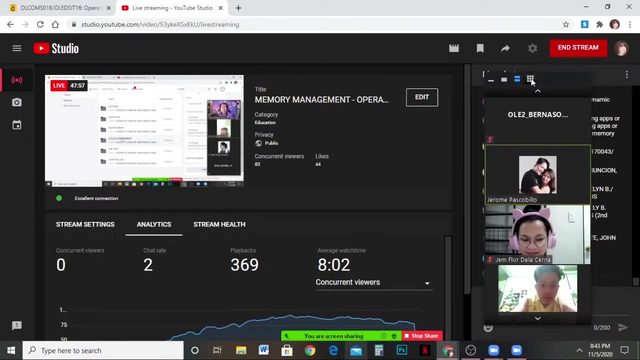 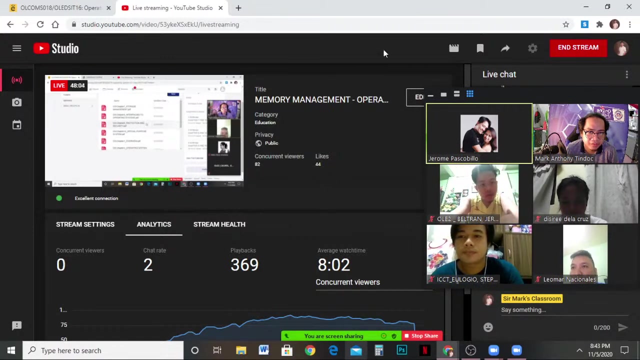 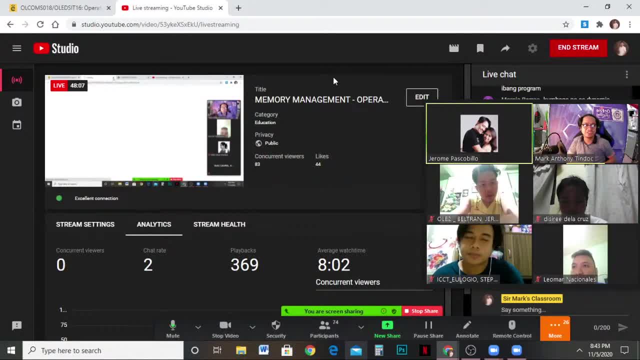 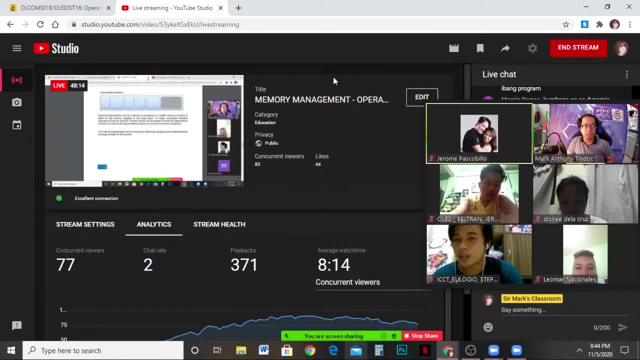 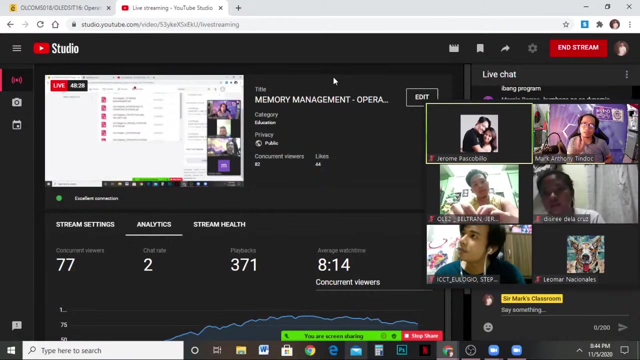 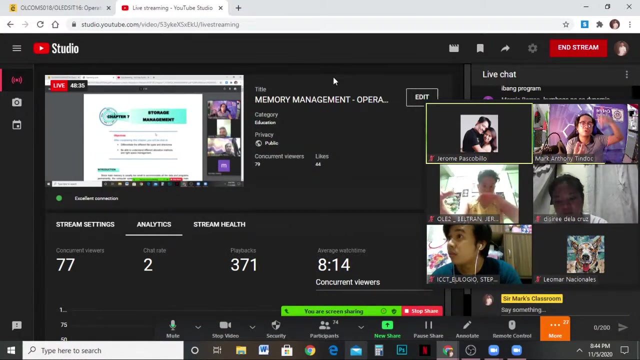 okay, actually it is the function of the operating system. this is the power of the operating system: file management, memory management, process management, task management, all of that. this is the function of your operating system. do you remember our operating system is? it communicates from your hardware to our software. 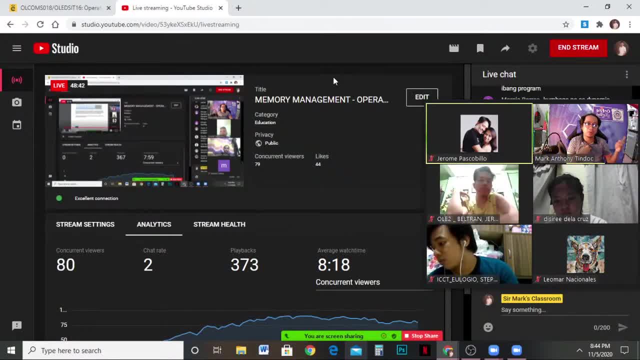 until it reaches our user. it also communicates from one hardware to another hardware. it can't communicate the two hardware without the software, which is the system software that we call, and one type of the system software is the operating system. it's like this for you to understand. 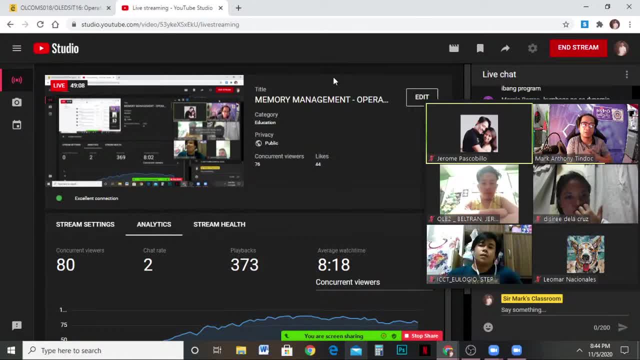 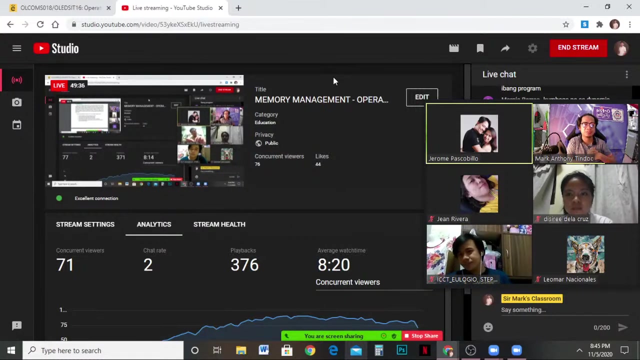 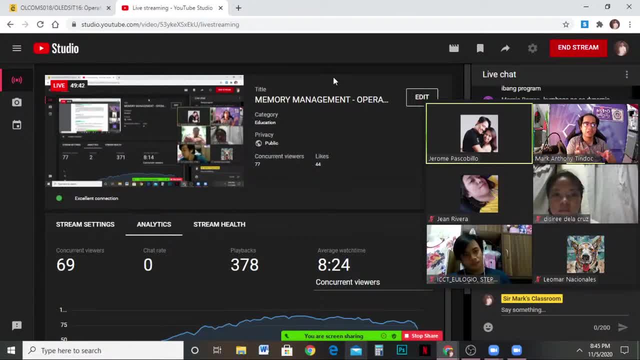 your hardware, your computer. they don't understand your printer. so how can they understand? you need drivers and that is one of the systems. that is one of the system software. it's one type of system software. our operating system is the same. one type of system software is operating system. 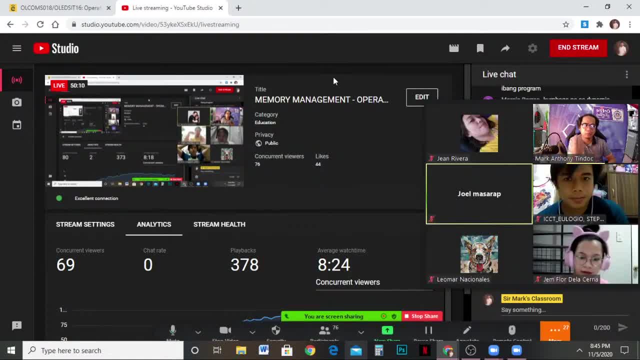 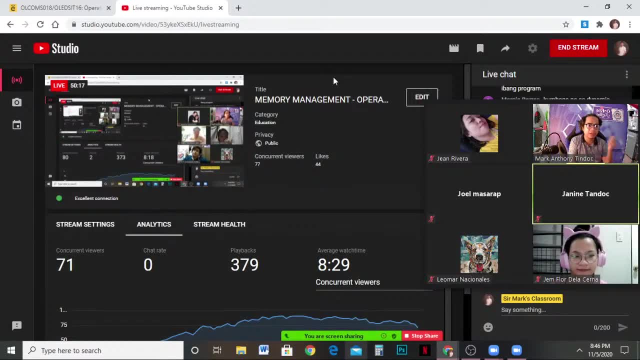 our operating system so that they can communicate to each other. your memory, your processor, needs an operating system. your output devices needs an operating system. so what we are talking about, what we are talking about is all about the operating system, how it functions, what it does on the computer. 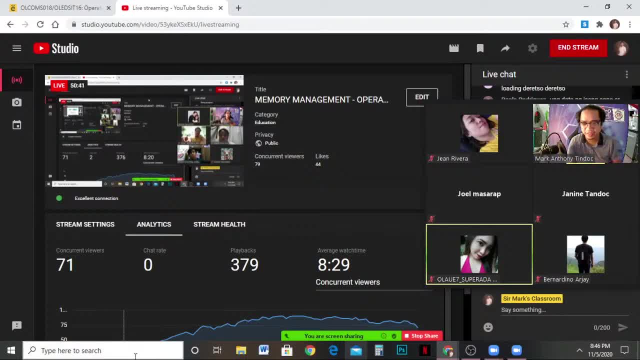 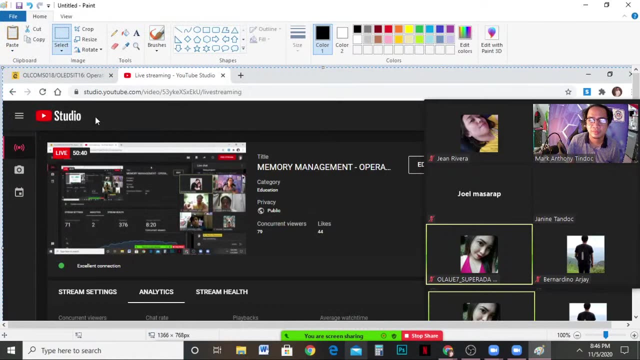 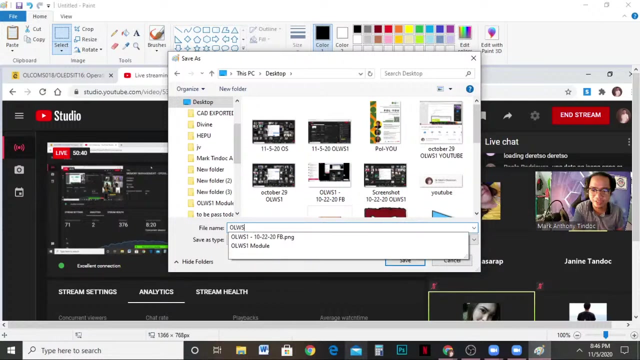 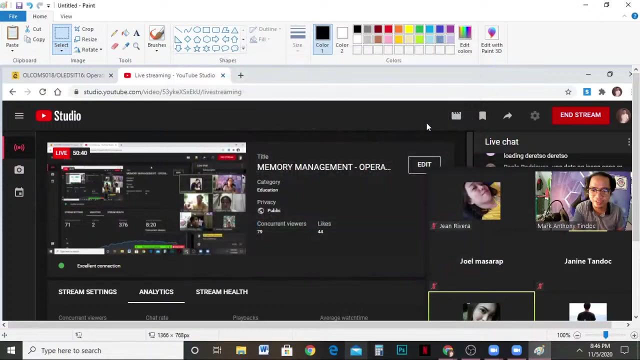 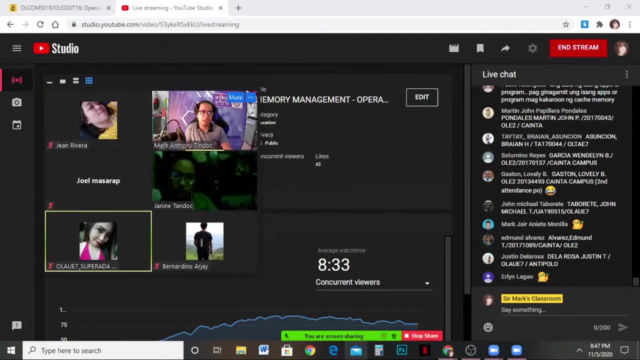 explain my logo. i will print out this a few screen screen i will pass him. okay, okay, question, no question. Talang, talang, Talang, talang. Wait a sec, We're out of YouTube. No attendance, Sir. it's a mess. 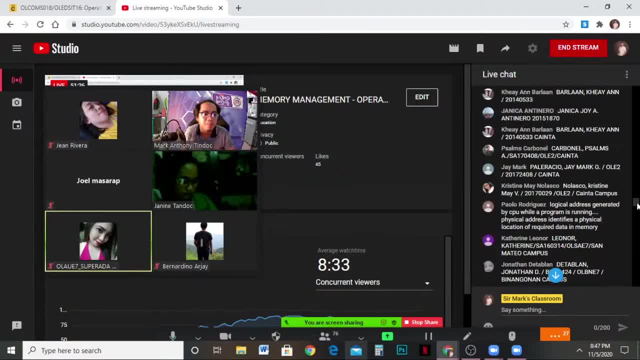 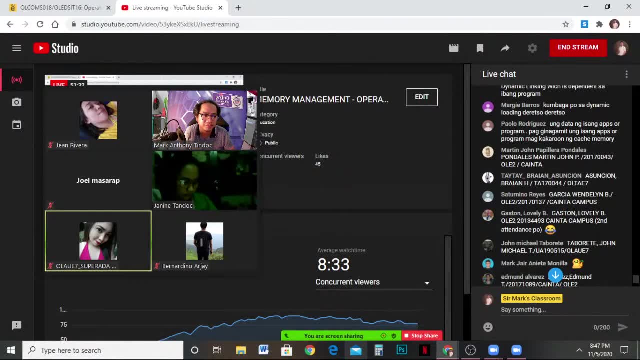 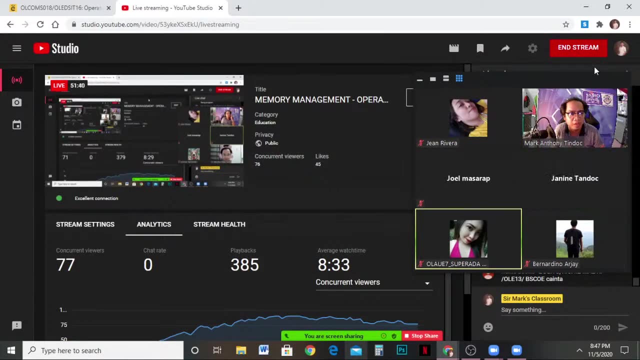 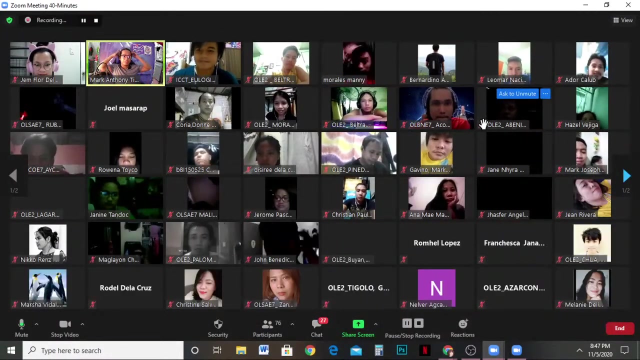 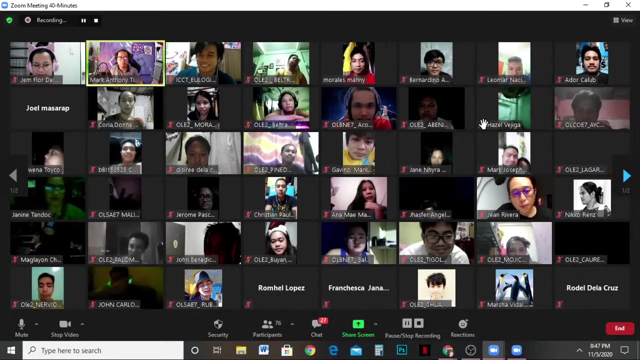 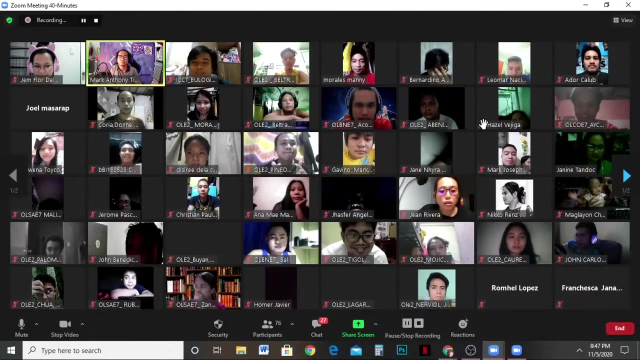 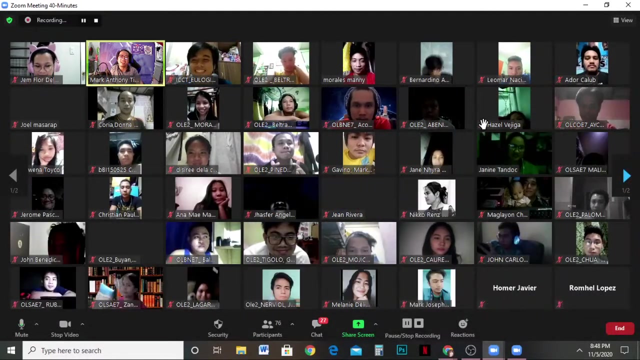 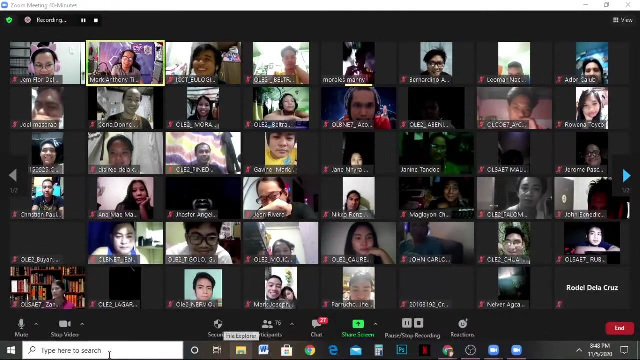 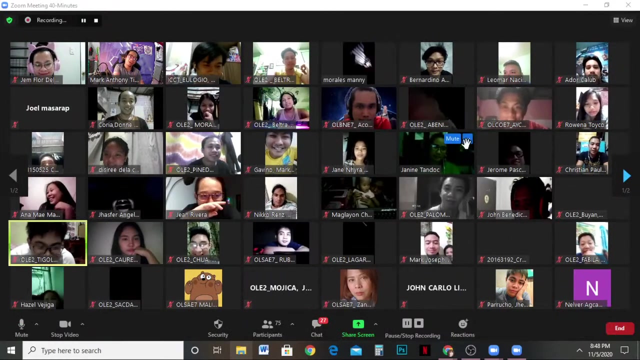 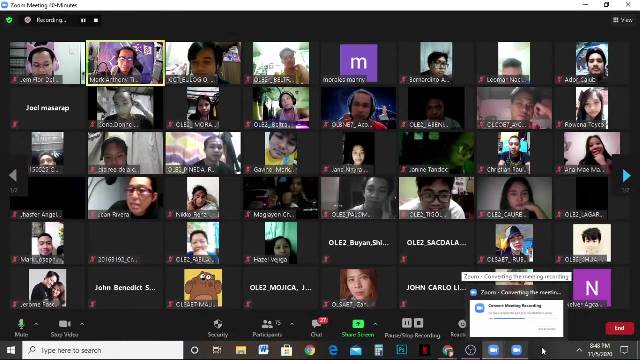 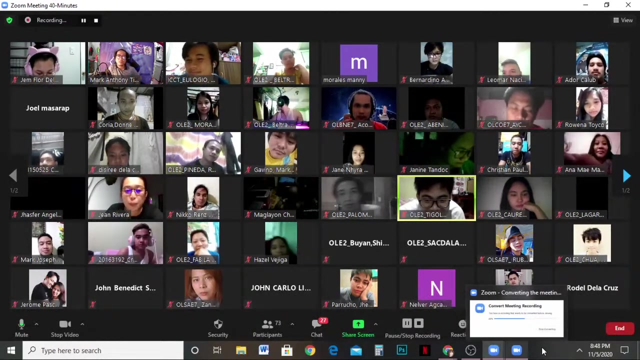 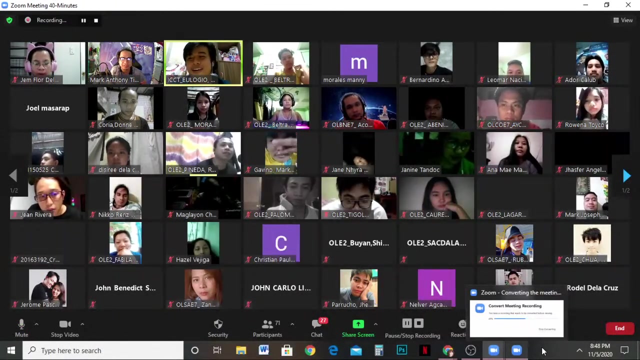 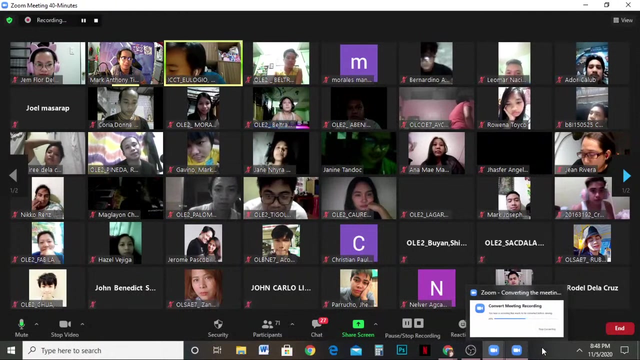 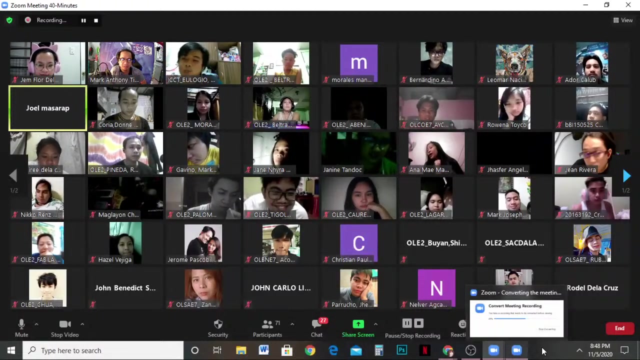 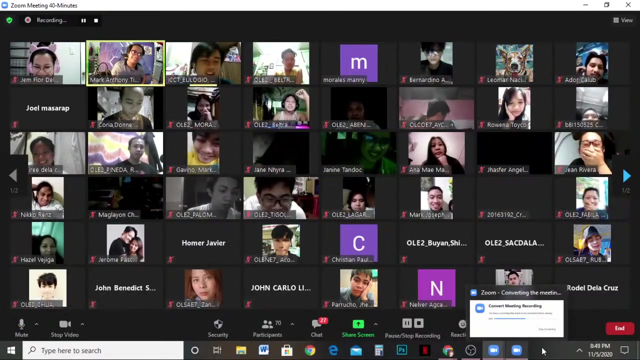 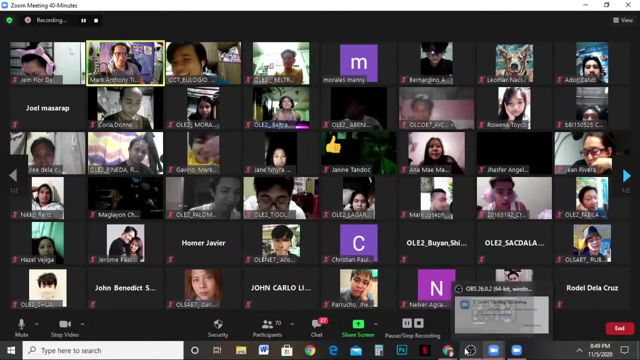 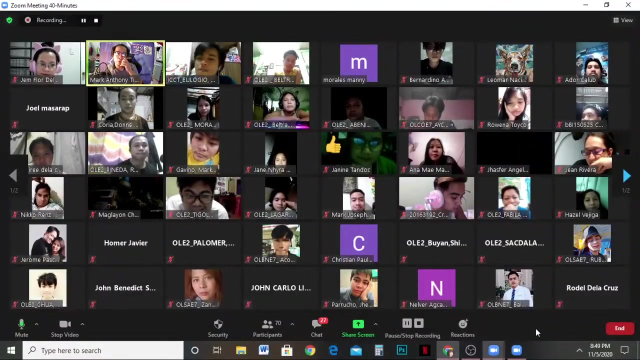 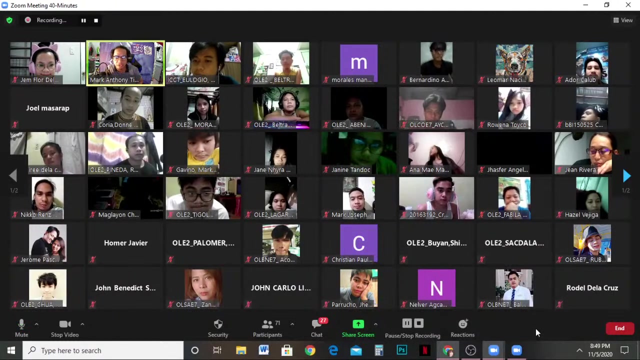 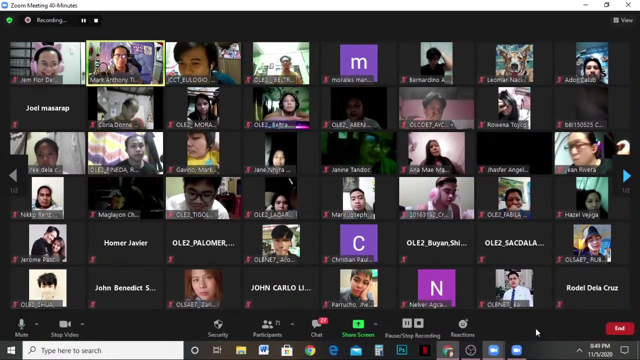 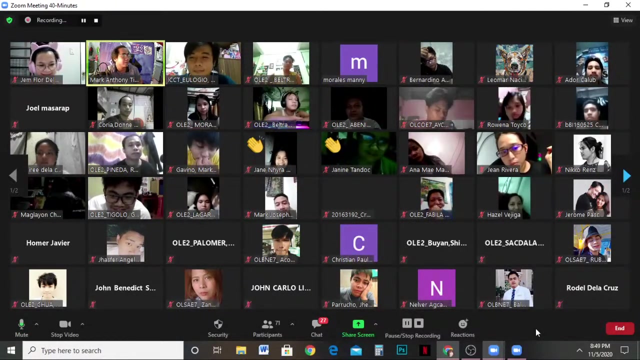 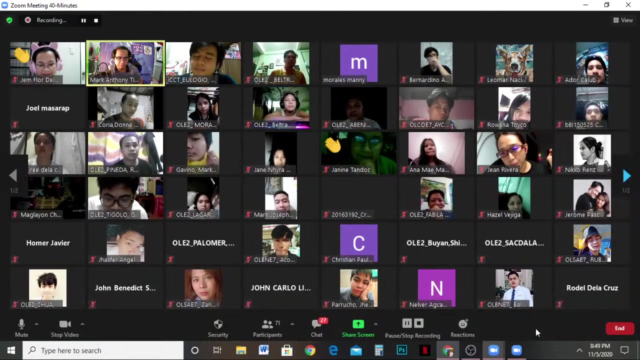 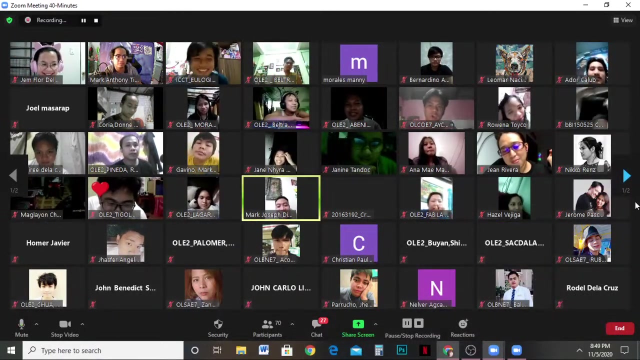 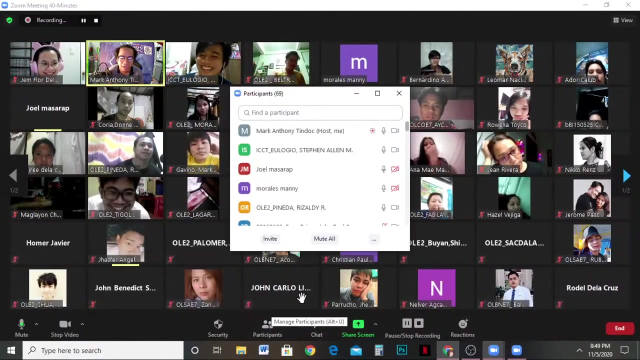 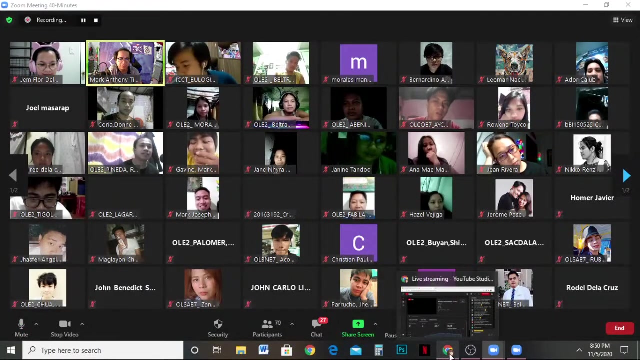 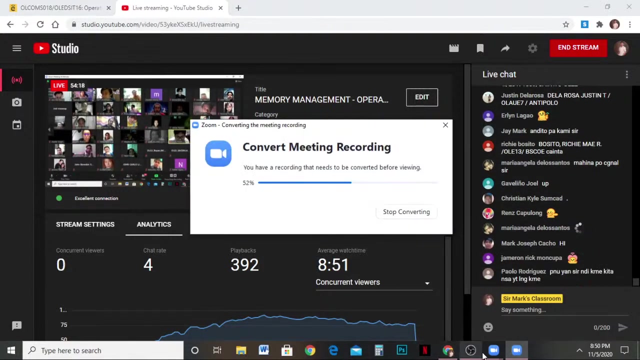 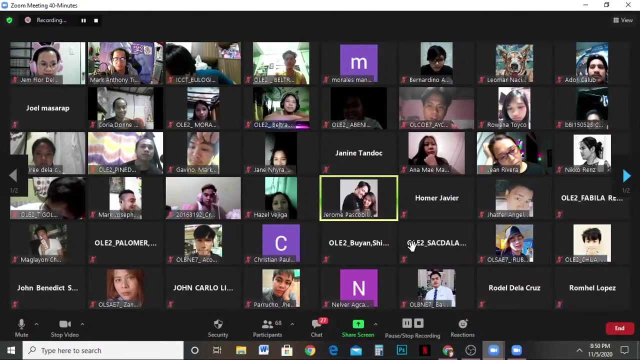 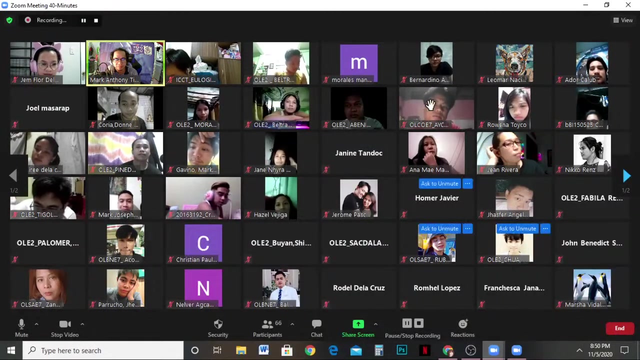 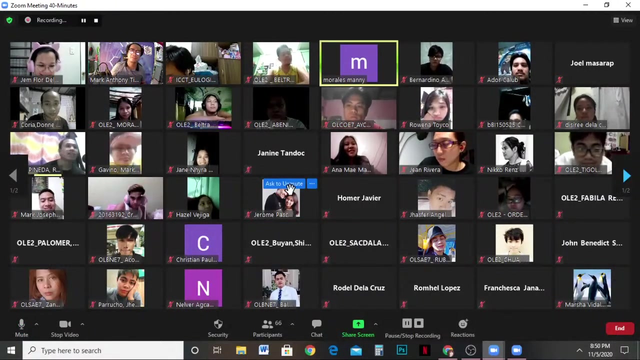 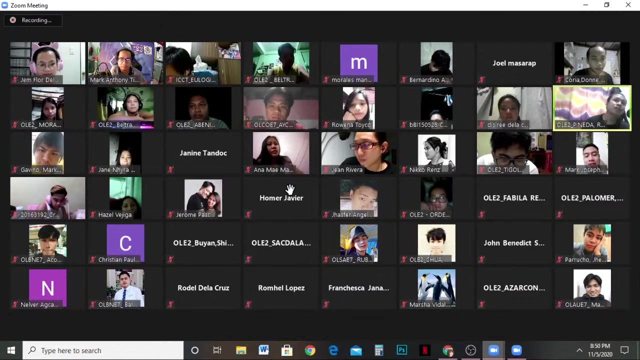 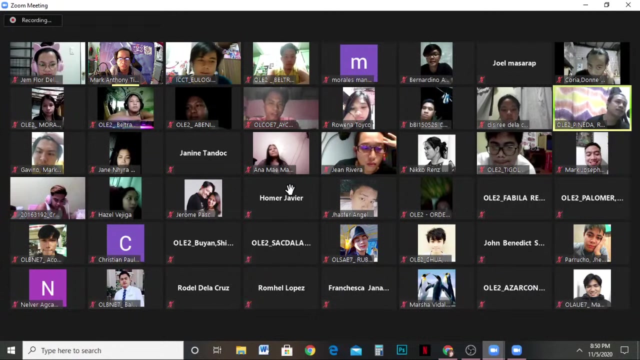 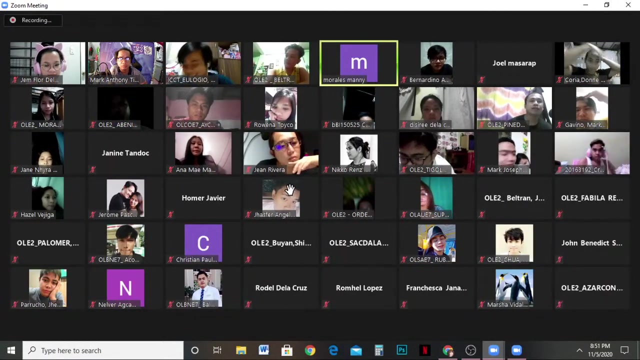 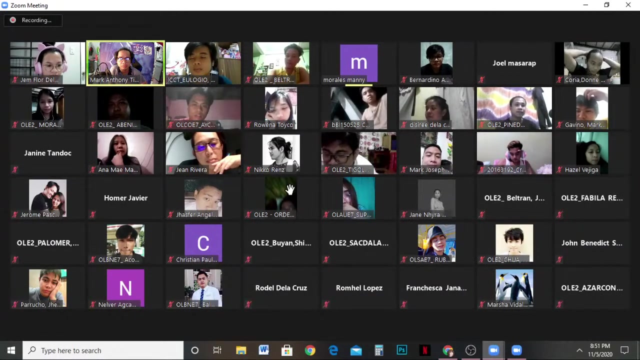 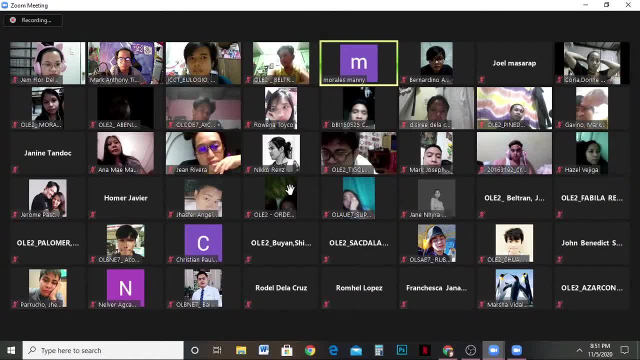 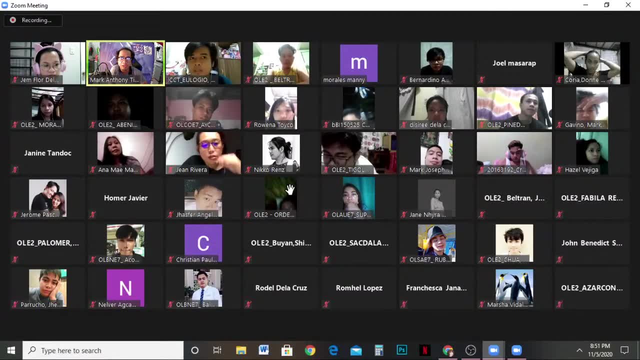 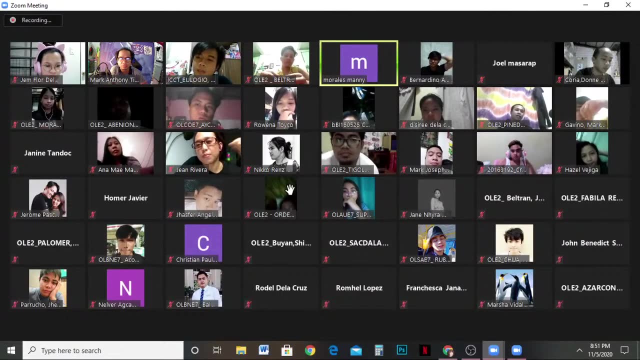 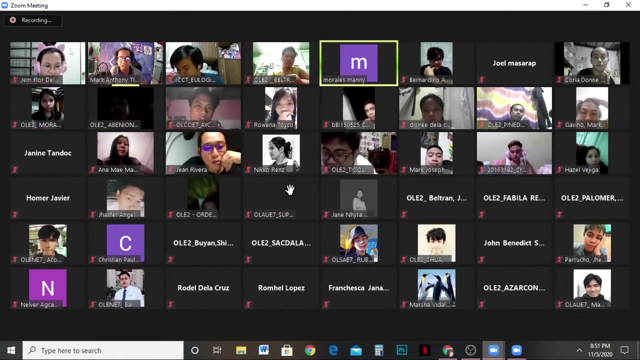 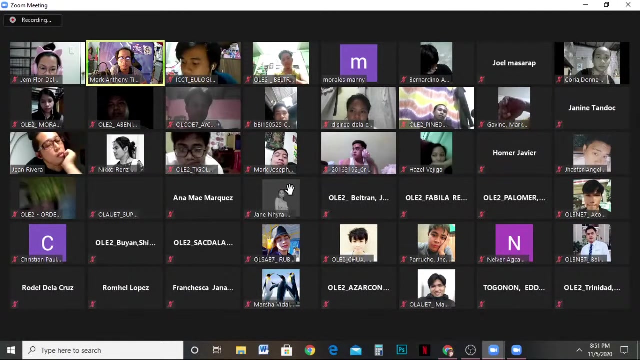 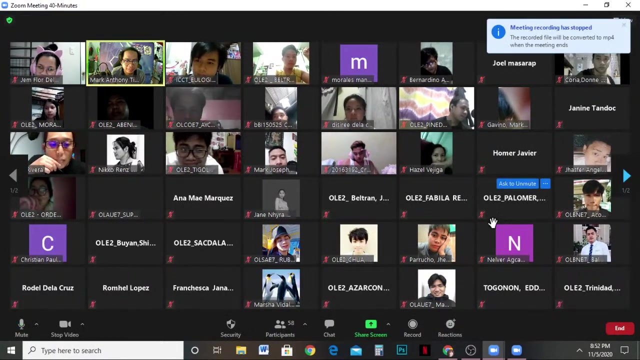 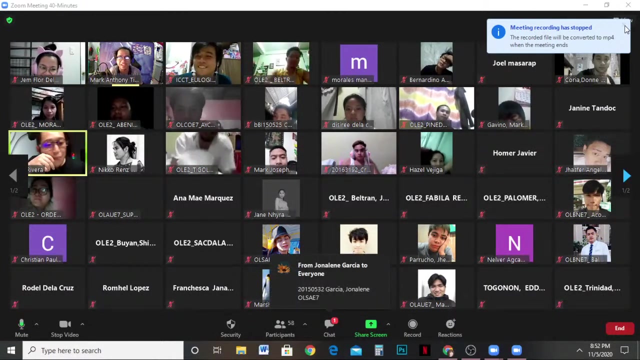 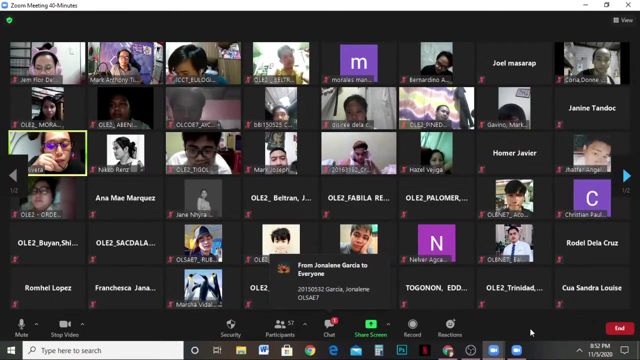 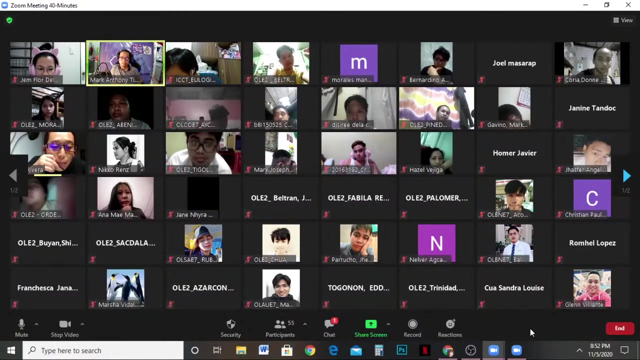 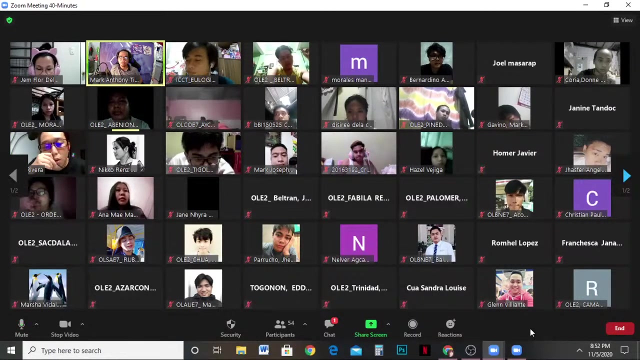 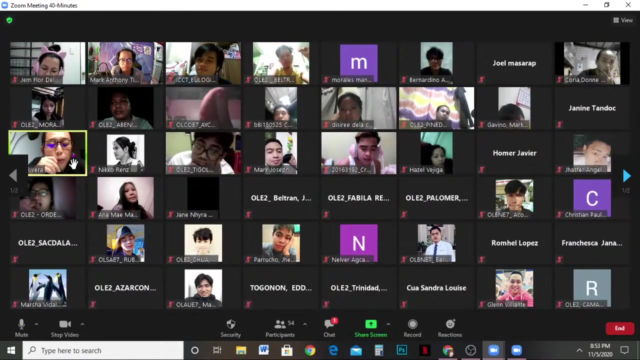 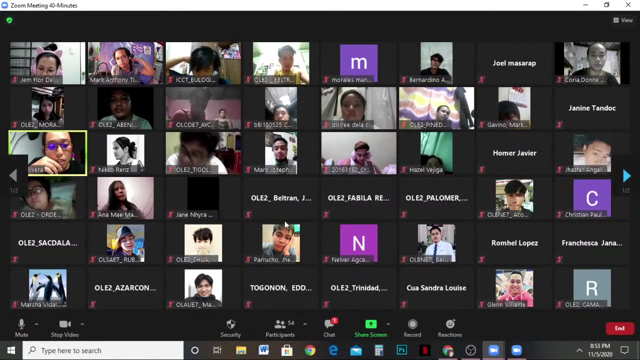 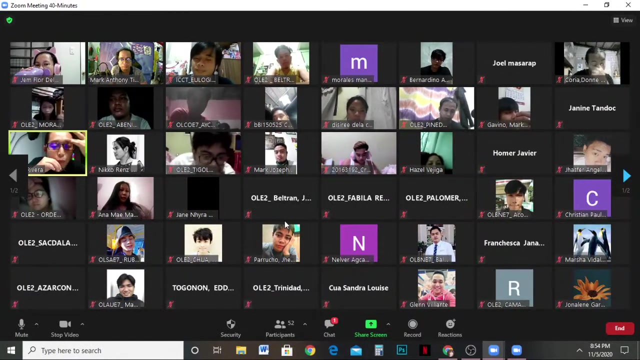 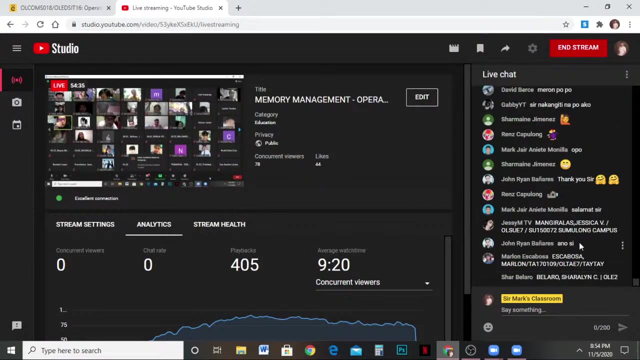 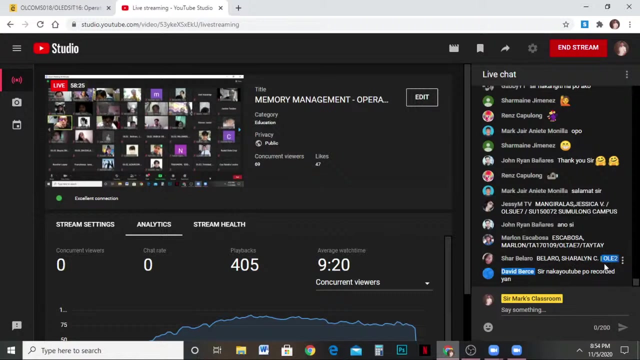 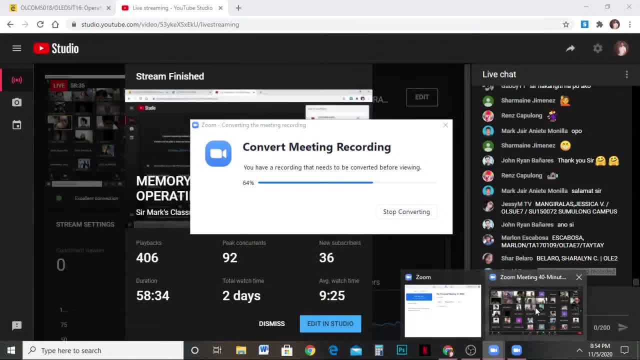 Hello sir. Yes sir, I love what Gene said about the company.